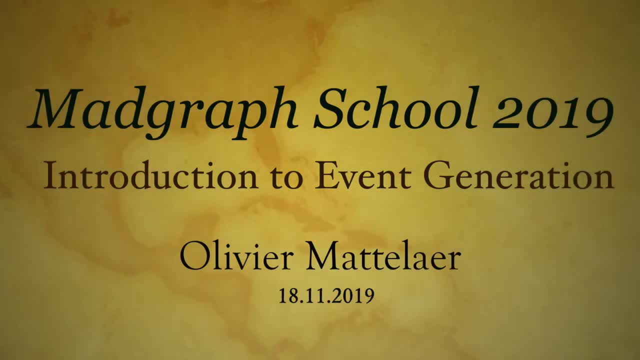 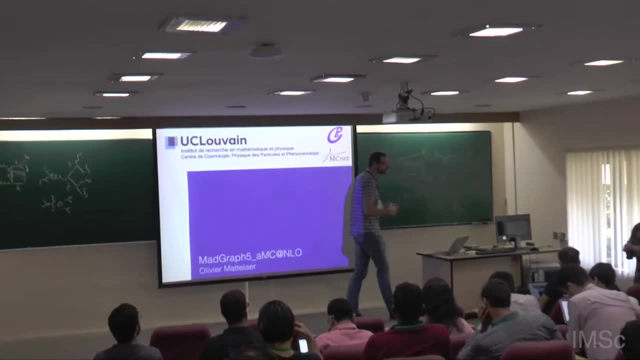 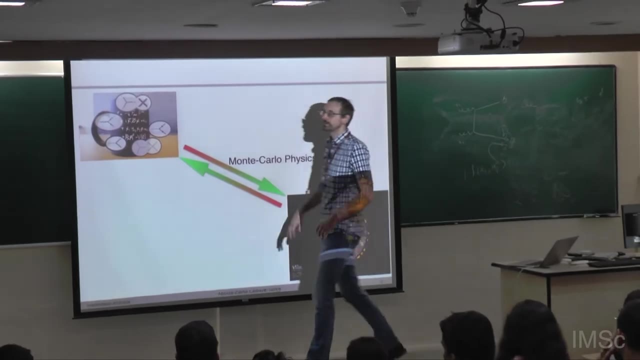 So I'm going to continue basically the same lectures that Benjamin just gave you. so the same idea, and to remind. the idea is basically to close the bridge between the theory part, when you have those marks, those theories, those Lagrangian, where you have all those. 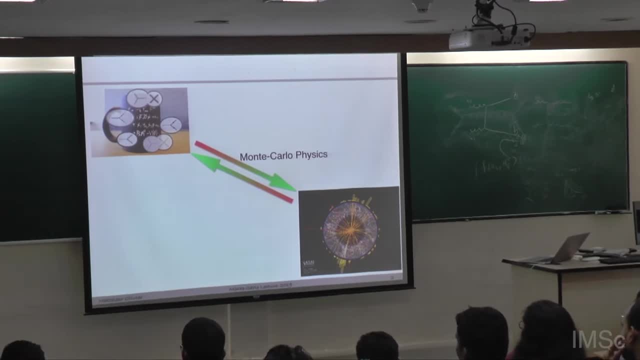 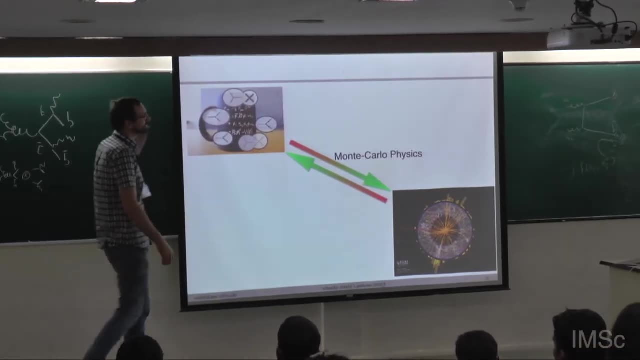 theoretical ideas, all those different ways to approach the problem and, of course, what is key, important for me is all those famous diagrams, so all those famous rules and to bring that to basically what is observed in experiments. so a lot of collisions, a lot. 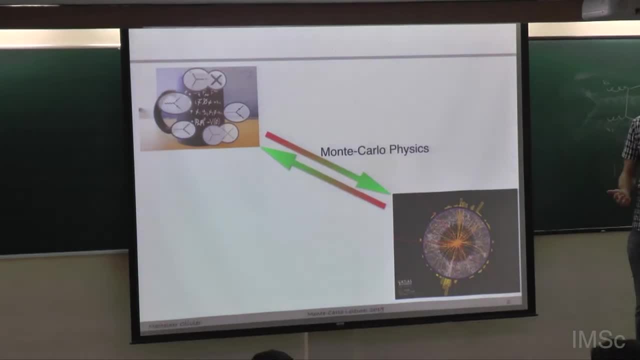 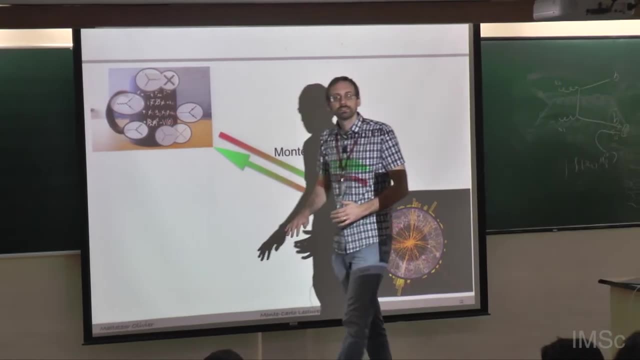 of histograms and you want to see how much they match to each other. And in all fields, especially in MadGraph, I think it's quite important with the arrow here going in both directions. so from theory, I want to be able to explain data, but I want 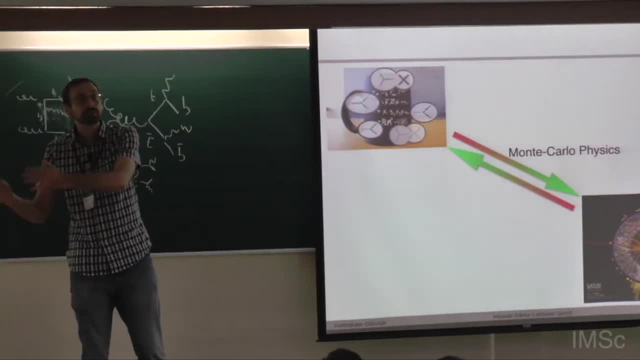 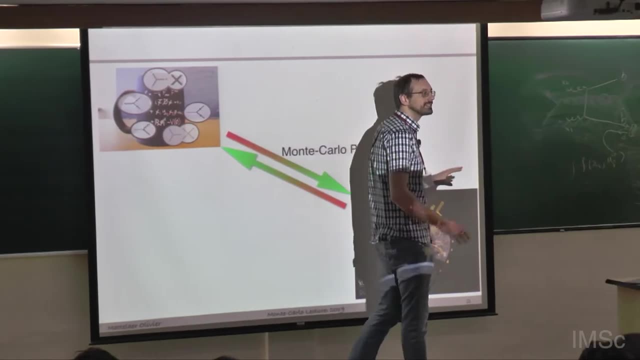 to also try to help from the data to be able to explain what is the theory beyond the data. so I really want to be able to go in both directions In practice. MadGraph is very good: from the theory to go to the data and that's actually. 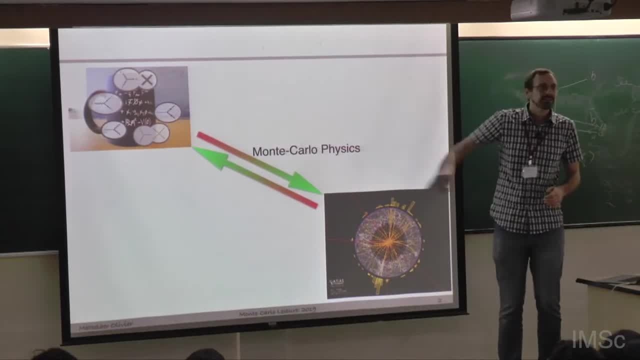 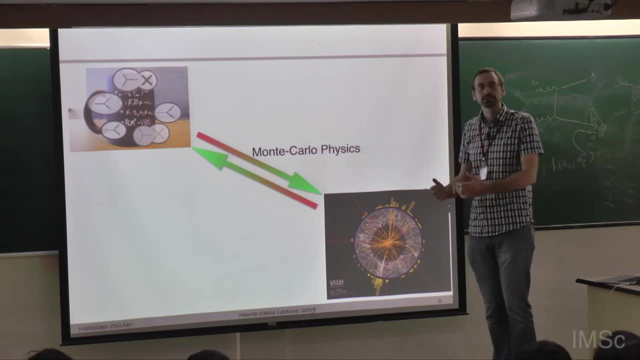 the easy part, I would say, but from the data to go back to the theory is actually much more difficult. We try to help, but of course that's the work of experimentalists to take all those data and try to extract that and that's extremely difficult work which is much more difficult. 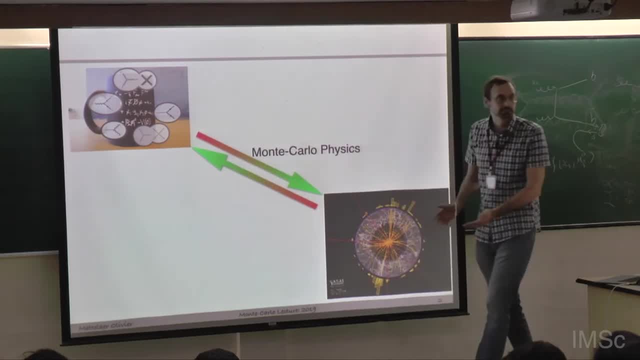 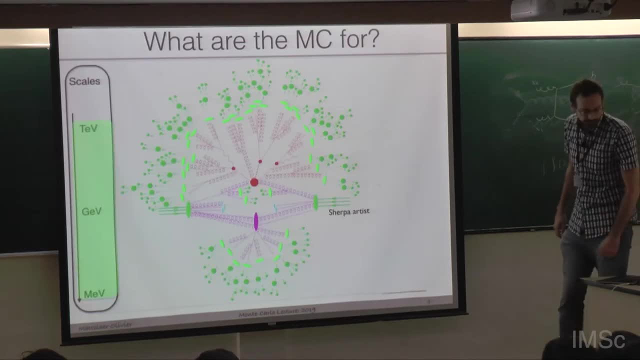 to automate that. you have a theory what would happen in your detector. So, Of course, what MadGraph is doing is simulation of collider events. You have already seen actually this picture, so I'm not going to go back in details again. 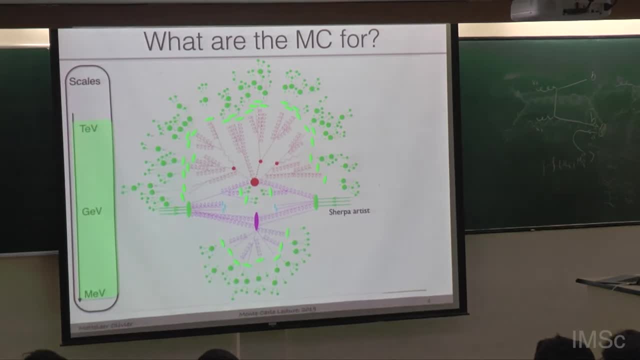 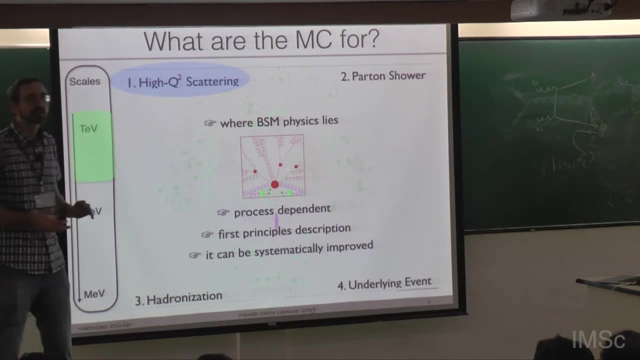 What we are interested in here today, at this moment, is only the curve of it, So only the odd interactions, and that's only what I'm interested in. So tomorrow there will be a lecture by Leif about the pattern, so we see the second step. 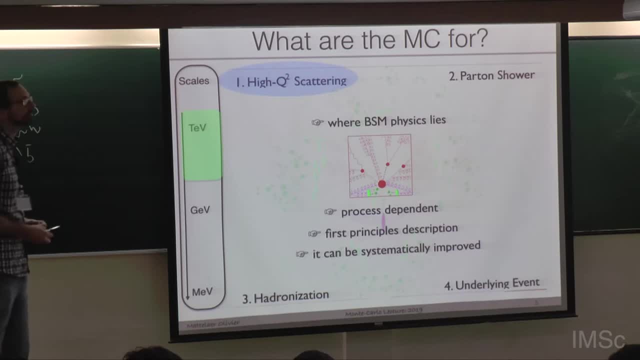 but here today it's really the odd interactions and that's it. So why am I interested in that? Because I'm basically coming from a BSM background. I'm coming from the glorious day before LHC where we can have any kind of idea and say: 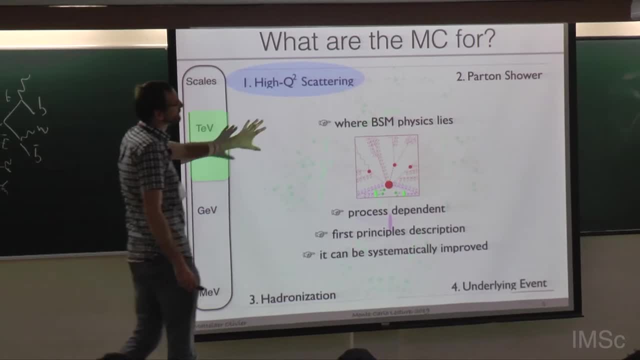 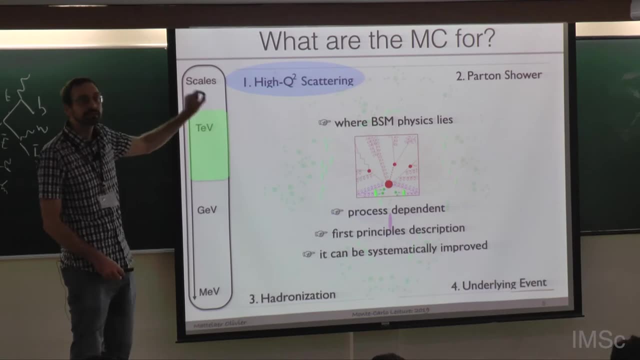 oh, we're going to discover it at LHC and that's really in these odd interactions that you can have BSM. So if you are lucky to find one day BSM, that would be here that something will change your descriptions. This is completely process-dependent. 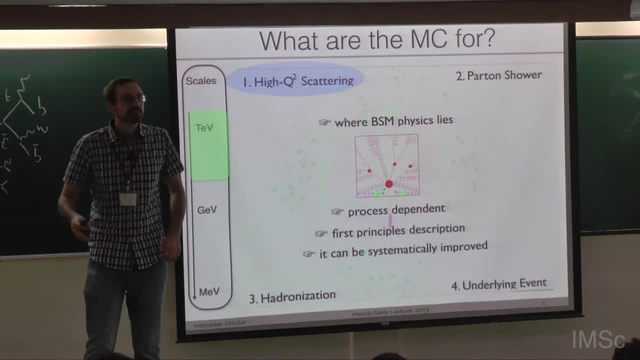 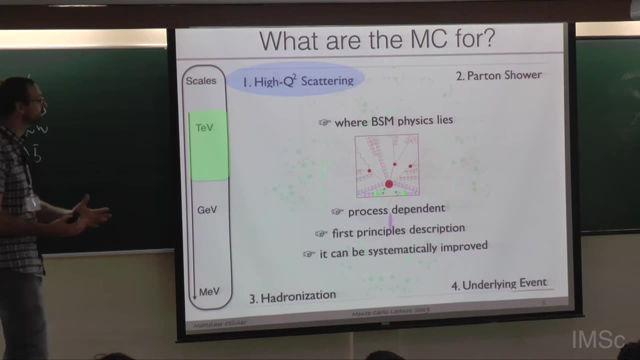 That means for each process we need to do different computations and that's what you do naturally every day. You say, oh, I'm going to do study, tdbar, zx or whatever. You specify your process and that's exactly specifying what's happened at the high energy. 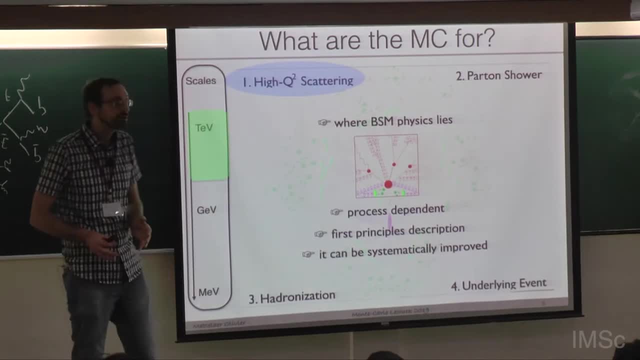 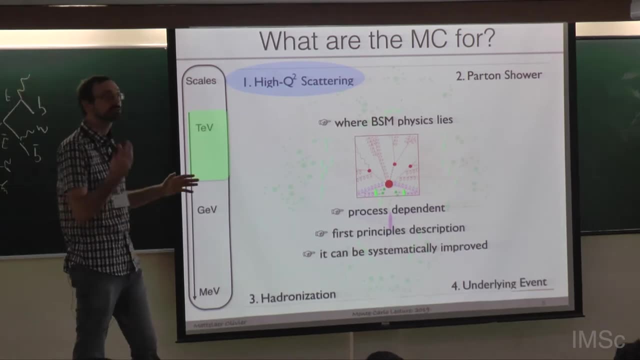 And what is cool here is that we know exactly what we are doing. We know the theory, We know it's a perturbative theory, so we know that we cut In these lectures. I'm basically going to cut at learning order. 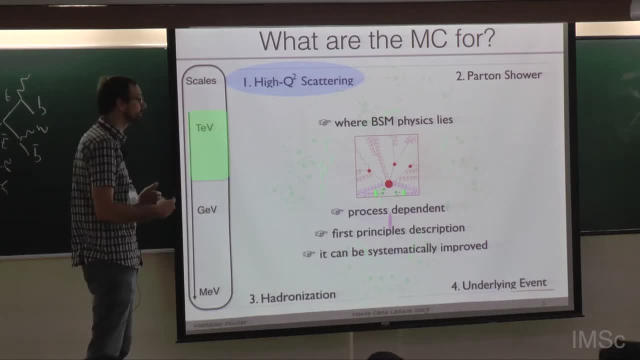 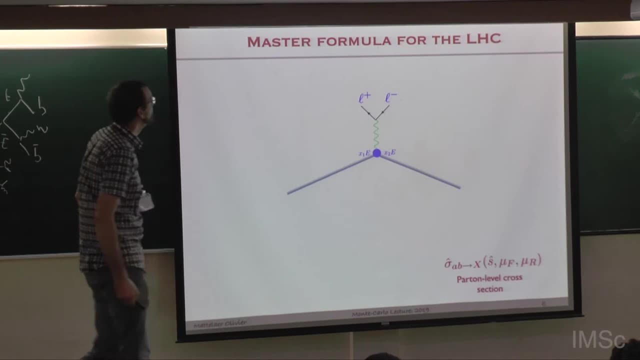 We're coming back to that in one second, but it can be improved So we can go to next learning order, next to next, and so on. So we have everything here quite under control. So let's put the most important formula for today and probably for this whole week actually. 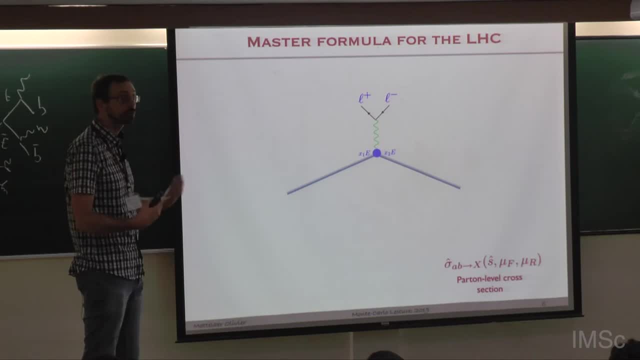 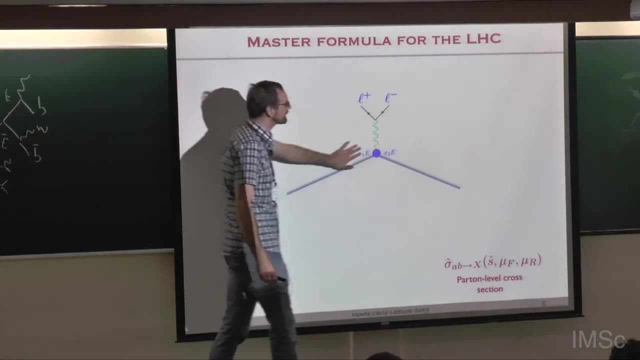 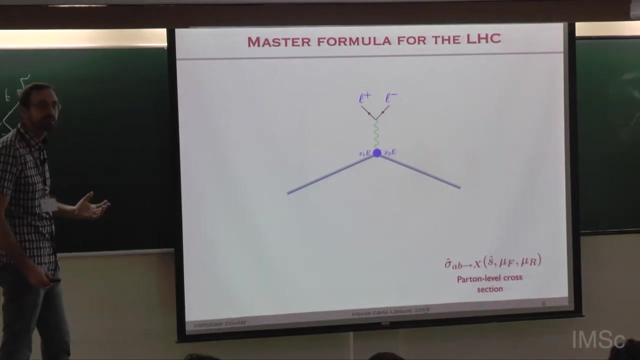 And that's what happens. what is the formula related to all new computations for a simple collision satellite? So in this case I have two protons, actually two quarks, here colliding, going it's a, so that's going to a z of photons and then that's decaying: l plus l minus. 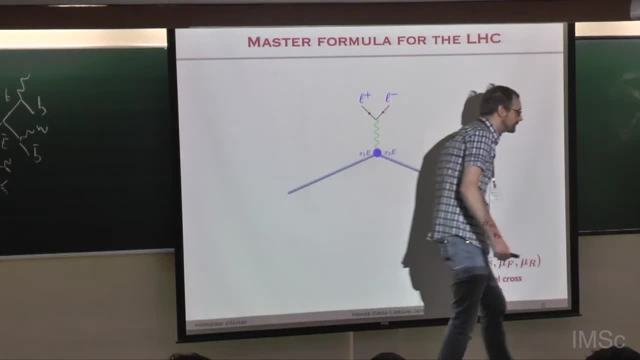 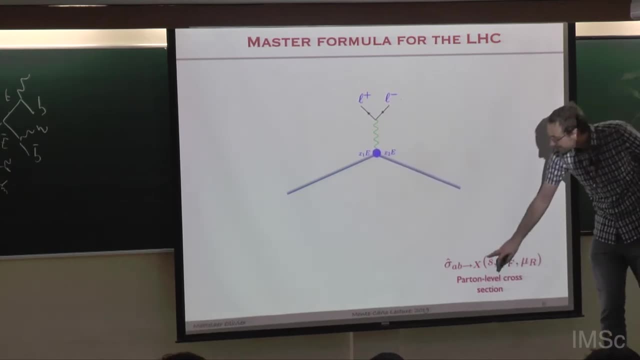 And the cross-sections can be computed. Sorry, At this stage I don't specify where I compute it. Is it learning order, Is it next learning order, And so on. That's not really important. There's, of course, three parameters. 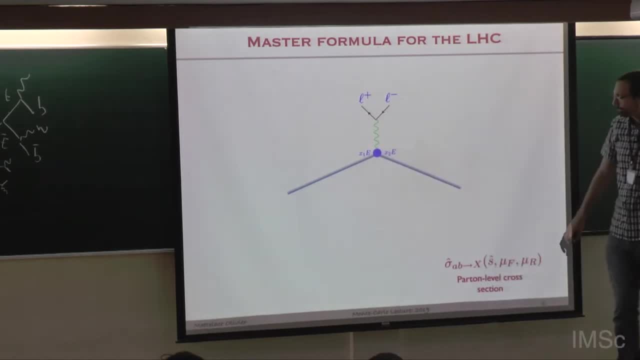 First the energy of the collisions. that's the most important parameter. and then I have two scales: the factorization scales and the chronolization scale. I'm coming back to that in one second. Of course, in LHC I don't collide quarks, I collide protons. 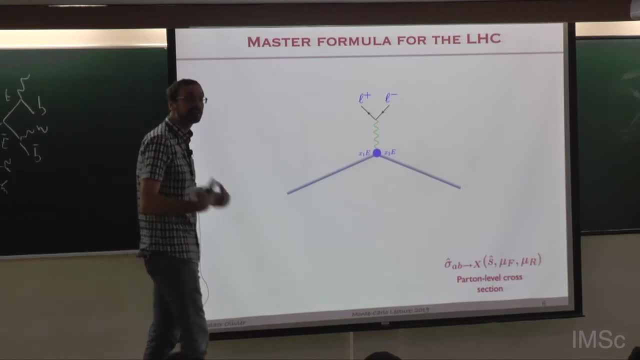 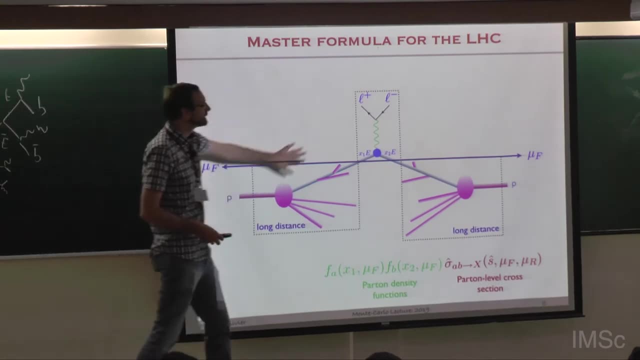 So there's a lot of particles that could have collided and there are a lot of radiations coming with those particles. So that's what the factorization scale is: it's a separation between the hard interactions and all those radiations which is associated to my quark and my proton. 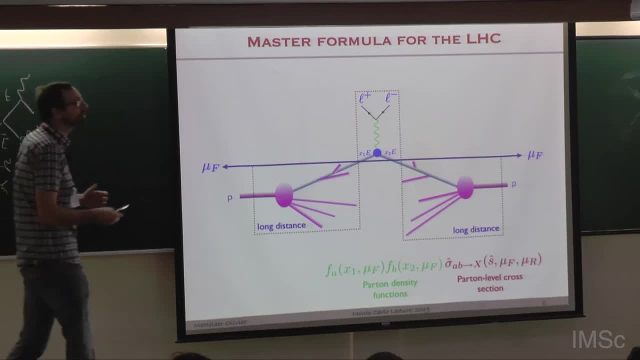 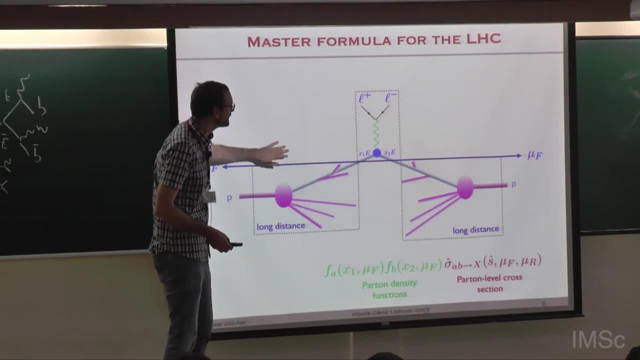 So all those radiations will be included in my PDF, which can be naively said as what is the probability to find a given pattern at a given energy, assuming that all very soft emissions are re-summed inside my PDF. So that's what the PDF is. 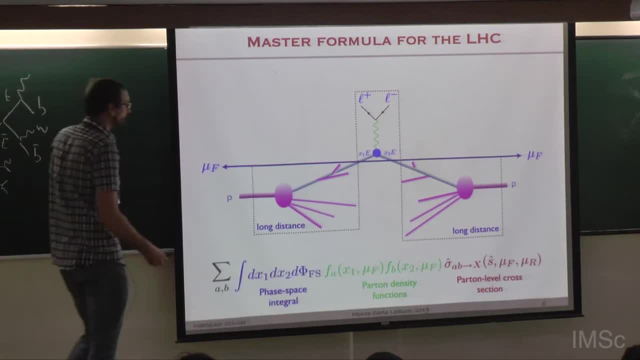 Then of course, I need to compute. Okay, So I need to integrate over all the final state phase, space and also what is the energy of my initial particle X1 and X2.. So that's my huge formula for today. 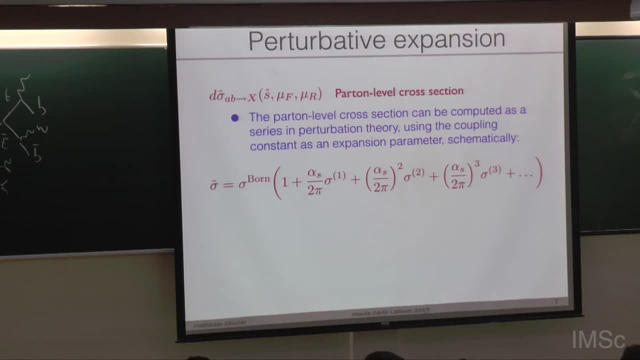 If you have any questions, don't hesitate to stop me at any time. we're quite cool here, so don't hesitate. If something is not clear, just ask. So, as I said, the cross-sections- I didn't define it exactly yet, but we can do a perturbative. 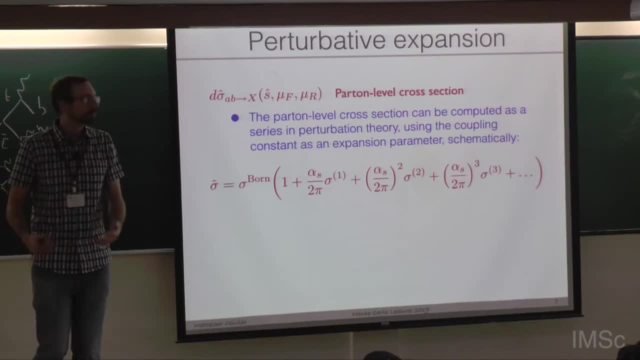 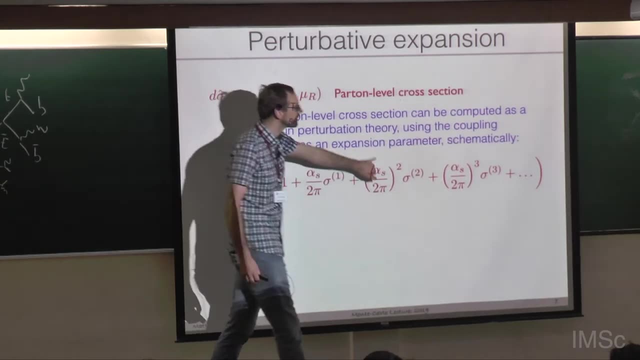 expansion. Basically we do a perturbative expansion in alpha-S in the strong coupling, So we have multiple terms. so first the lowest order in alpha-S and then we have the first order correction, second order correction. That's basically a Taylor expansion to any order here. 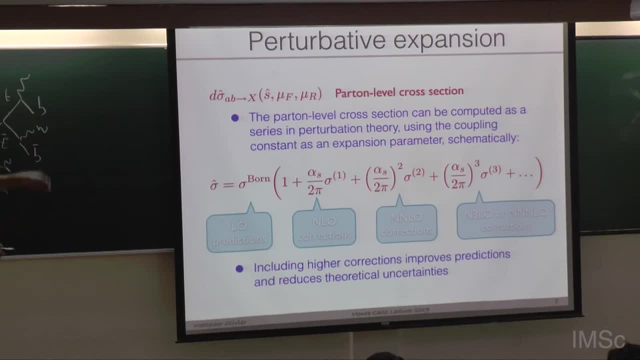 So first order is called leading order, then NLO and then NLO and so on, And, as I said, today we are going to focus only on leading order. So the scale alpha, mu-r and mu-f are actually re-summed. 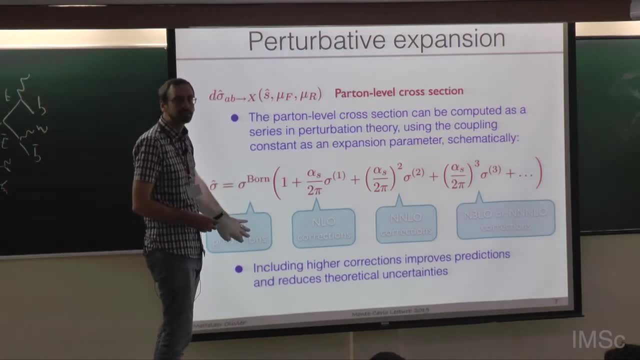 Okay, Okay. So it's really important if you do only leading order. In principle, if you do these full computations here, it should not matter which scales you use. You can put any value. your total cross-sections will always be the same. 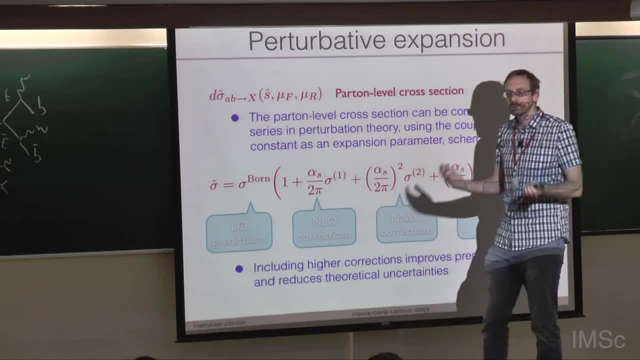 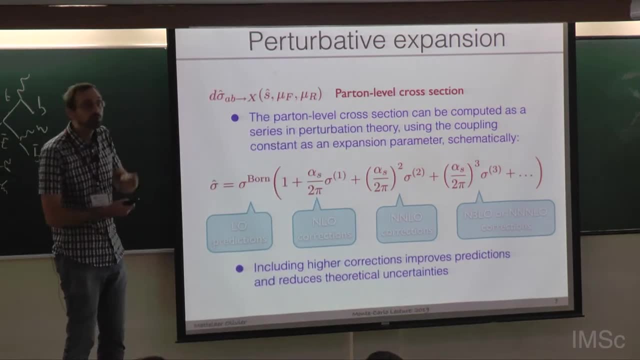 So those are scales which is called unphysical. They should not enter your computation. they should not matter which value you take. In practice you will see that at leading order you have huge dependency in those scales. So you can have up to 50% uncertainty in your full cross-sections simply by changing the 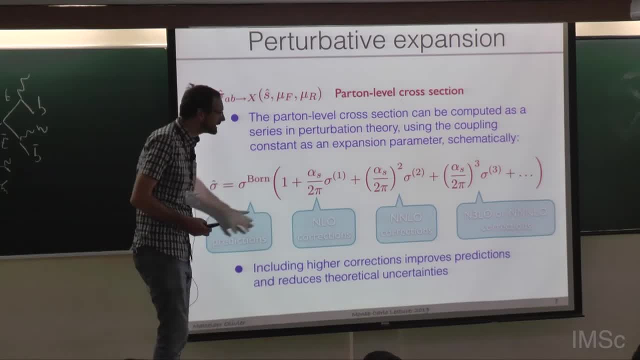 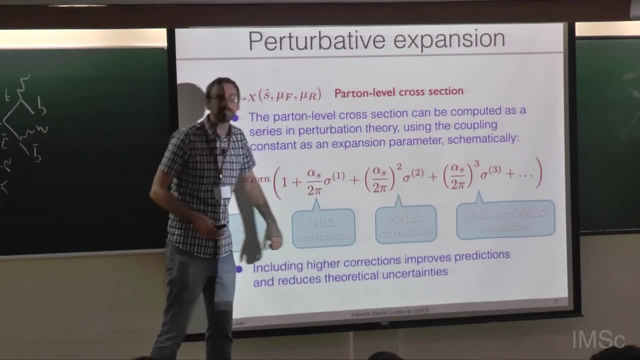 scale by a factor of two. So that is really huge issue at leading order. You have huge dependency in those scales And that's why it motivates us to typically go to next leading order, where we reduce this dependency already quite a lot. 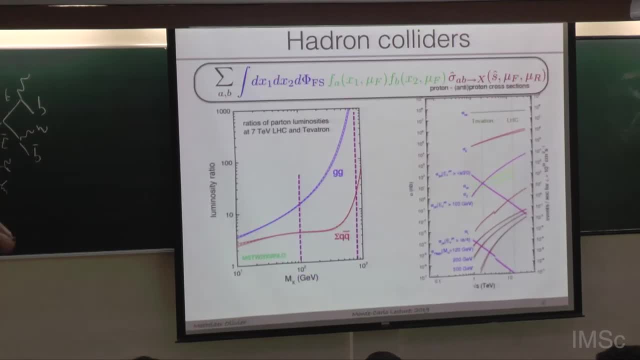 That's the main motivations for NLO. Let's go back to these full expressions here. We already discussed this first term and say that we are going to focus on leading order. I want to stress the importance of the PDF. Okay, So this is a quite old table now. 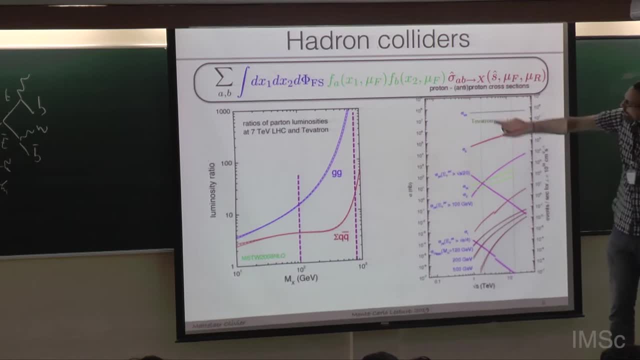 So basically that's different energy, squares of energy where this first line here was corresponding to the energy of Tevatron in the old days and this line is the energy of LHC. You see different process and some process doesn't scale that much and some process. 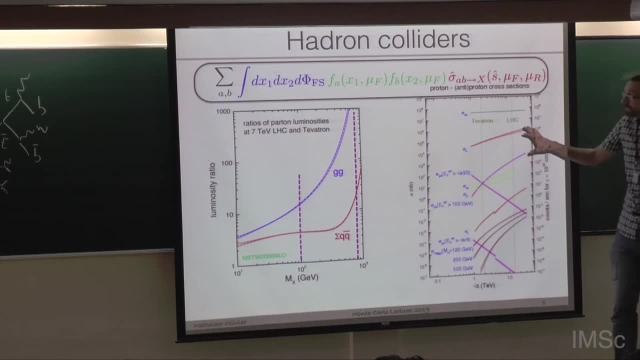 like, for example, this one is the top scale a lot And that's really the reason for that is not with the matrix element itself, but it's really the PDF And that's what you can observe here. This is the ratio of the PDF between 7-TV, LHC and Tevatron. 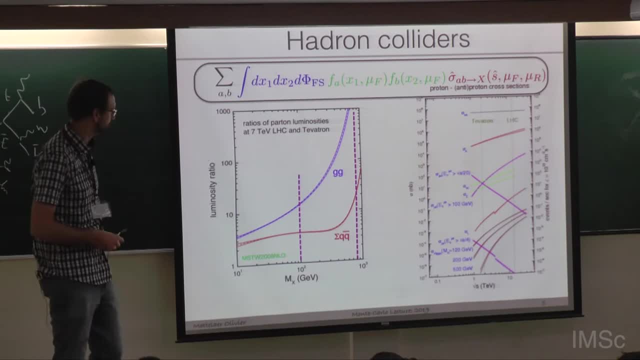 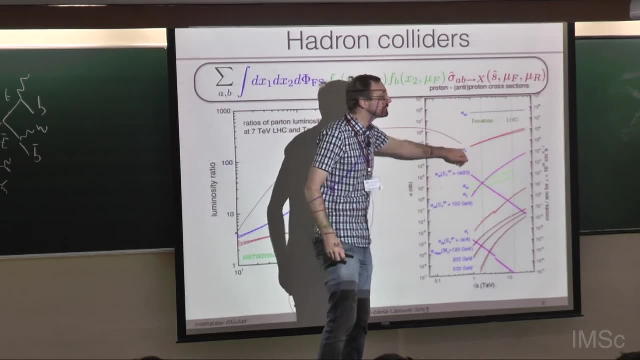 So it's also a fact. of course, Tevatron was PP, bar not PP. And now, if you look, for example, to this process, so that's B productions, Those are B, so they are very massless particles. 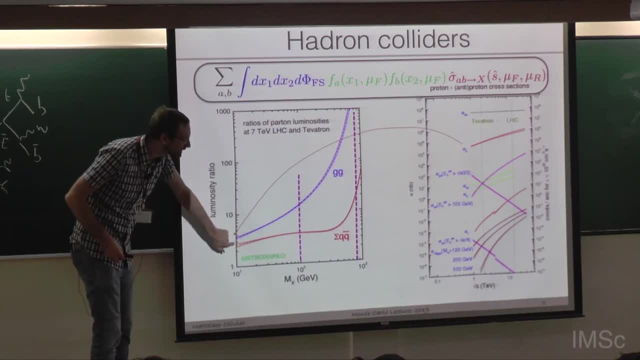 So the energy is very, very small. So you can see that in this regime the ratio of PDF is very small and that's why that doesn't grow that much. If you go to the next slide, The next one I want to focus is the Z productions. 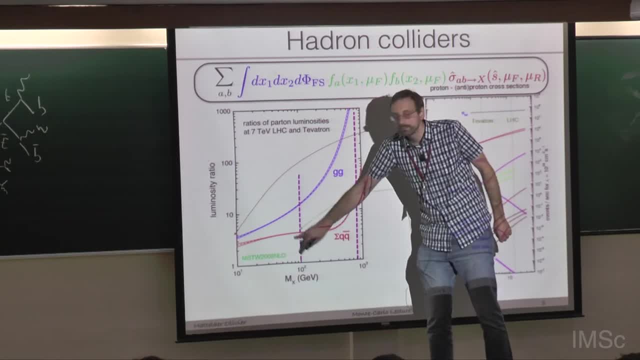 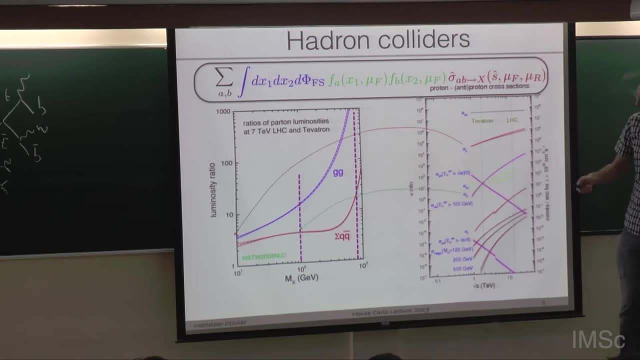 In this case the energy is bigger. but you see, still, since you have QQ bar to produce the Z, it doesn't increase your cross-sections that much. it's relatively flat. Now, if you go to the top, the top is dominated by gluon-gluon productions, and that's why 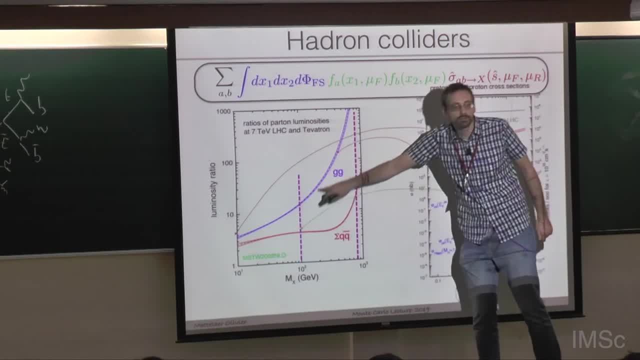 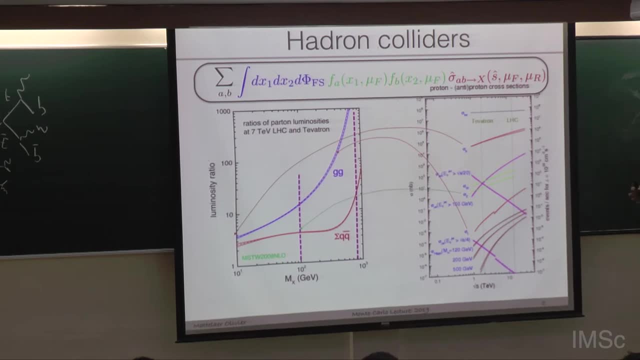 you have a huge productions increase here which correspond to this gluon-gluon ratio between the two. So that is typically what dominates your physics. actually, in the collider It's really related to the energy. So you can see that. 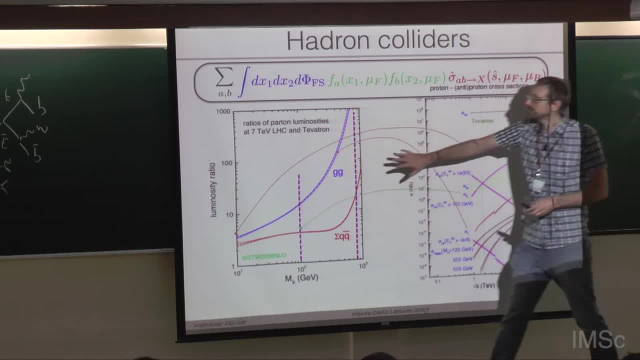 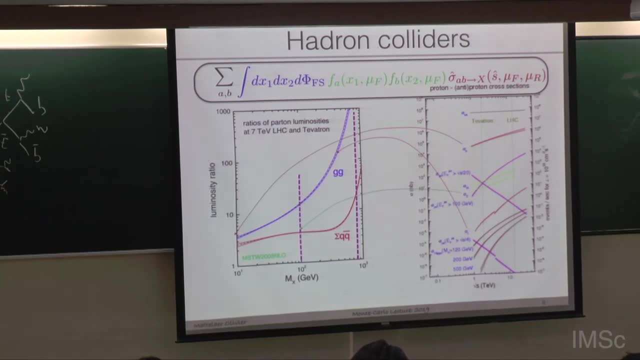 It's really related to your PDF And that's why these kind of plots are crucial for those days where we are looking: should we go to 27 TV or LED TV? which kind of process will be available? all those parts will be. 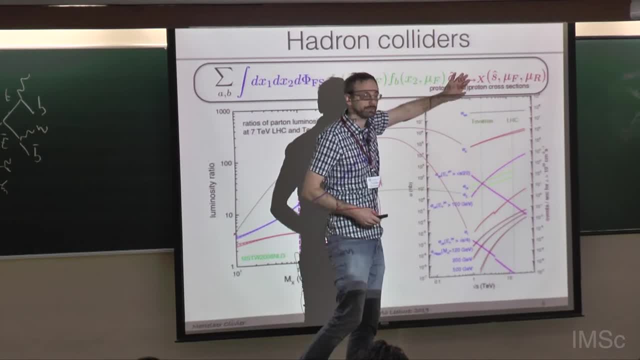 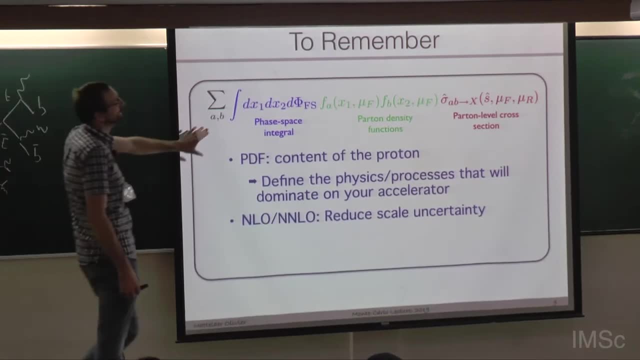 actually dominated by the PDF, much more than the matrix element itself. Okay, so what to remember up to now? So that the main part for the physics accessible is actually related to the PDF that we define the physics and process that dominates in your accelerator. 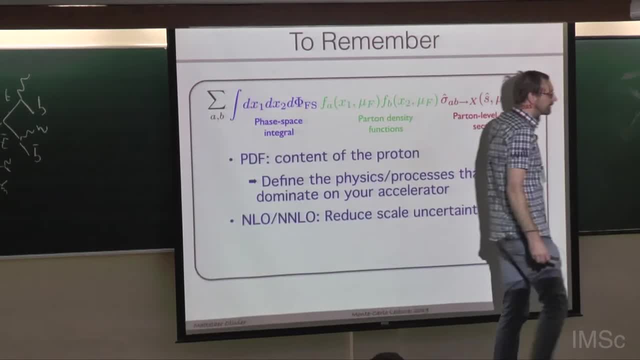 And the second part is, if we want to get rid of the huge dependency in those scales, mu f and mu r, you need to go to higher accuracy, you need to go to NLO or NNLO In a rule of thumb. leaning order is already quite good to predict shapes. 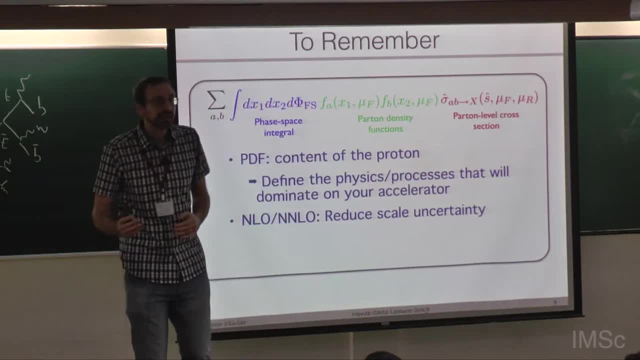 So if you want to look at differential distributions and you don't care about the full normalizations, leaning order is quite accurate. it's quite good to do that. Okay, If you want to get the full normalizations correct, then you need to go to NLO- NLO. 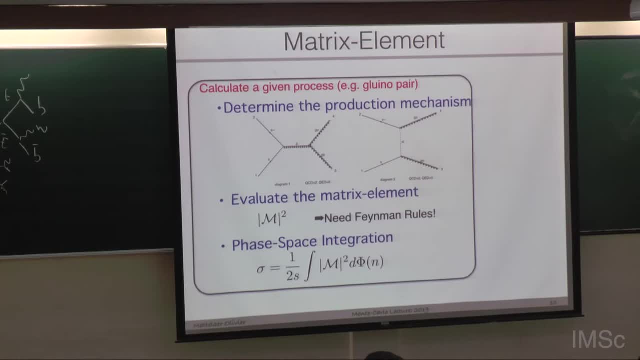 Okay, so now let's move in the program of how to do those computations automatically within MadGraph. And there are basically three main steps. The first step is to determine all the Feynman diagrams. So for that you give me a model, you give me a piece of paper. in principle, I can determine. 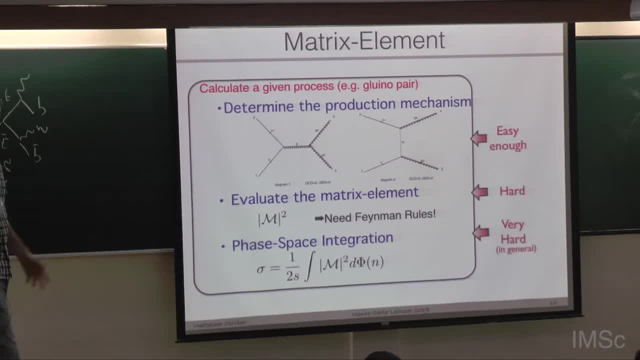 myself all the Feynman diagrams. So that's what I call. this part is easy enough. You give me a pen of paper and everyone in this room will be able to do it Now, for 2-2-2 is trivial enough. 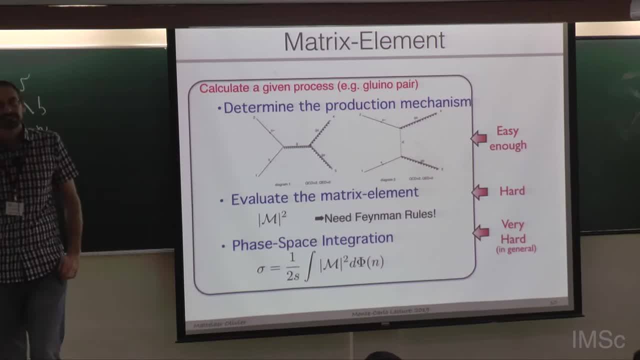 If you ask me to do all the 2-2-3,, 2-2-4,, 2-2-6, I'm pretty sure first I will take a lot of time, obviously, and then I will always forget the one Feynman diagram. so make a. 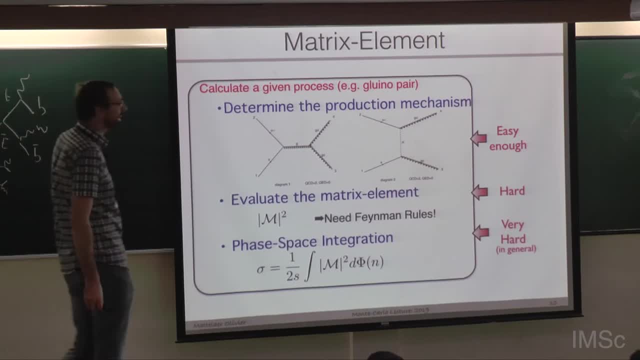 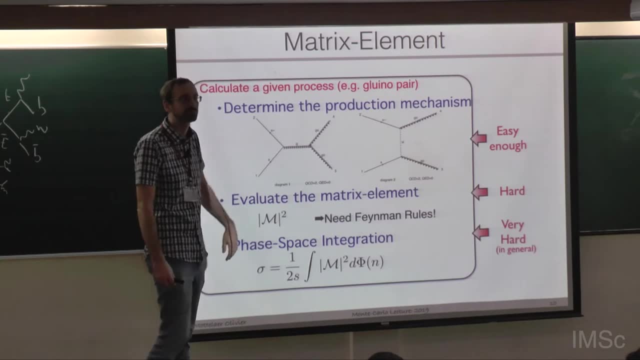 mistake on one or whatever. So it's a boring task, but that's very simple to do. Computer is perfect for that, obviously. So we're not going to discuss how, in MadGraph, we do that. it's just boring details and not. 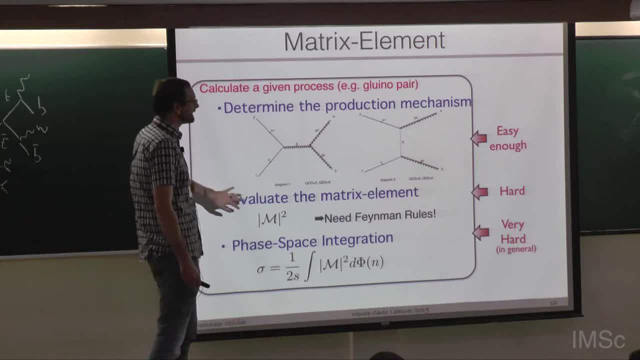 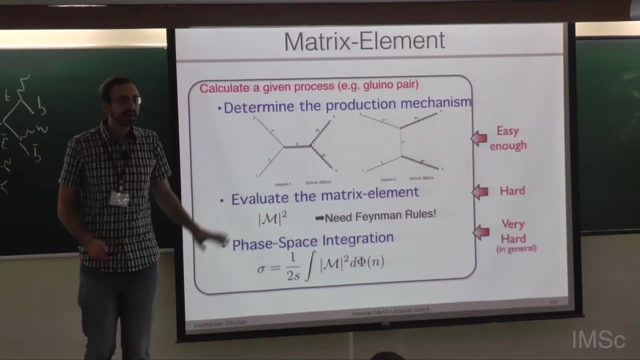 really interesting. The second part is more complicated: How do you evaluate the amplitude square? So that was already covered, actually, by Benj in the previous lectures. I'm going to re-explain it a bit relatively quickly because it was already explained. 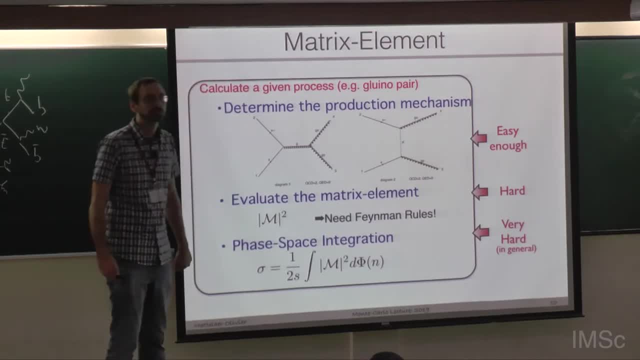 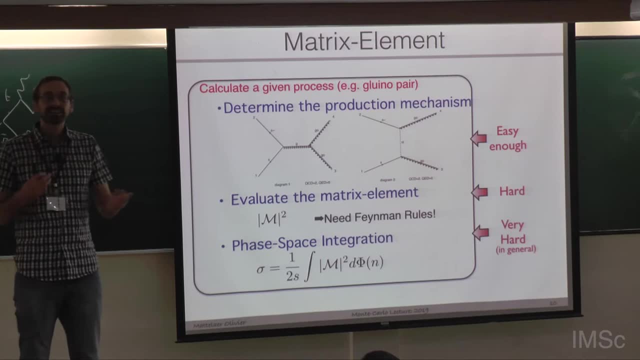 And then actually the most difficult part was the phase-space integrations. That's typically that a lot of people say, okay, yeah, it's phase-space integrations. no, really one cares. They say: you just have to do it. 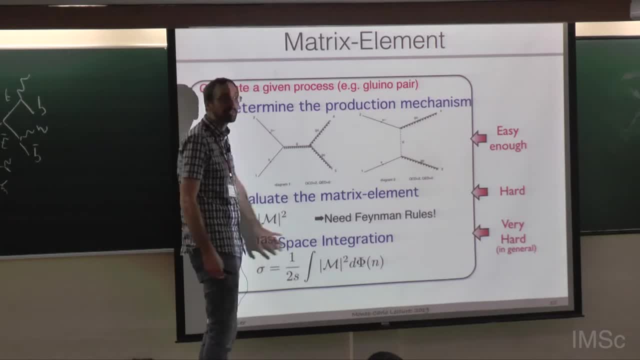 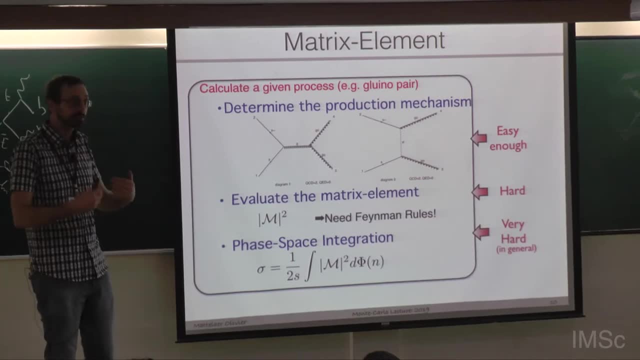 It's actually, from my point of view, the most difficult part. Actually, my full thesis was how to integrate some specific functions, And that's really something which is really difficult: how to design correctly and how to integrate correctly a phase-space integrator. 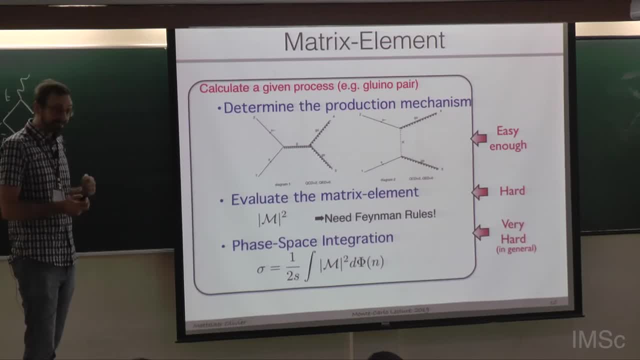 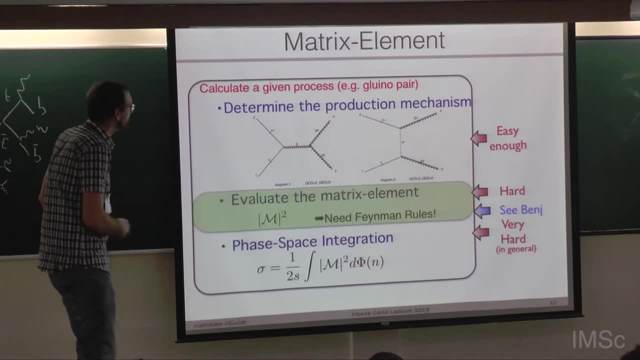 And I think that's something which is important for you to understand- that this is not something trivial and you cannot do anything that you want because otherwise that step is going to fail. So, okay, Let's. Even if you see that already, I'm going to re-explain it a bit. 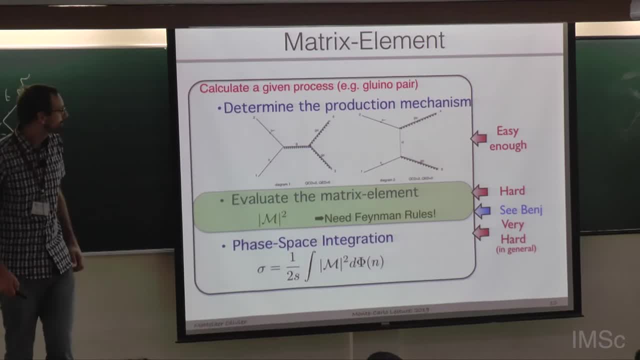 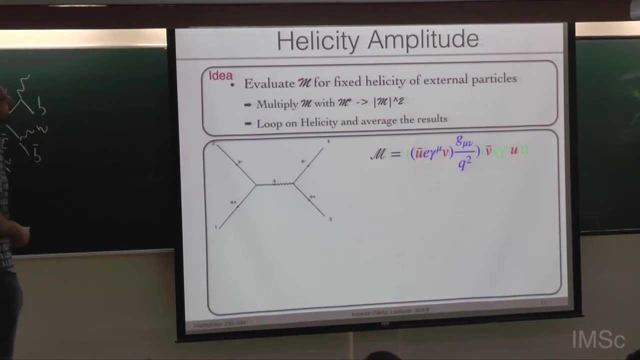 Okay, So already, let's refocus a bit on amplitudes and how to evaluate them. Okay, So, as you have just learned, computing amplitude square is very, very slow because you have a lot of MN diagrams, a lot of interference term and that's computations. it's extremely 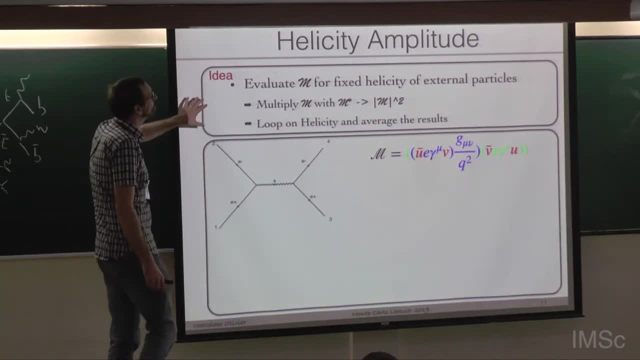 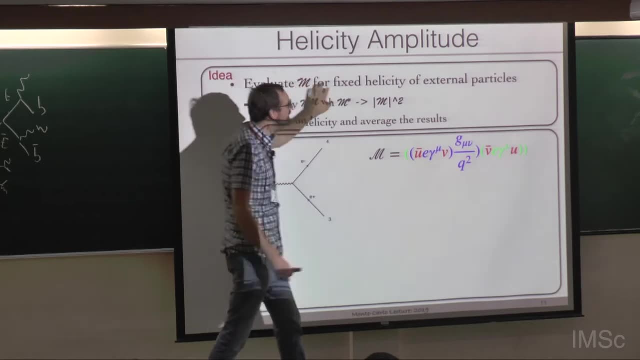 long to do analytically. So the solution was to go to the computing directly the amplitude and not the amplitude square. Okay, And what we do is that we fix the elicity. So we take the elicity, we fix one elicity, then we evaluate the amplitude. 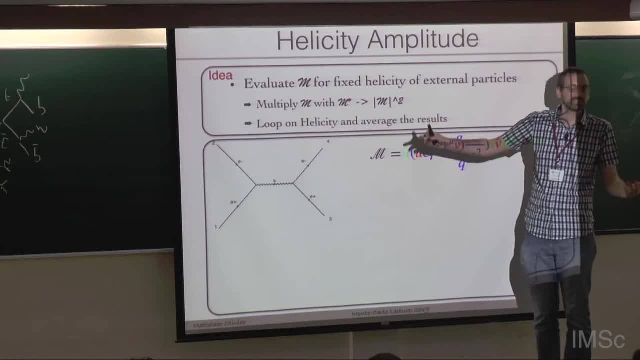 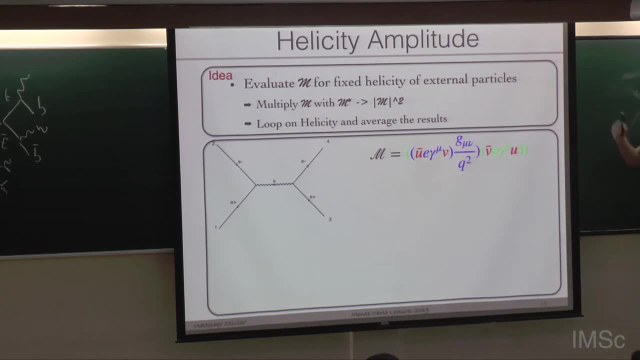 When we have the amplitude, we just take the complex conjugate. That's a trivial operation. So then we have the amplitude square for that given elicity And then we can do a loop. Now we go to the next elicity, redo the same. 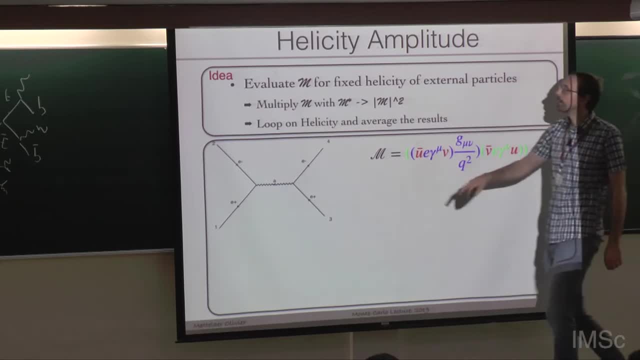 We go to the next elicity, we do the same again, and again, and again. So we just have a huge loop And each amplitude can be expressed like this. So the first part is all those red part which is just elicity vectors. 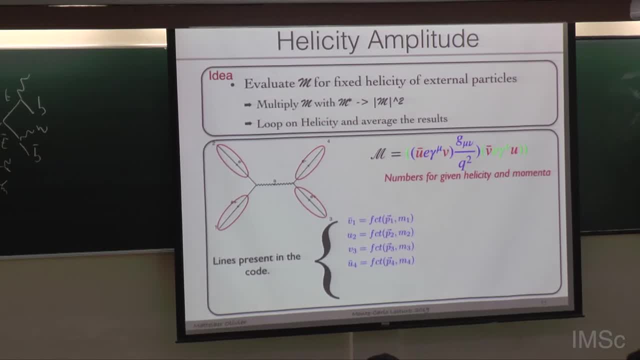 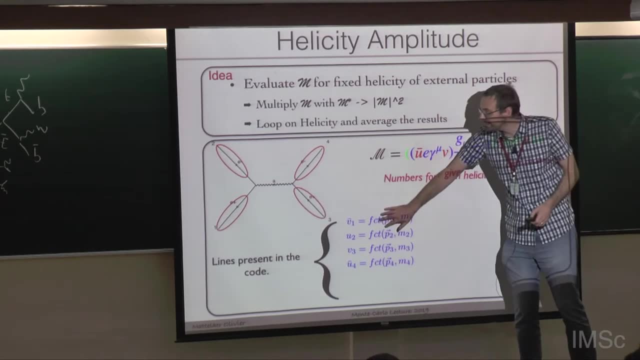 And we know we open your textbook Peskin and Schroeder, we know representations in four dimensions about those functions. So those are the actual line that you will see in MadGraph. Of course it will replace functions by some other crazy names, but there will be really. 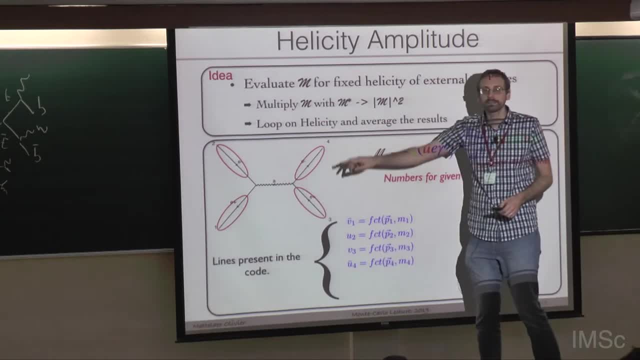 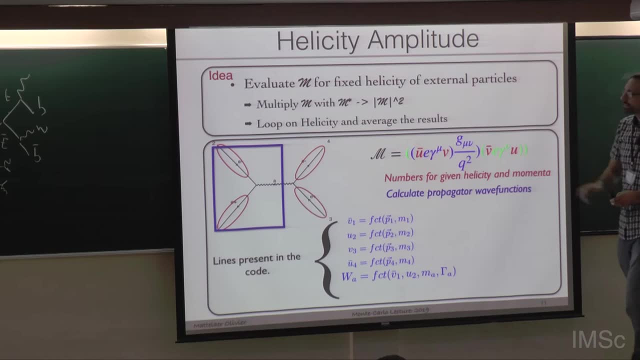 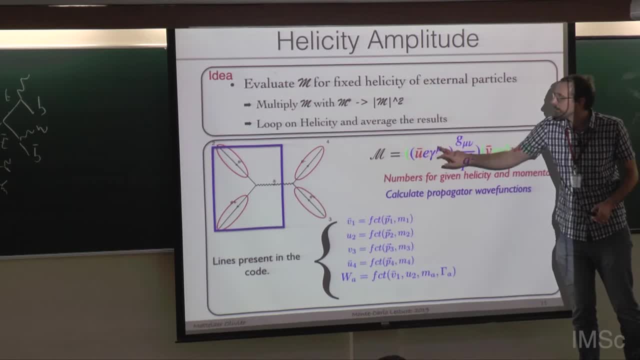 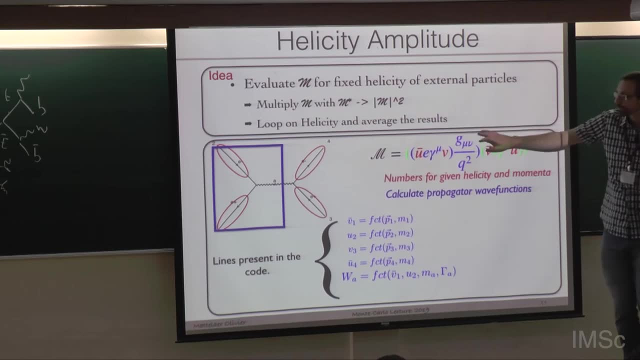 to the photon. So we multiply those two numbers via gamma matrices and then multiply the propagators, And this will give us the propagator, what we call the propagator wave functions, And I'll just show the line in the code. So what is really important here to understand is that in MadGraph we don't have the analytical 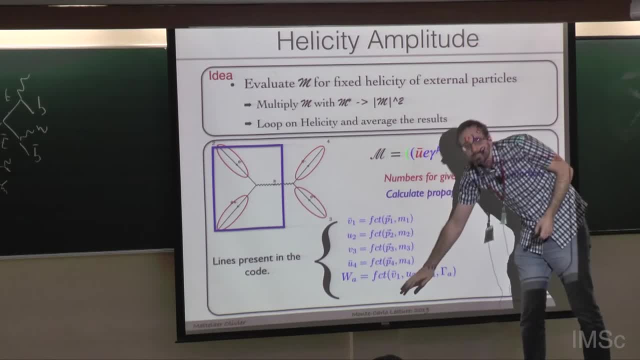 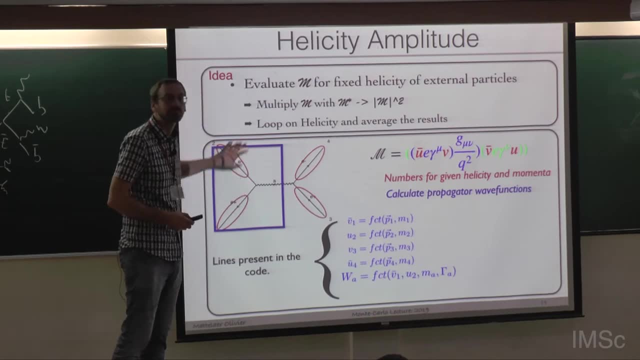 formula in itself. We just have a huge series of lines that describe your Feynman diagrams step by step, And each of those lines corresponds to one propagator or one final state particles in your Feynman diagrams. And then finally, the last line, of course. 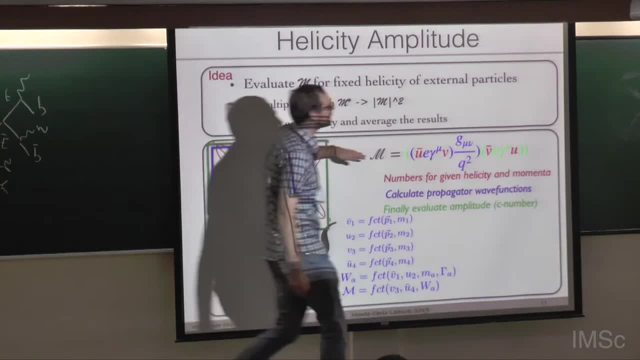 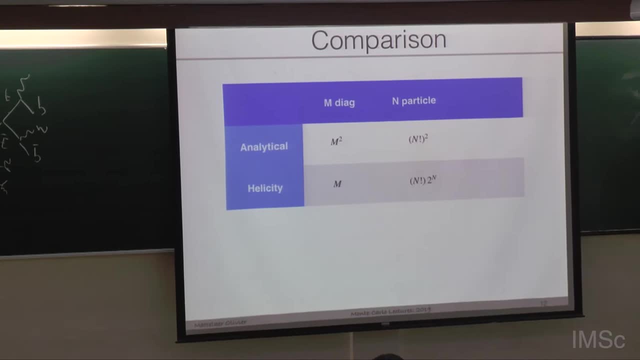 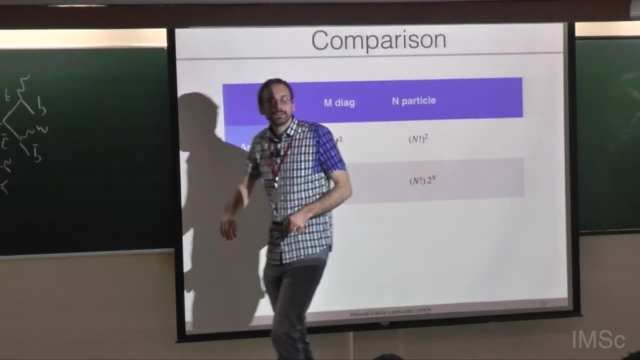 is the full amplitude that we evaluate. It corresponds to the full stuff, this full green stuff here. So you already also seen this slide, actually, So saying what is the speed of the computations. So if you have n Feynman diagrams or n particles, 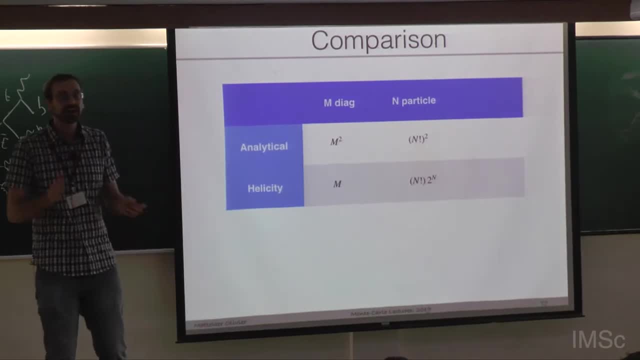 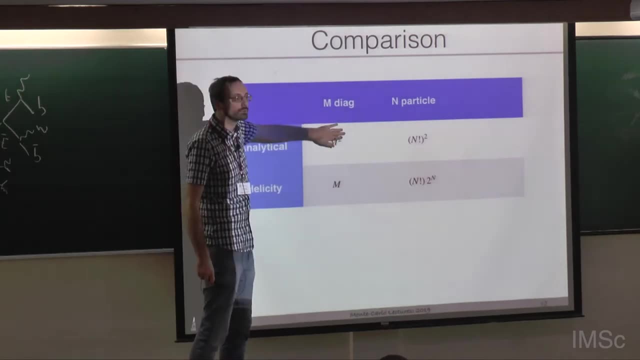 you assume that if you have n particles, you roughly have n factorial Feynman diagrams, which is the correct order of magnitude, at least. So that's why for the nickel computations you have m squared, because you have all those interference terms and therefore n factorial squared in terms. 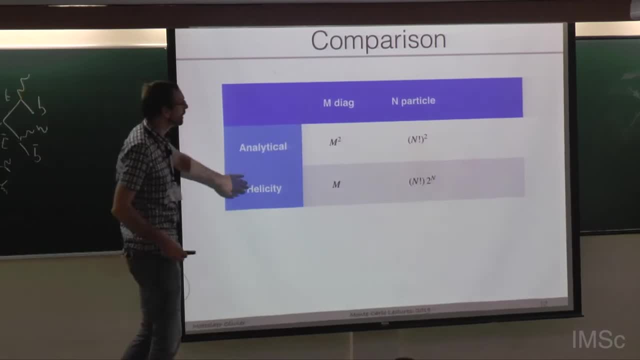 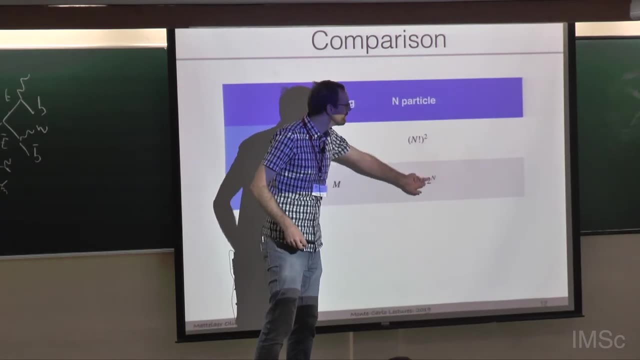 of dependencies. If you go to Elicity now you have the dependencies is only proportional to your number of diagrams, which is n factorial these times. But you have a 2 to the n simply because you have to sum over all the Elicity. 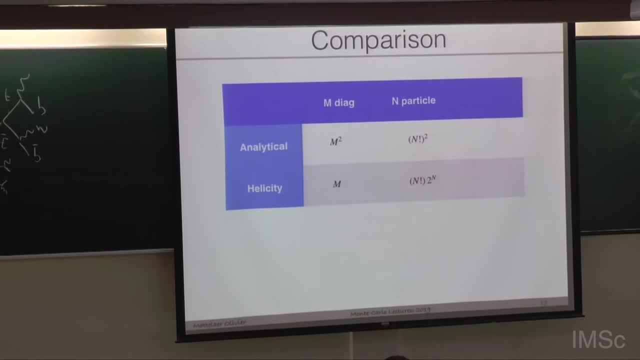 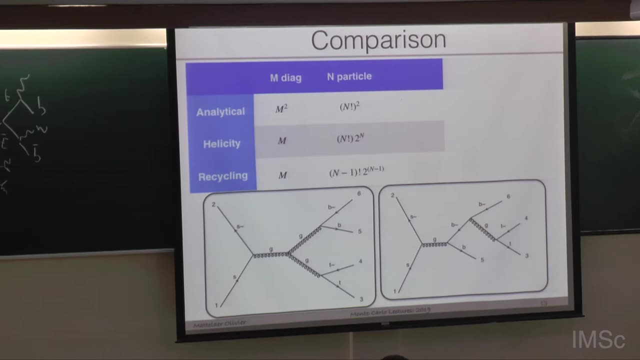 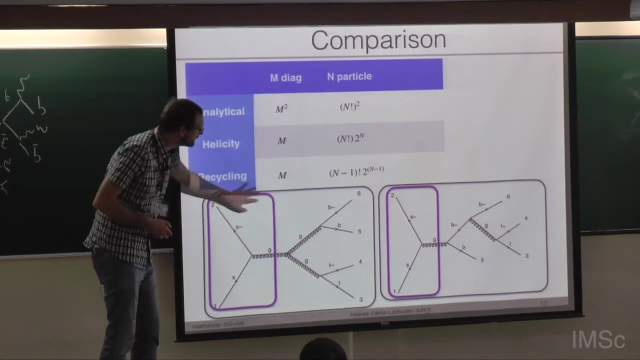 So you have this growing which is going back here. So now we can do a bit better in MadGraph, because that's still quite slow And what we call recycling. Recycling is actually realizing that some part of the computations, in this case this glion, this current 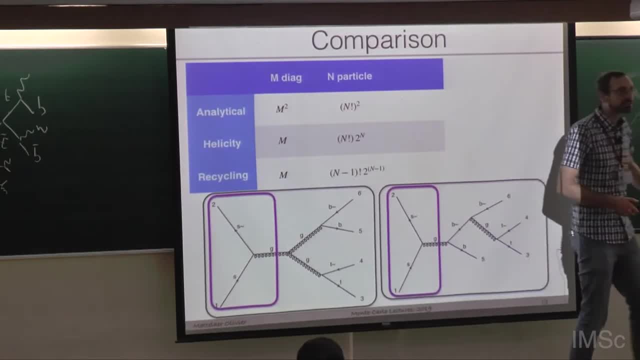 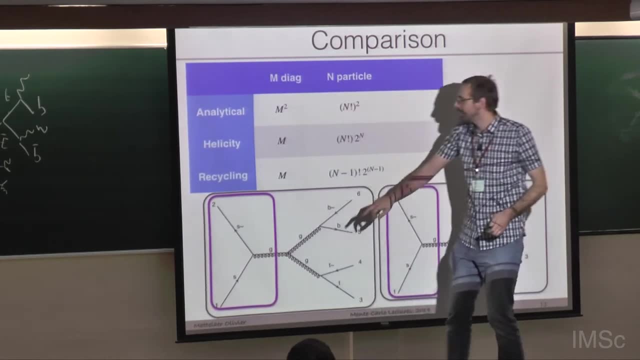 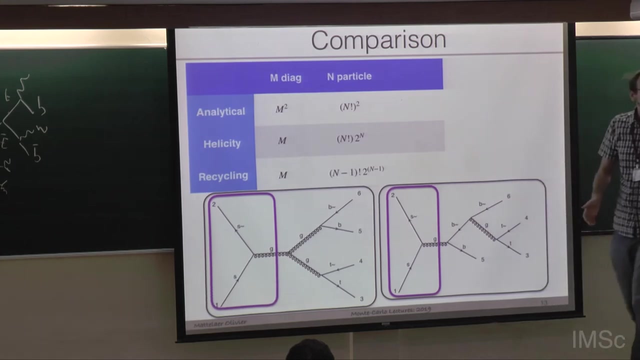 is actually present in multiple Feynman diagrams. So if I have computed this box, So the u bar v, gamma times the propagator j minus divided by q squared, I would have exactly need the same computations for these second Feynman diagrams. 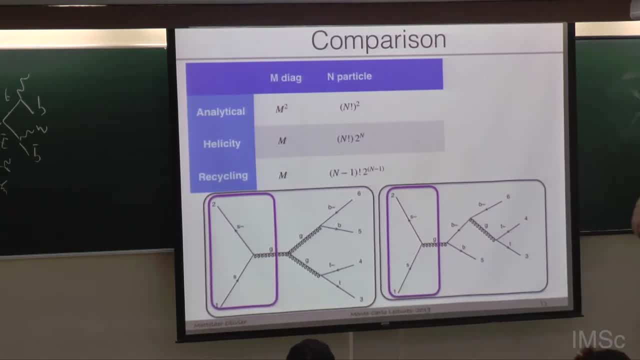 And therefore I don't need to redo the computations And that's basically save you one, That's give you one particle for free. So the time to compute five particles to do five case, you can go for free to do six, thanks to that. 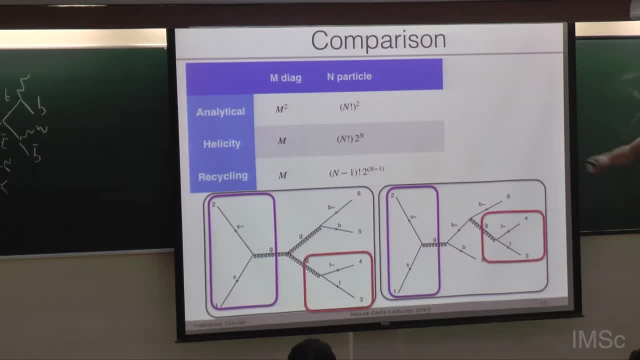 And that's what is implemented in MadGraph. And actually it's not only for initial particles, also this, in this case, final state particles- you can share in this case as well. So that's a lot of recycling. That's why it's called recycling, saying oh. 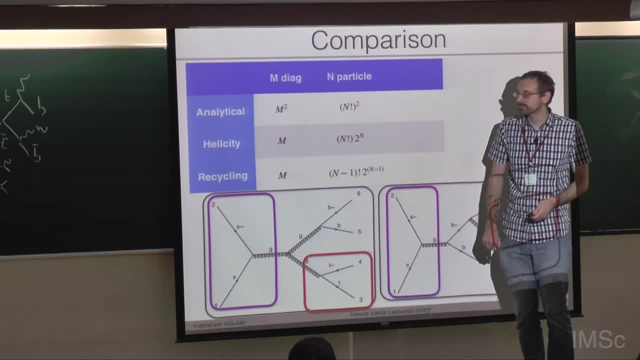 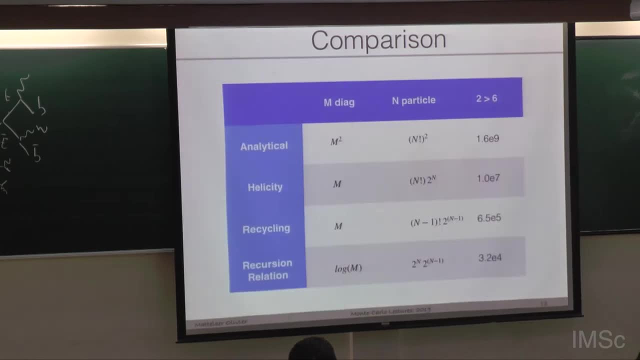 when I'm trying to compute these Feynman diagrams, I don't need to do the first step because I already done it, So there are actually ways to go even better than that, And that's something that is not done inside MadGraph. 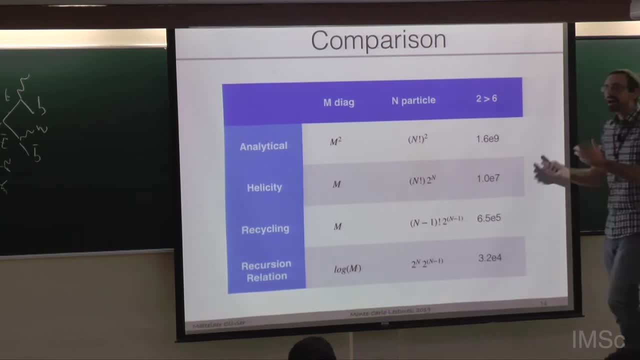 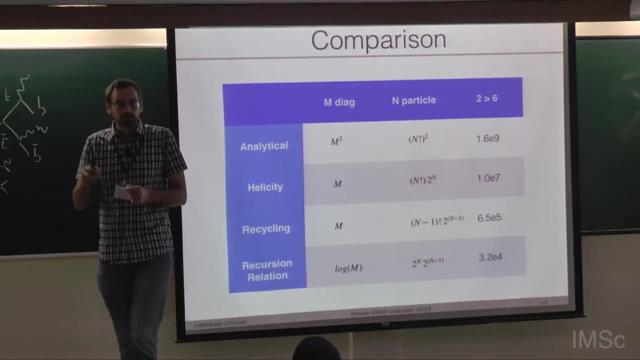 And that's called recursion relations And that's recombining some propagators together. I'm not going into the details. What you lose, What you lose as information, is the amplitude for each Feynman diagrams. So in the ECT, even in the recycling case, 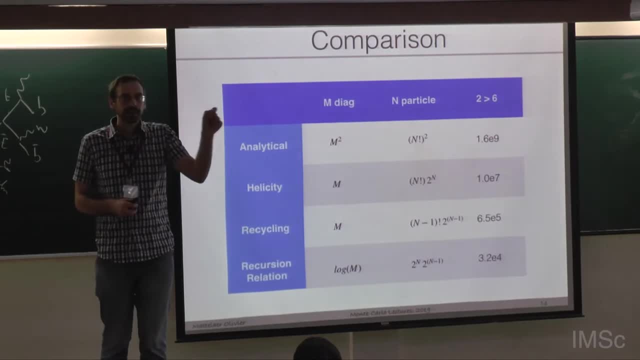 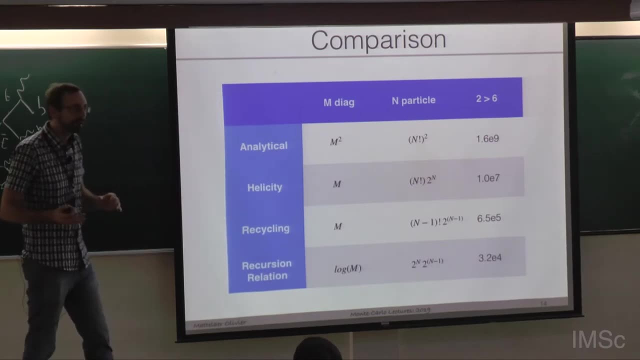 I know what is the amplitude for each of my Feynman diagrams. That's something I will use later. So that's why it's important to realize that In the recursion relations I'm losing, that I'm computing less number than my number of Feynman diagrams. 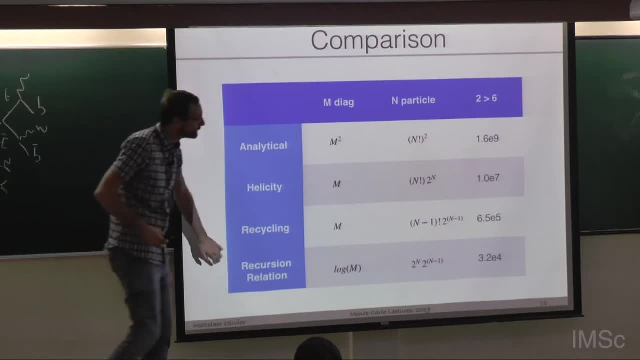 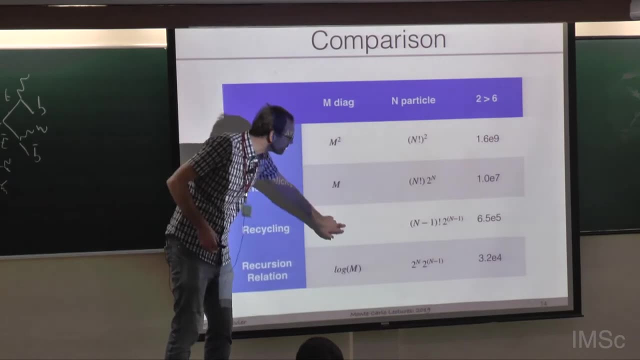 because I'm summing Feynman diagrams together actually in this case. And then of course, you are going much faster in terms of evaluating the matrix element, But you will have less information and MadGraph you will see later. 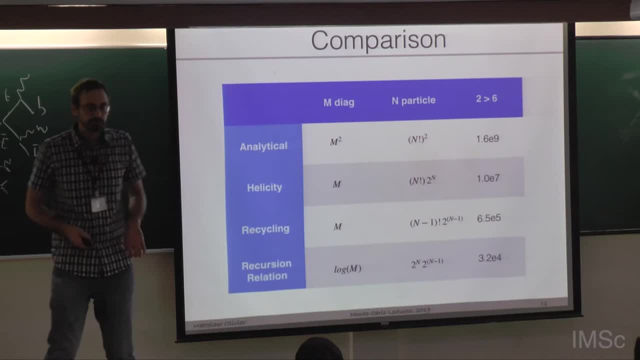 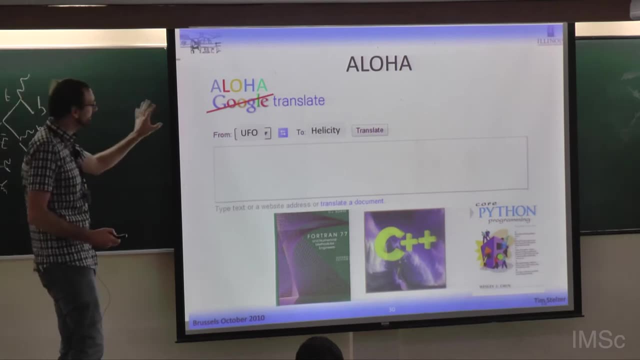 uses a lot of information of each Feynman diagram individually And you will see that in a couple of minutes. OK, So last comment: I guess Benj also told that already We need all those elicited routines. So each time it's a line, it's a function, as I said. 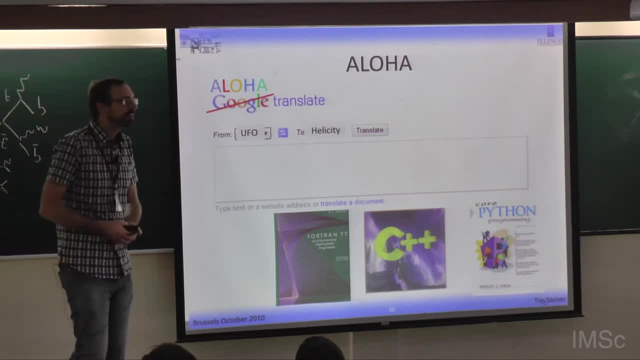 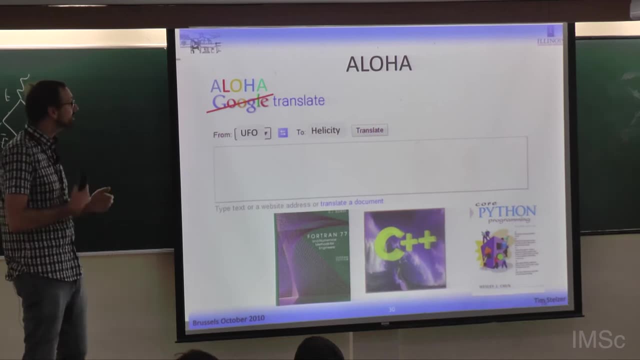 So we need to outcode that function into the code, And that was done originally for the standard model, then for Susie, then for some x-effective fields. So it's a very simple theory, but each time, for each model, someone has to write those functions for you. 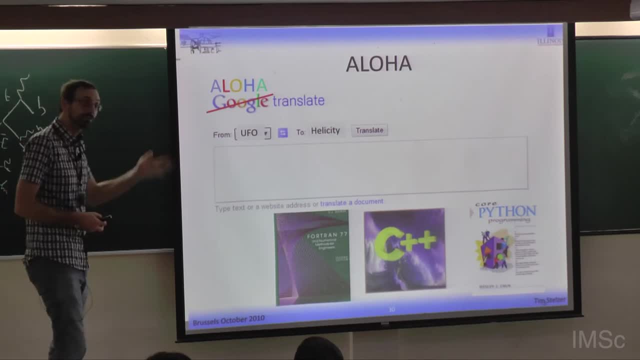 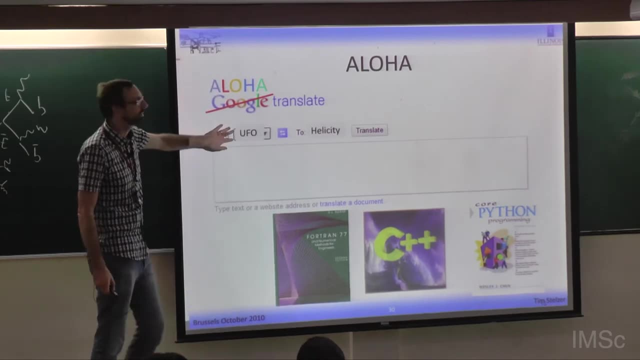 And that typically takes a month of work. So what we have done- actually now, a long time ago around 2011,- is to create a LOA, which is a translator. It takes your model and creates the functions for you. So very simple now, and that allows us to say: 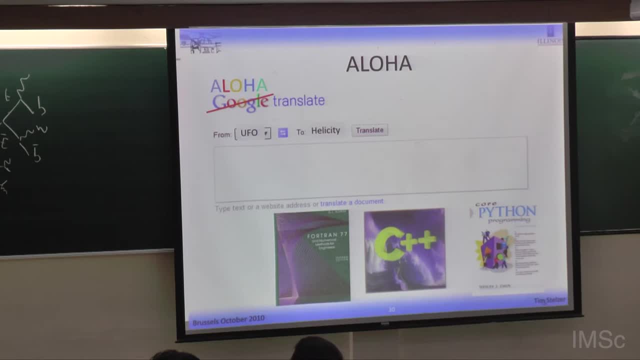 from any Lagrangian. you can now go and actually make the actual implementations, generation of events, completely for free, without having to take those long time of work, And that's really the job of LOA. actually, That's the idea. 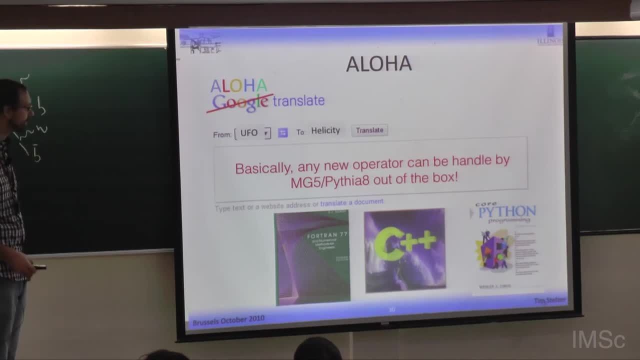 Any new operators, any new model you want, you can do it now. I'd like to give credit here to Tim Sledzer for these slides. So Tim Sledzer is the original author of MadGraph, back to 94, if I'm correct. 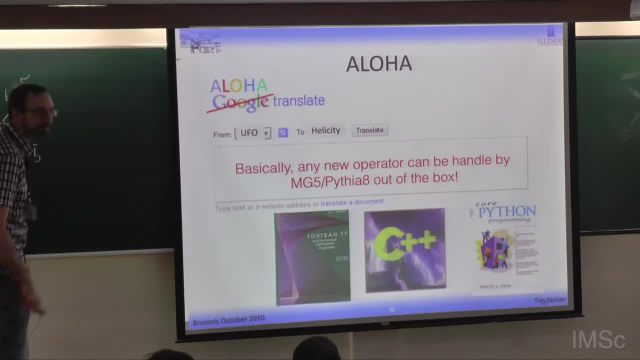 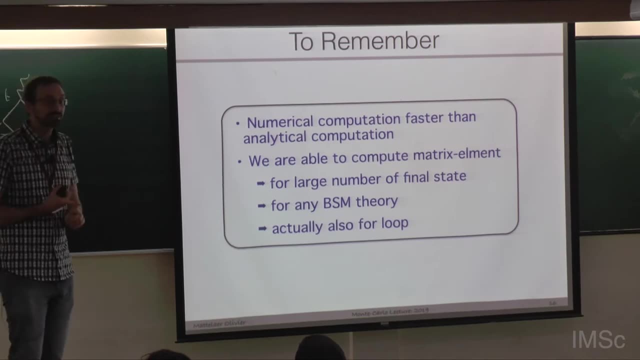 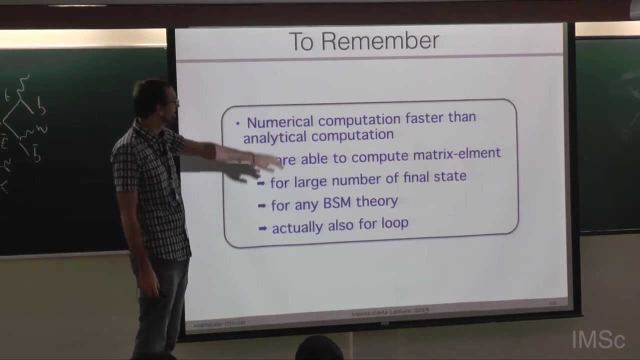 So the real first author of MadGraph was creating this slide. actually, I like it a lot, OK. so what to remember? numerical computation are faster than ethical computation. That's a key point. And then, basically, we are able to compute matrix element. 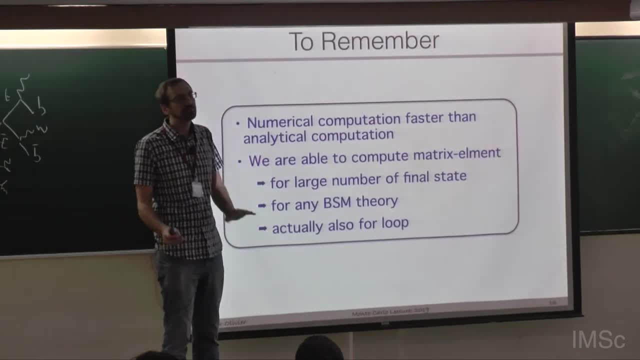 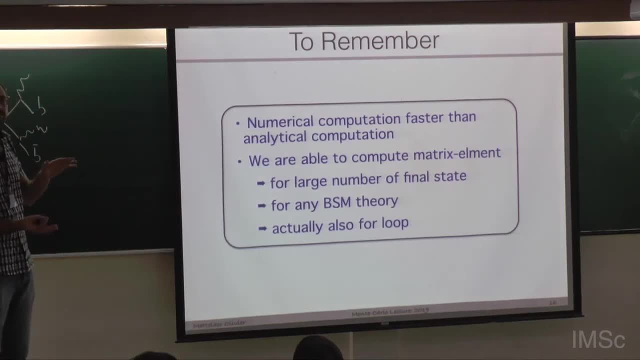 for large number of final states. Large still means quite small. right, It's six, eight, sometimes a bit bigger than that, But it's still quite small compared to what you learn tomorrow, when we can go to particles So large. you need to be reasonable what. 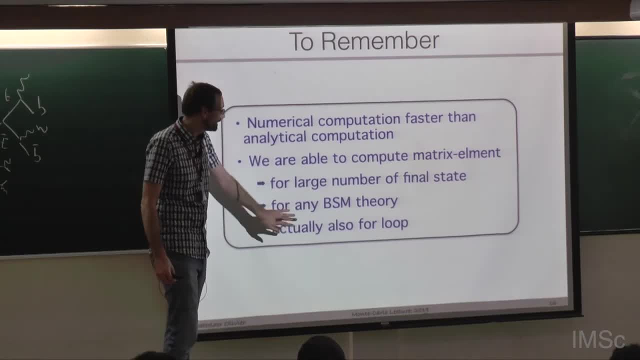 it means by large. We can do it for any BSM And actually we can do exactly the same for loop. So loop are a bit more complicated. I don't know if is going to enter in details. Yes, So you'll see also that the same infrastructures. 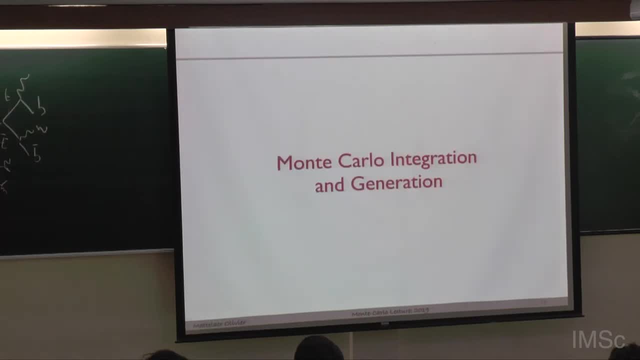 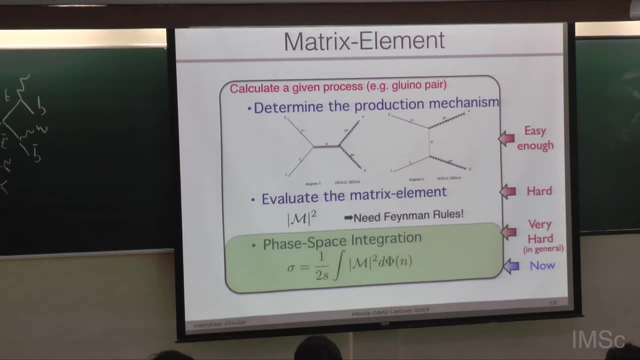 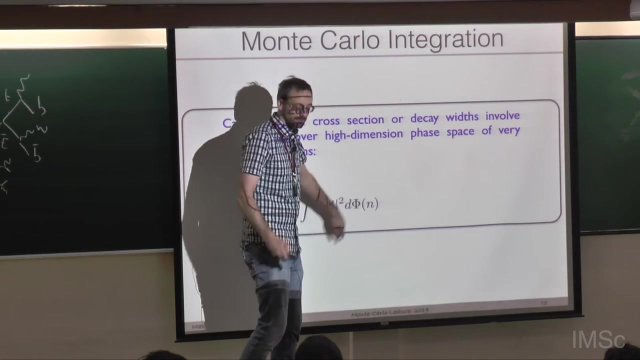 can be used for loops. OK, so next part, Monte Carlo, integrations and event generations. So that's what I was focusing about. So this integral is, in principle, quite simple. The only issue and the main issue here is the dimension of the phase space. 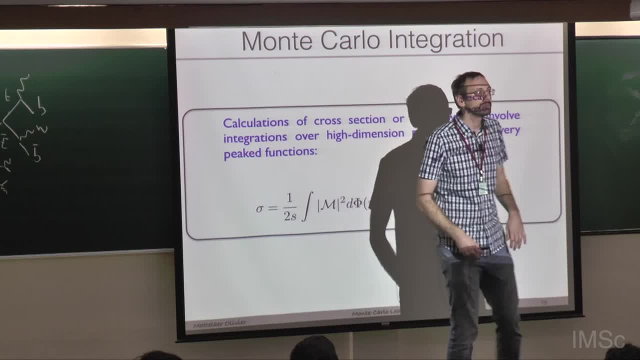 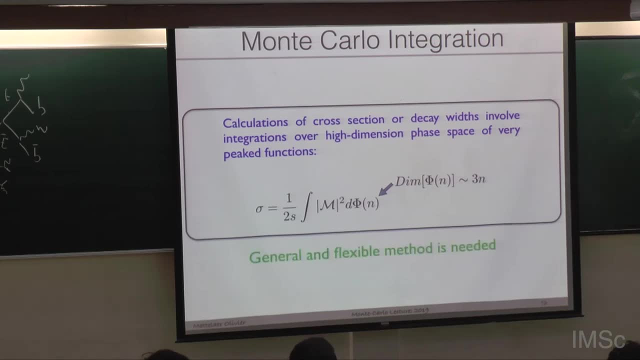 We're interested not in 2 to 2,, not in 2 to 3,, but typically in 2 to 4, at least, or 2 to 6.. So this number of dimensions is actually quite large, And that's a key, important point. 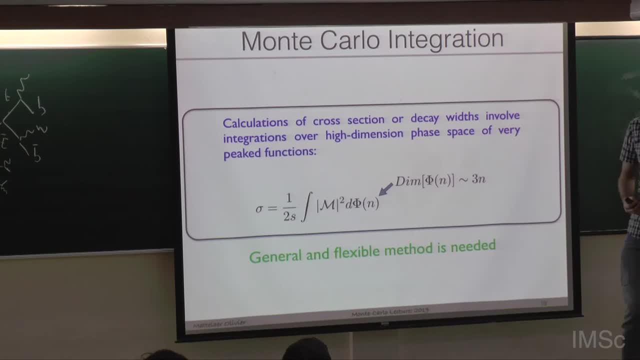 So of course, we also want, inside MadGraph, to have something which is quite generic and flexible. So we want to be able to generate the phase space integrator for any model that you provide, for any process that you provide. So we need to have something that. 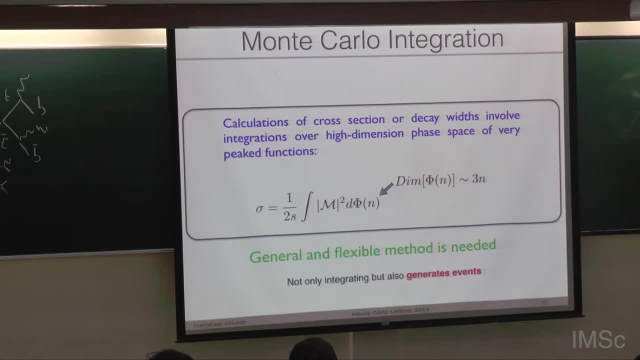 reacts to what you are asking us. And of course we're not only interested in doing the phase space integral here to have the cross sections. What we want to provide is events, So we want to provide representatives, so that histograms that can say: OK, that's. 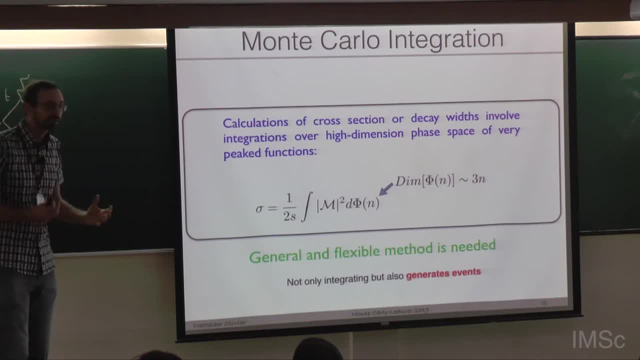 what you're going to observe in your detector for a given PT, for a given. So we really need to have events that after that can be passed to the pattern show and so on and so on. So we need to have a way to generate. 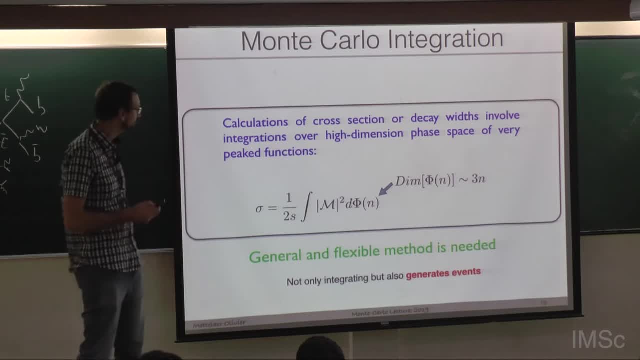 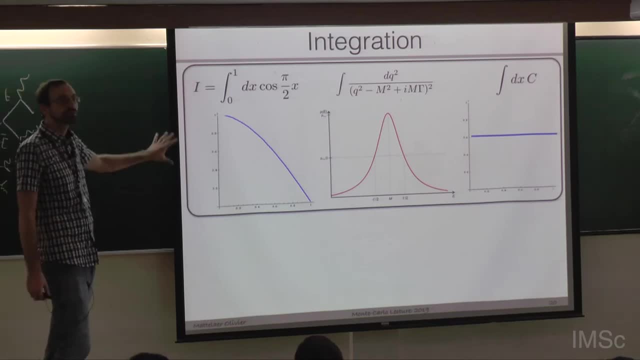 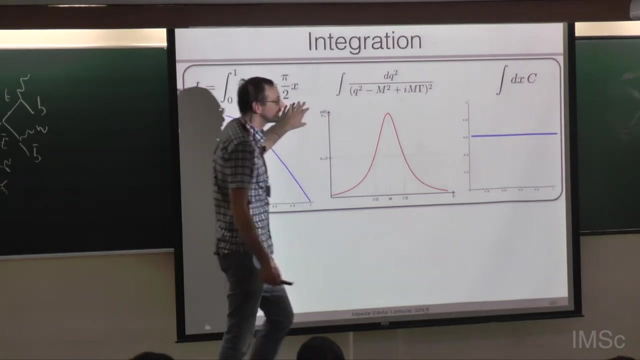 representations of what you observe in your detector at the end of the day. OK, So let's go back to very simple stuff. So here I'm going to focus on three functions, three very simple functions, a cosine that you can all integrate analytically. 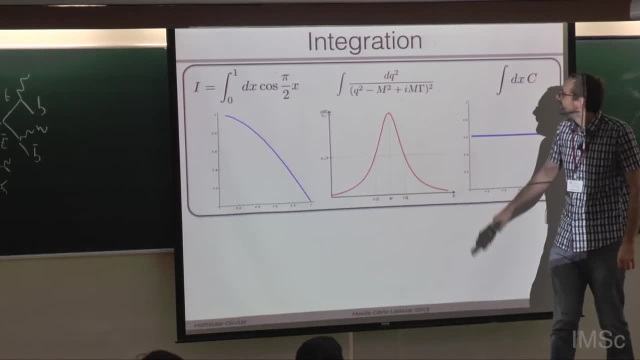 if you remember if it's plus sign or minus sign. I never do. The second function is also very simple, more difficult to integrate analytically, It's the break Wigner, obviously. And the third one is, of course, very simple as well. 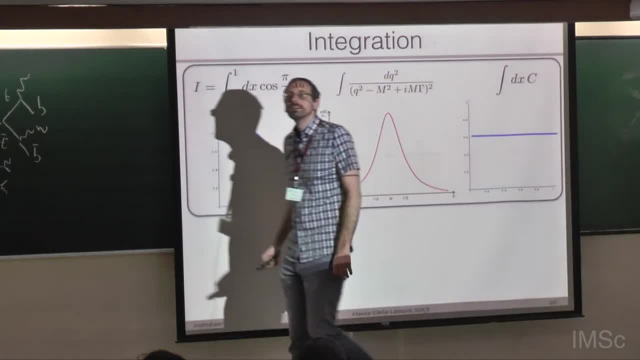 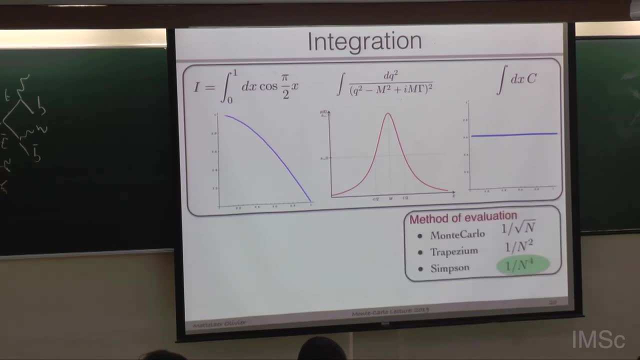 It's simply a flat function. So if you open textbooks in mathematics, you will learn that there is three main methods you can do here, And they are called Monte Carlo, Trapezium and Simpson. And here I present you the speed of those methods. 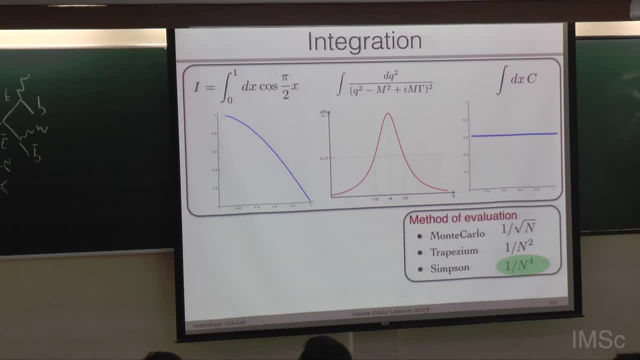 So Monte Carlo is actually the worst. It's one of the square roots of n. n is the number of times you need to evaluate the functions in order to get a given error. So the more the power is basically, the more you can do. 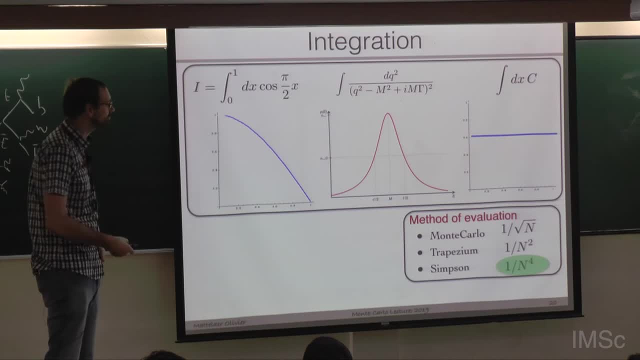 is, the power is very slow, So that means you need to really evaluate a lot of times your functions, While Simpson is 1 over n4, so that means you need to evaluate much less times your functions. So it's much better in this case, to use Simpson. 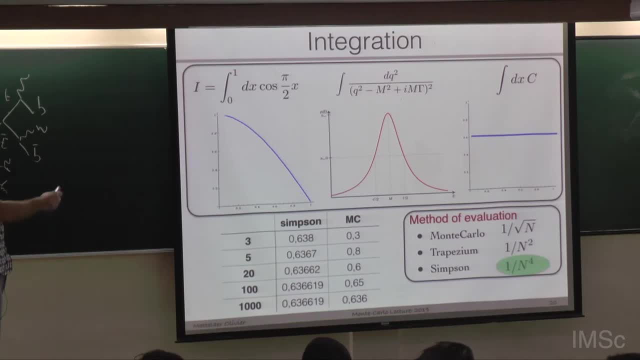 To prove you that this is an example with different value of n. So if I'm evaluating three times my functions, I have this number for Simpson- 0.638, while I have 0.3 for the Monte Carlo. If I'm going to 1,000 events- Monte Carlo, Trapezium and Simpsons. 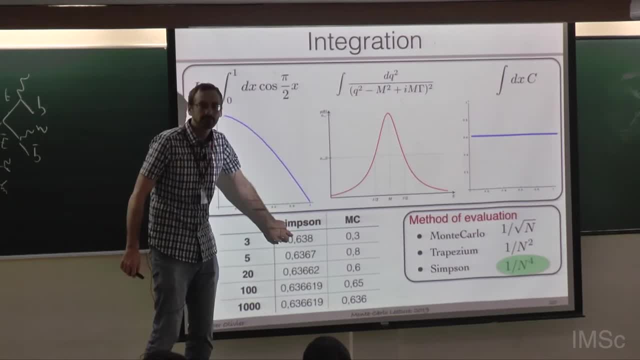 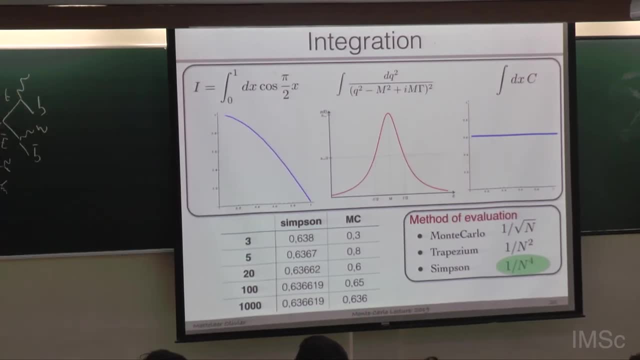 0.638.. Monte Carlo start to have a number which is kind of close of this one, And why? if I'm going to those numbers, something extremely precise for Simpson. So that just gives you how much slow Monte Carlo is. Monte Carlo is really, really slow. 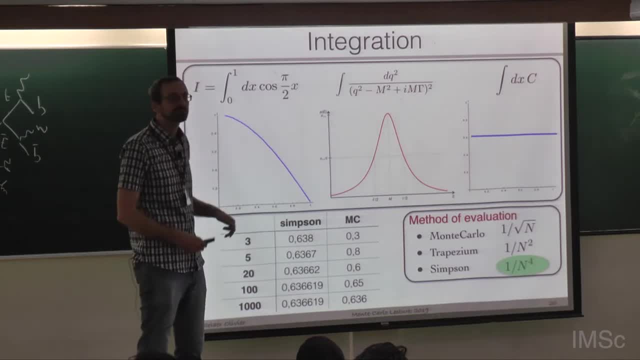 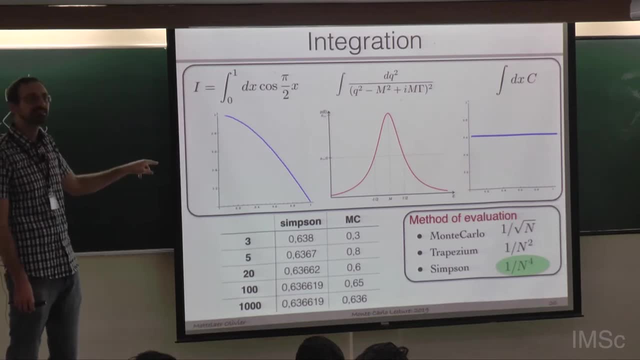 So if I ask you which method is going to use Mad Graph? who is going to answer Monte Carlo? No one. That's surprising, but good. Who was going to say Simpson? Couple of people, And you are so those who say Simpson. 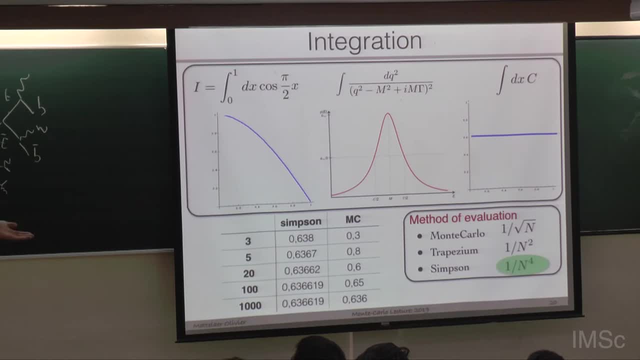 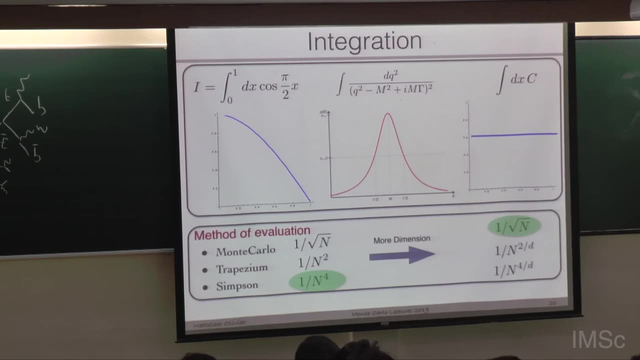 are actually wrong. We are using Monte Carlo, And then that sounds stupid, right? I just tell you how slow Monte Carlo was, And the reason is: if you go to higher number of dimension. So this was the case in one dimensions. 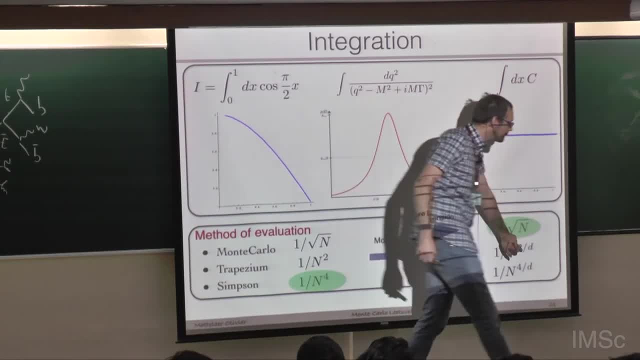 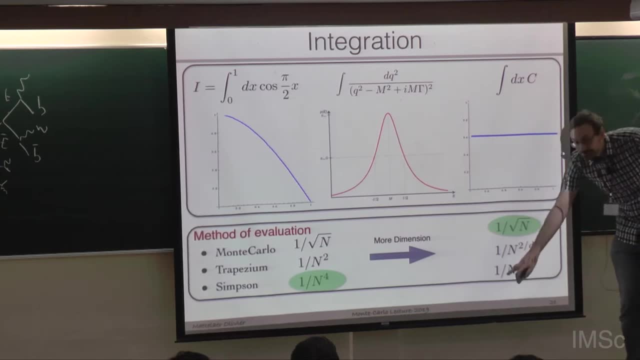 If you go to a higher number of dimensions, you see those number here if each times divide by d. So now, if you go to dimensions eight, Simpson was my fastest method- is now as slow as Monte Carlo If I'm going to d. 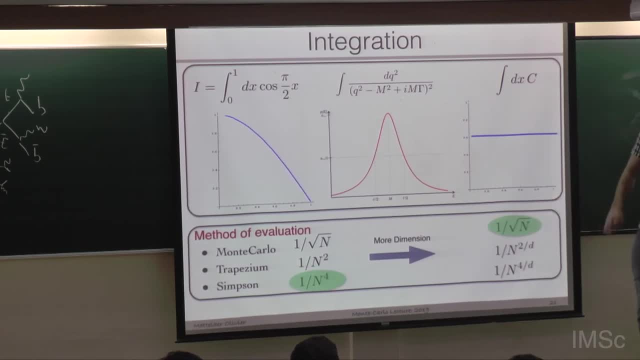 If I'm going to, d equals 10,. Simpson starts to be even worse now than Monte Carlo, And since we are interested in that regime- high number of dimensions- Monte Carlo is actually now the best- Doesn't mean it's extremely fast. 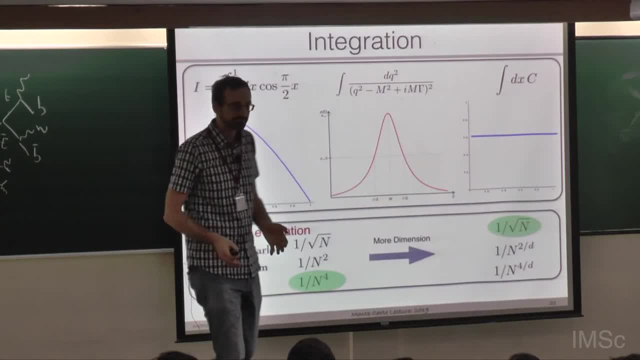 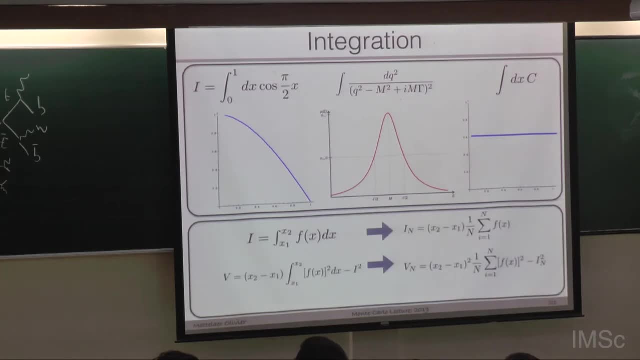 It's still extremely slow, but now it's the best method. So that's why we are going to Monte Carlo. So to explain what Monte Carlo is is just you take random numbers. So you take any random numbers between zero and one. 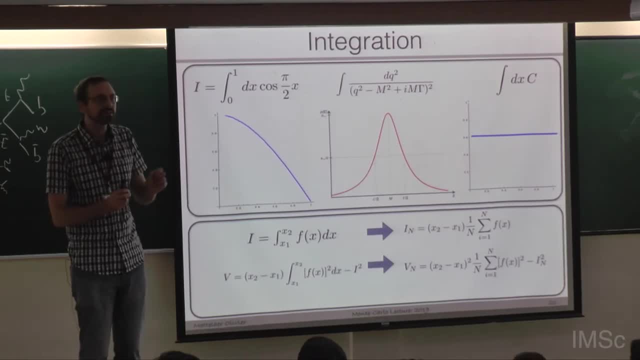 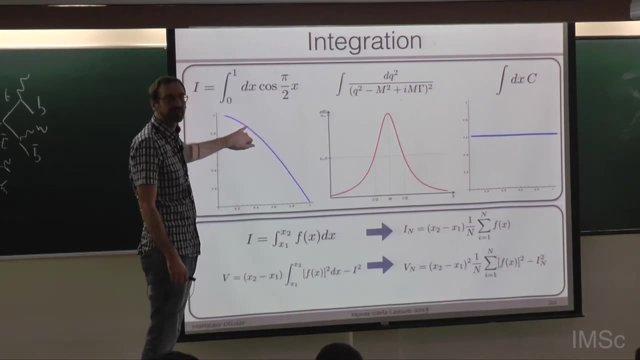 Completely arbitrary. You don't have any picking. oh, I'm going to take a number more in that direction and that direction. It's completely random. And then you evaluate the functions and you take the average, And that's what this formula is. 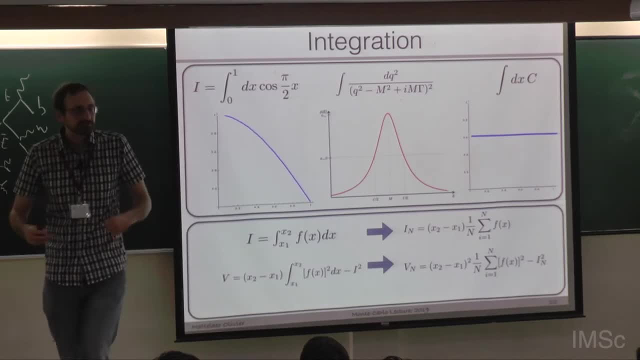 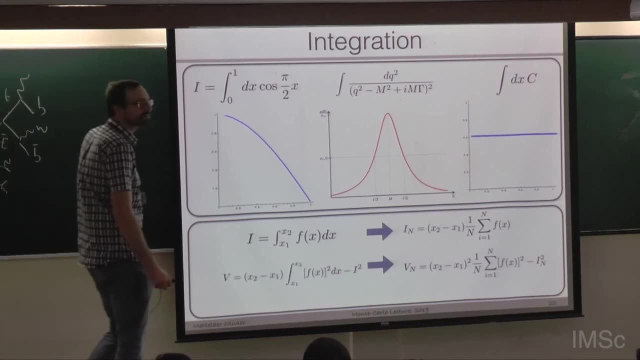 You take n random number and you take the average And if you take enough numbers, this is going to converge to the true value And, in order to have an estimate of the error, you typically estimate these functions, which is a variance. 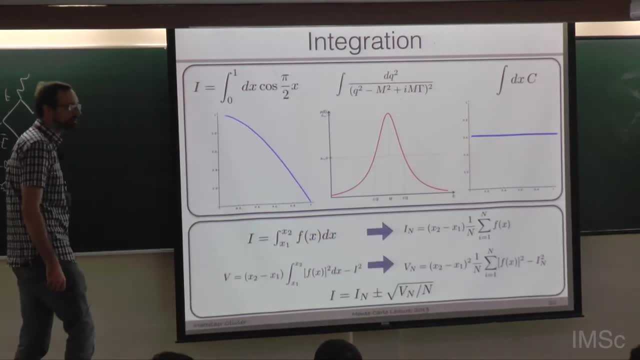 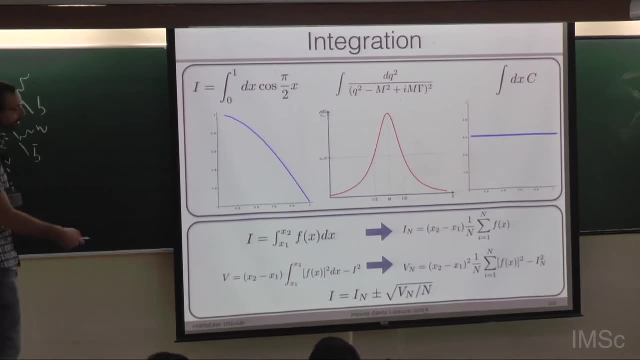 so the Of the functions And the actual error is the square root of the variance, of course, divided by square root of n. So the more number you use, the more accurate will be your result, obviously, And that's what I said before. 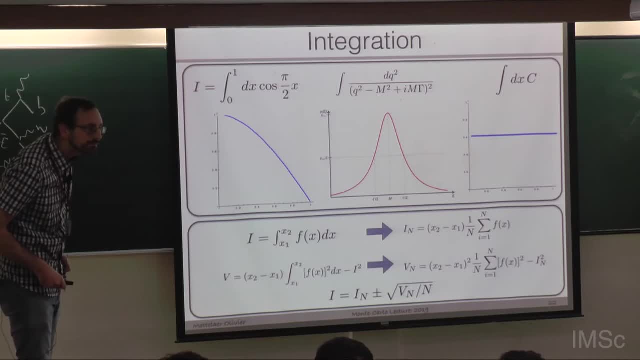 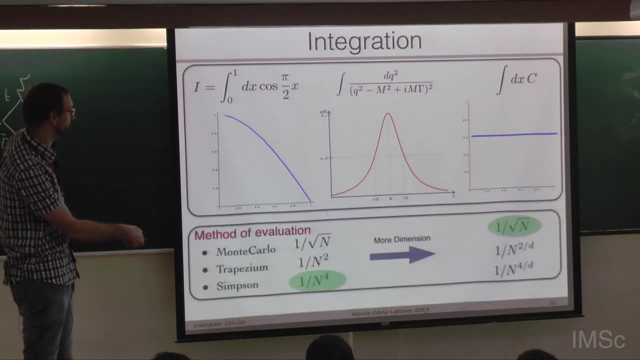 Yes, Is this from the Monte Carlo method? Yes, The error in Monte Carlo is always like this: It's like a. So in other methods that go back here, the error will be like this one times also: a prefactor, which. 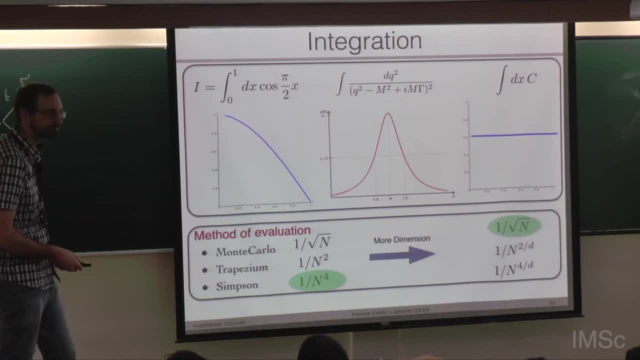 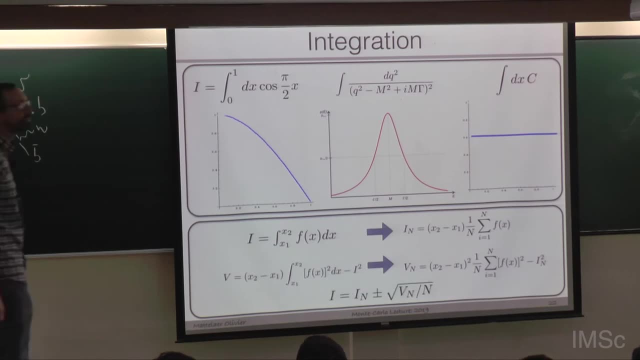 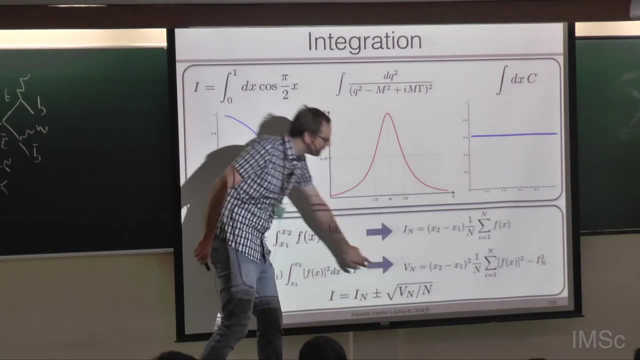 is typically also related to the variance. So now we can think which one of those three functions is the easiest to integrate, And you can really think two seconds on that. and the answer is quite simple, if you know that v is the variance. So the variance means how much you fluctuate. 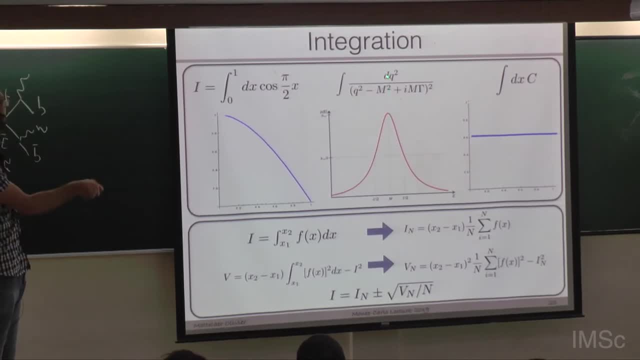 compared to the average, And here you have a function which fluctuates a lot. That's a break. Wigner, You expect to have a huge number here, a very small number here, So that variates a lot. So this will be extremely difficult to integrate. 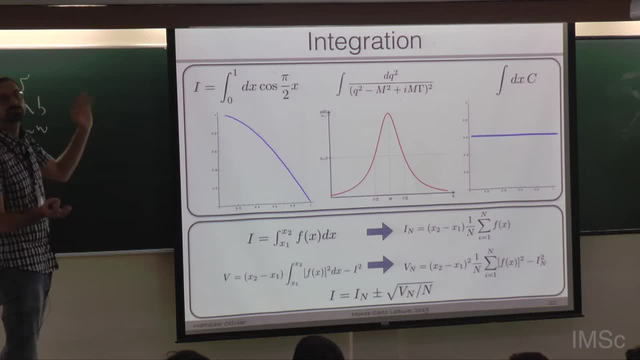 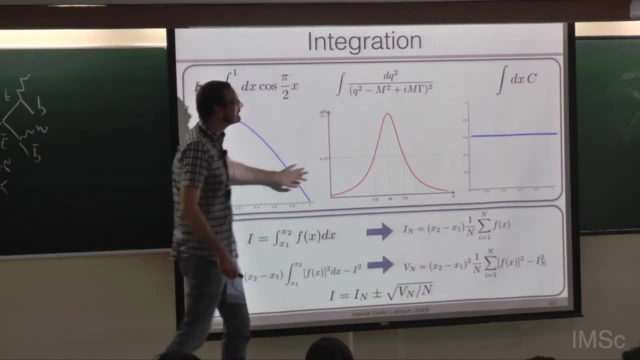 with this method. This one is going between 0 and 1.. It's a quite smooth function, a cosine, So that will not be too difficult to integrate. But this one is a killer because that's a function which is flat. 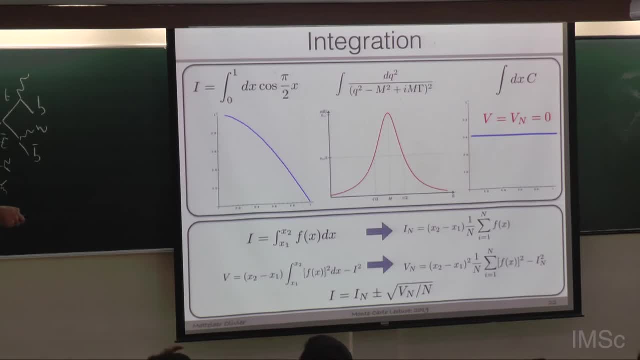 So if the function is flat, it means the variance is 0.. In other words, in order to integrate this, you only need one point, And one point with the perfect result, you have the correct. If you take more points, you are just wasting your time. 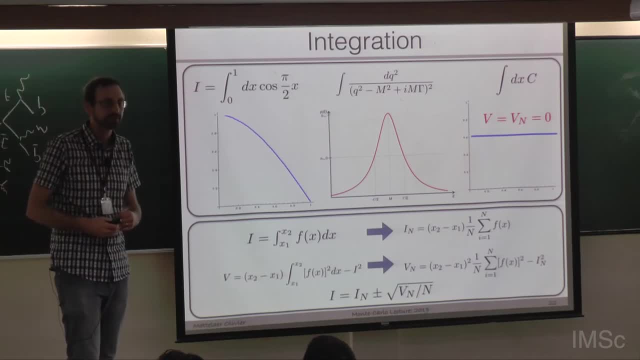 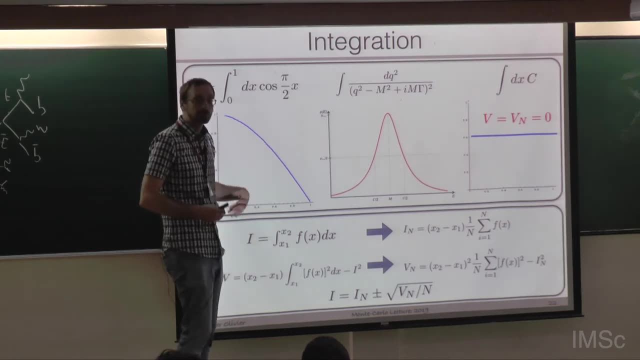 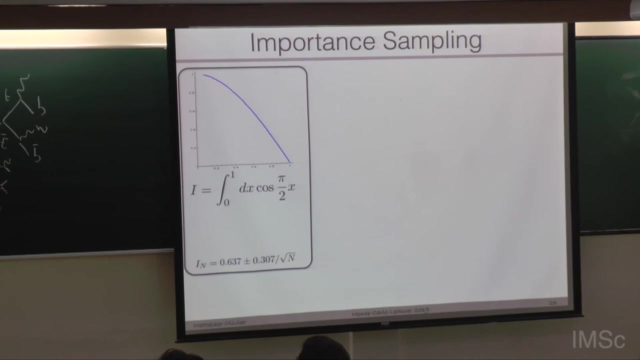 but you're always going to get the same result, And that means that we can use tricks actually to try to have the variance as small as possible, And that's what we are going to do now. This is called important sampling, But the idea behind important sampling- 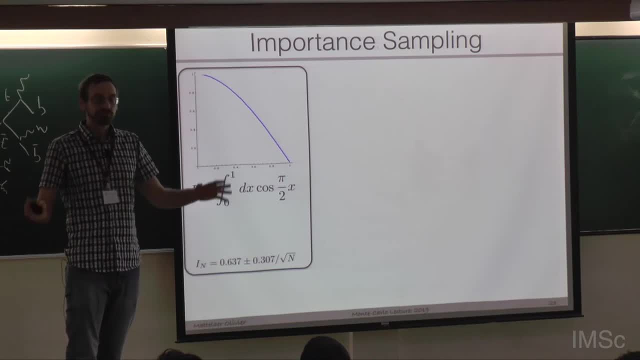 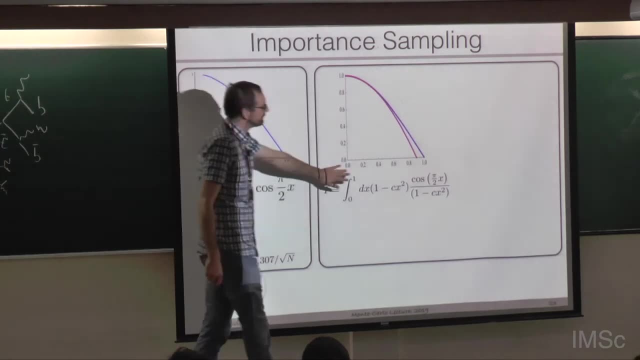 is trying to change the functions so that the function is now flat. In order to do that, I'm going to do a change of variables, So I'm going to multiply and divide by the same number, 1 minus cx squared, which is in this case, the Tyler expansion. 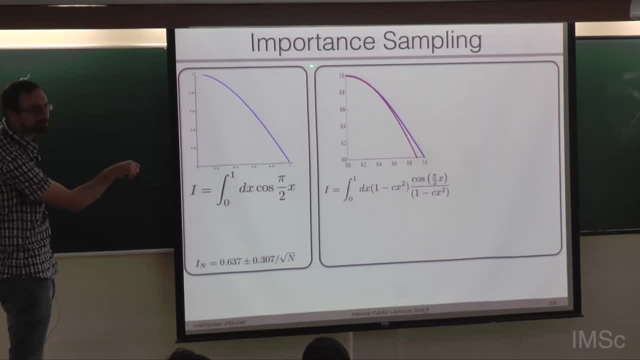 basically of the functions, And that is represented by this, It's red curves. So you see, it's very close, of course, to the cosine That's our Tyler expansion. And now I'm doing my change of variables, So I'm taking this defined as dki. 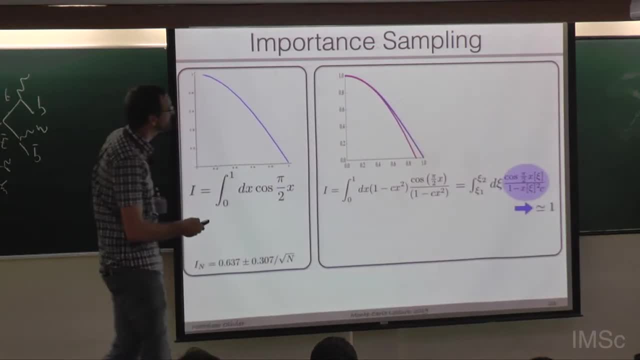 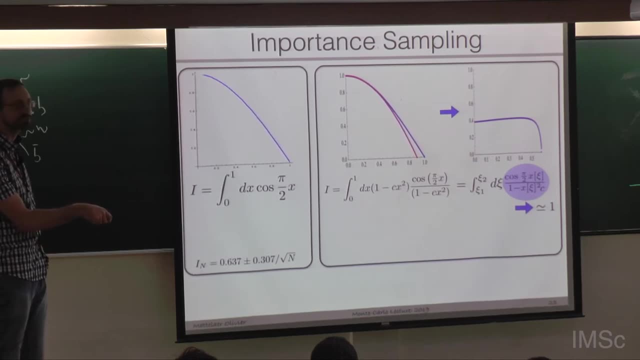 then I'm taking the change of variables associated to this And the functions, that result is actually this one And of course it's relatively flat, because I'm dividing the cosine by the Tyler expansions of the cosine and by construction. that should be relatively flat. 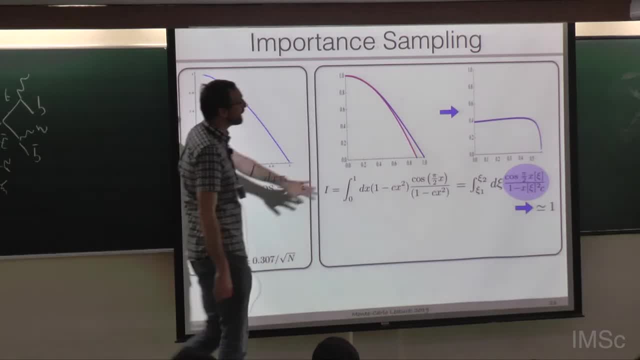 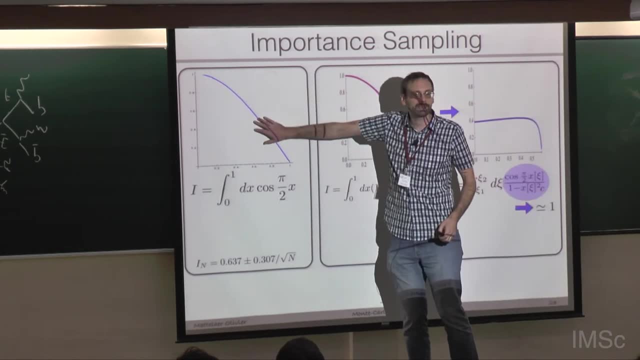 So this function now is relatively flat And therefore you expect that if I'm now integrating these functions, which for the cross sections will give me exactly the same number, if I'm integrating this one, I didn't change anything. I'm just doing a trick here. 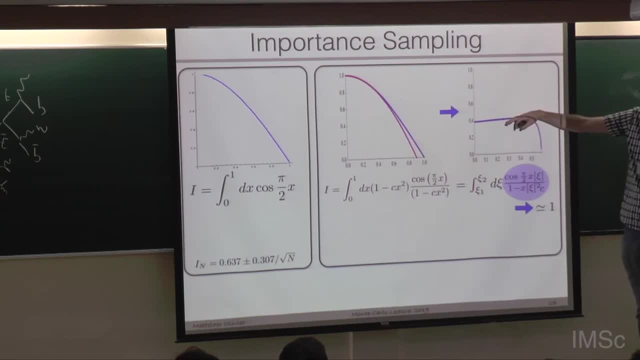 Now I'm going to be faster because my function is much more flat. The variance is reduced. So if I'm comparing the result, so this was the result in the first case. So I have, of course, the same value for the cross sections. 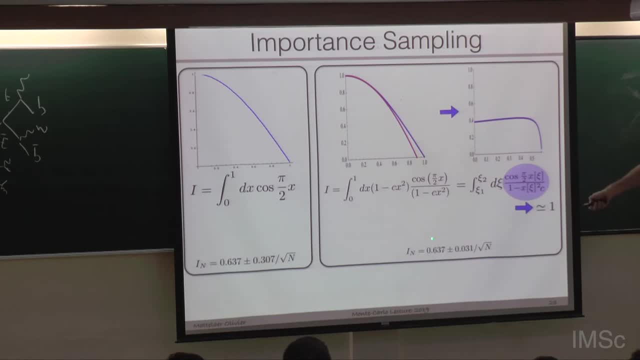 in both case, So 0.637 in both case, But now you can see that my variance is modified. So in this case, my variance is actually 10 times smaller than this one, which means that, in order to integrate this by using these tricks, I'm going 100 times faster. 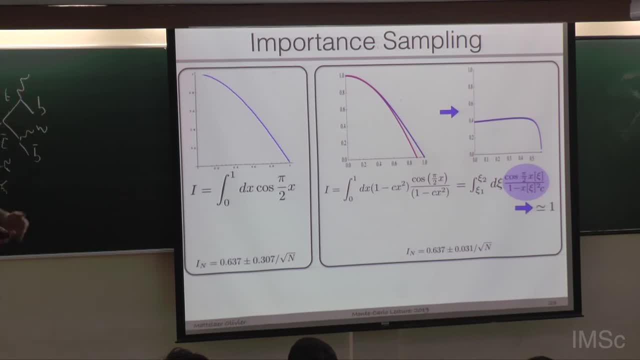 So that's a speed of our factor 100. So it's huge, But at the end of the day it's just a change of variables which makes my functions flatter. So I just want now to. we can do the same for the break, Wigner. 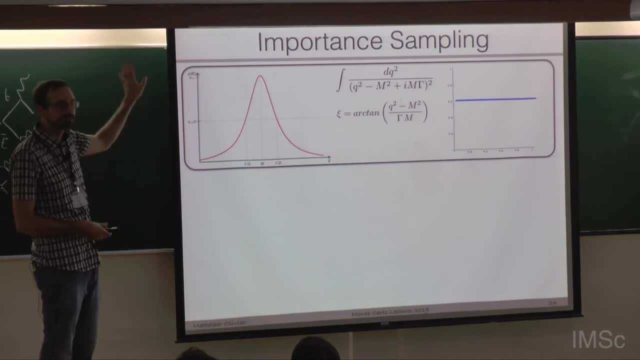 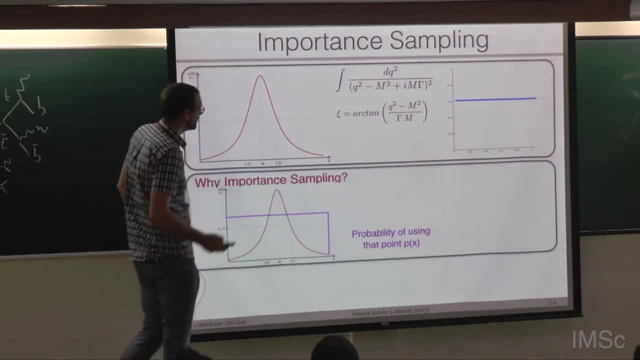 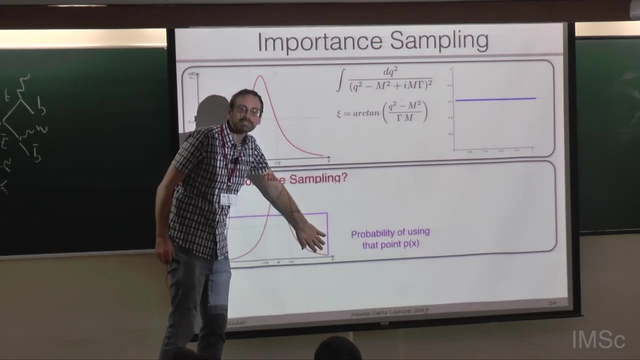 And here the change of variable is a bit different, But it's well-known in the community, It doesn't matter too much. I just want to justify why this is called important sampling And in the normal Monte Carlo the probability to take a point here is the same. 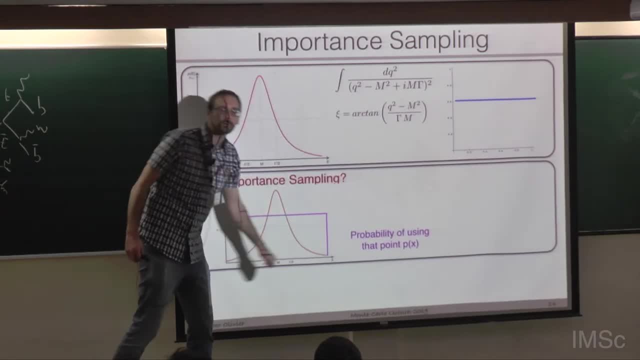 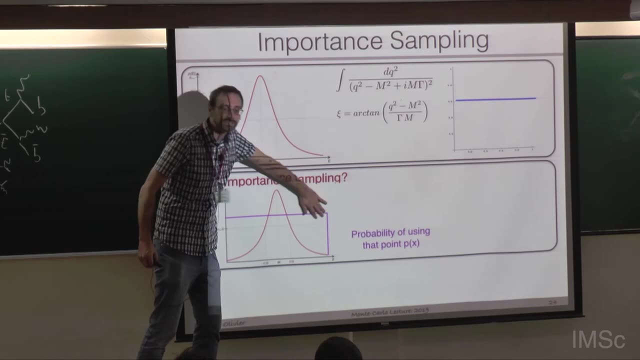 And now the probability, to take a point. I show that by these purple curves, Which is what is the probability to probe a given point. And the idea of Monte Carlo is everything is probably flat. So that's why this function is always 1, or always a given number. 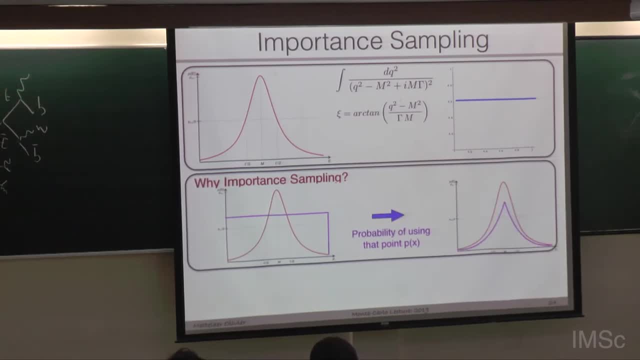 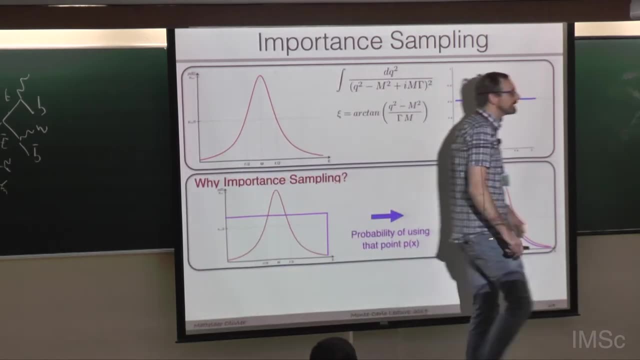 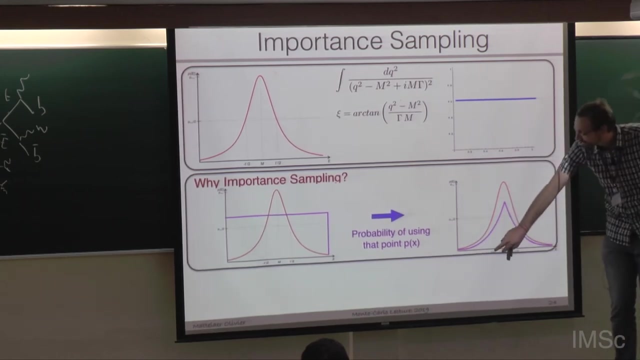 So that's the probability to pick a given point. Now, if I'm doing my change of variables, what I'm doing, I'm saying my code. when I'm probing these variables, I'm actually going to probe my real invariant mass And most of the time I'm actually 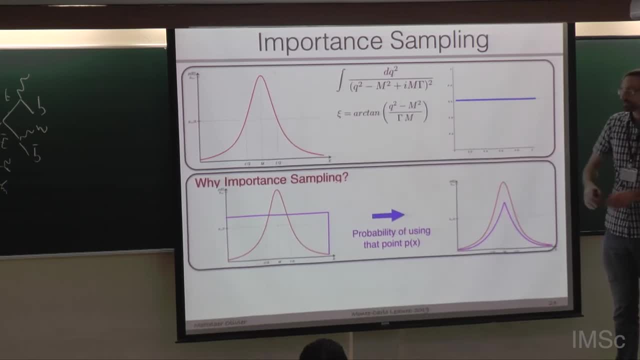 going to evaluate the functions here. In other words, it's important to the integral correct that I know precisely what is the value close to the peak. I don't need to know too much about where the function is small. So that is why it's called important sampling. 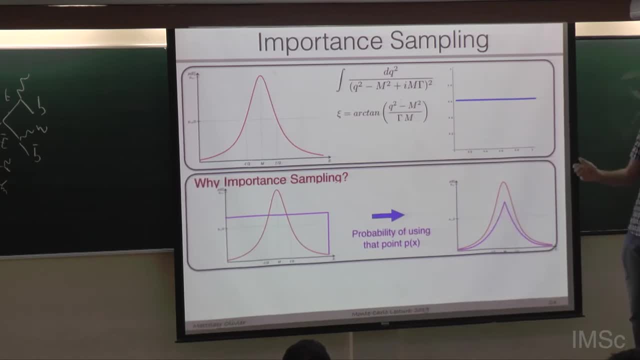 Because I'm going to probe not flat anymore, like in the standard Monte Carlo, But I'm going to probe according to the functions. The more often why the function is high I'm going to probe quite often, And when the function is small I don't care too much. 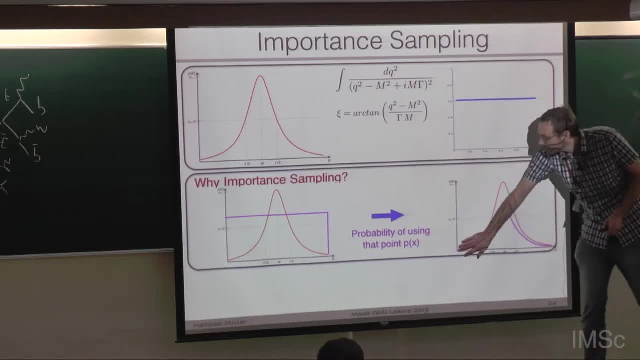 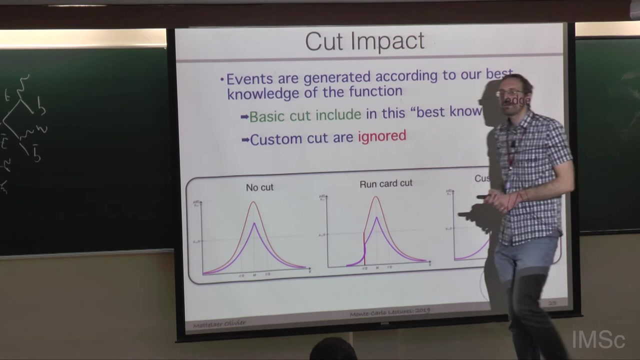 So I'm going to probe very, very rarely, And that's why it's called important sampling, because you're probing according actually to the function itself. OK, Yes, So why? I want to stress that a lot? because it has one impact for you. 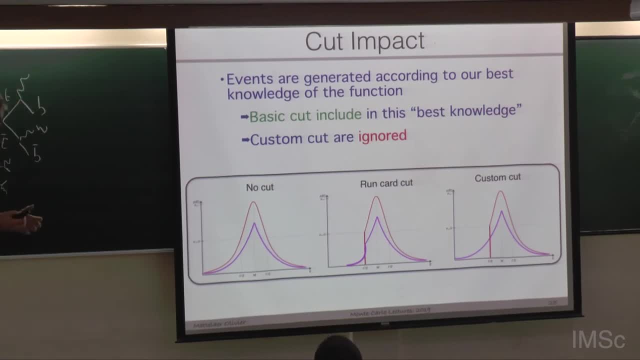 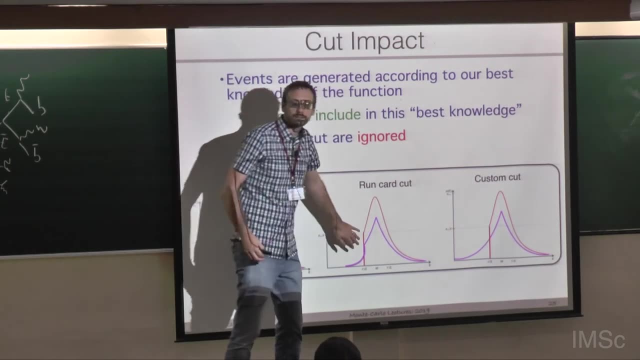 is when you impose cuts. So when you impose a cut in Madwell, let's say you put a cut in invariant mass, like in this case, here, you're going to change your functions quite a lot And MadGraph needs to react on that. 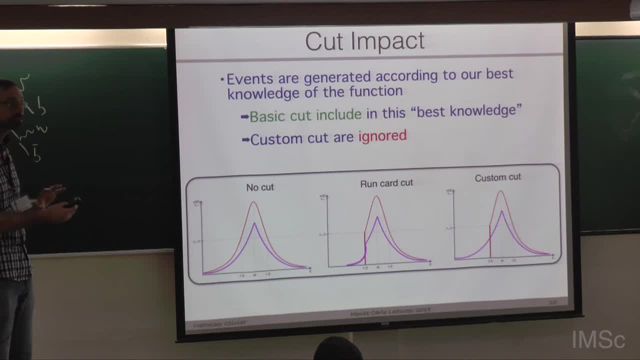 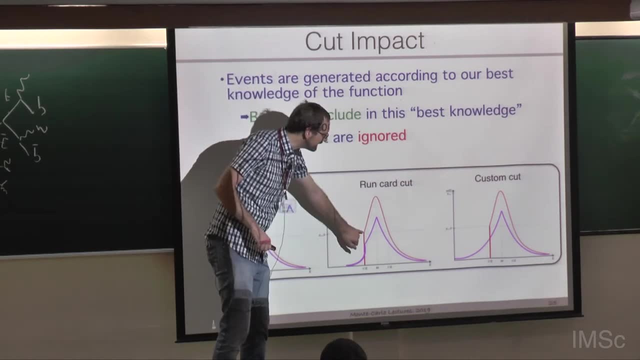 to change the way we probe the phase space to include the fact that it's a cut And in normal MadGraph, what we are going to do? we're going to change the phase space and therefore say, oh, now your function is zero in this case, 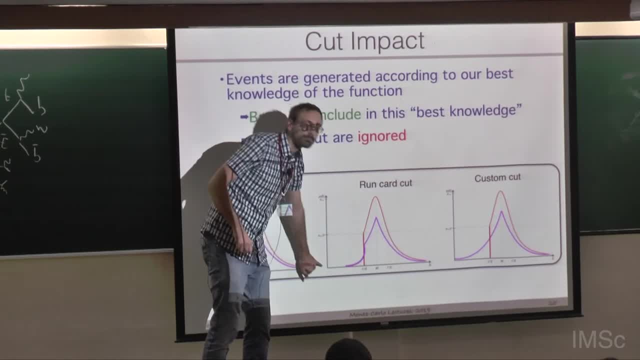 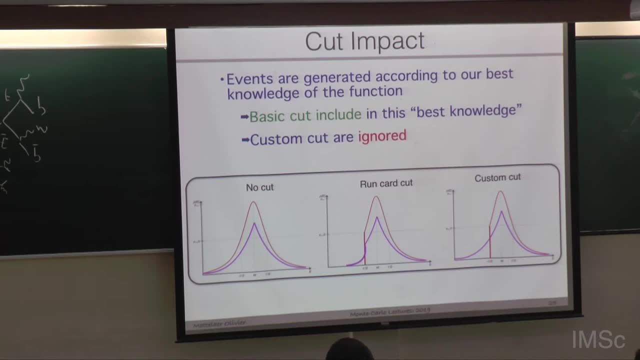 So we need to know that and basically try to not probe this part at all Because it's zero, we don't need to probe it And we try to do that analytically. There are sometimes users who don't use the predefined cut. 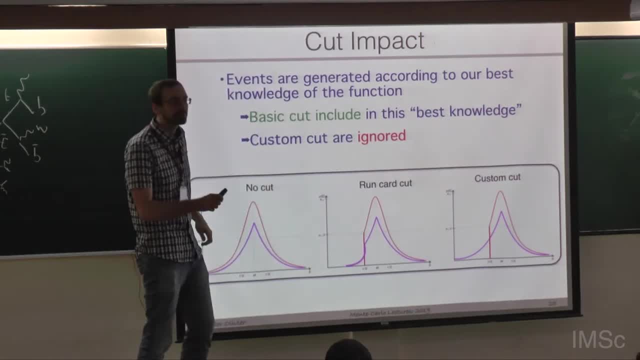 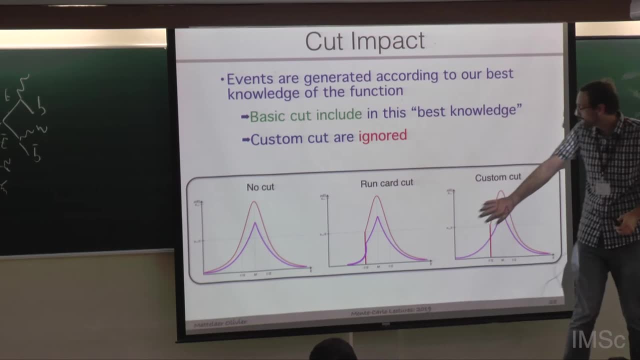 that we allow and that we're using, that They just go inside the code and output their cuts. In some cases, that's the only thing you can do if it's complex cuts. What's going to happen in this case is this: 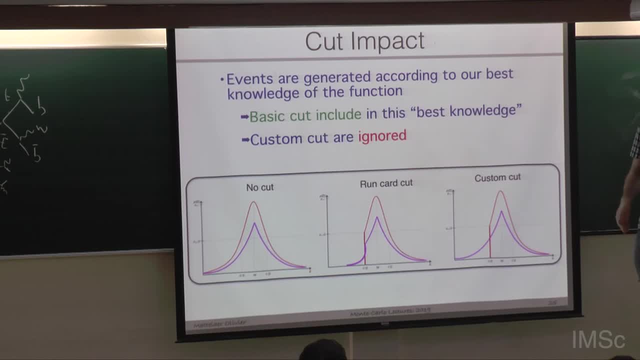 Your function will be cut, but MadGraph has no idea that you have put the cut there. So MadGraph is still going to integrate as normal, at least at the bottom. It's the beginning, And then it will react, but much later. 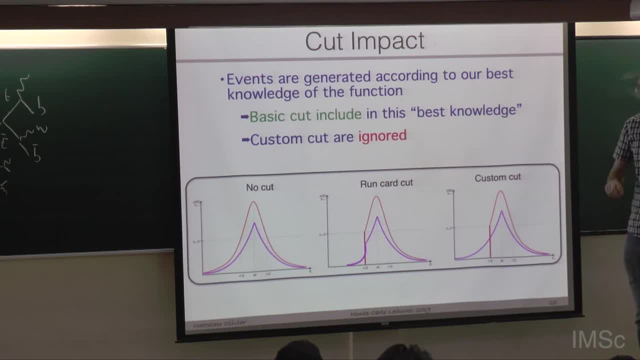 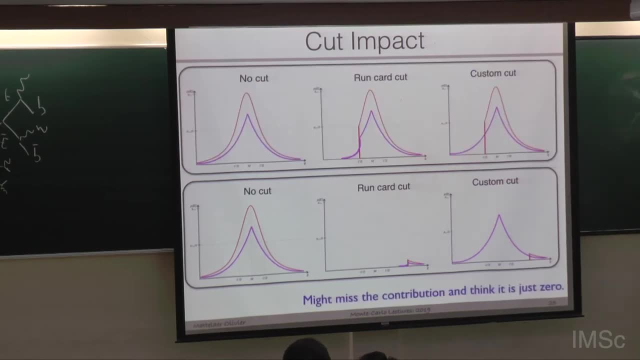 And in this case your cut is relatively mild, I would say So MadGraph is going probably to convert normally. no issue Now if I'm going to do the same now, but with a very strong cut. So now I'm basically cutting my full break-ziner. 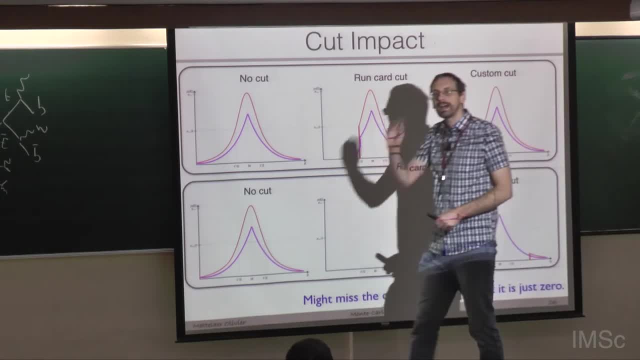 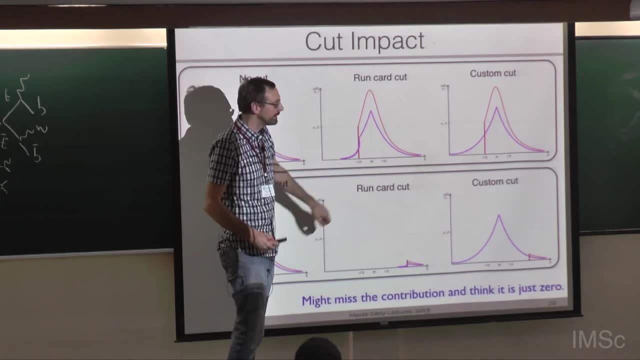 So I'm putting a invariant mass cut to 100 times the mass of the particles here. So very, very strong cut. If I'm doing inside MadGraph, MadGraph knows. oh OK, you are cutting the full break-ziner. 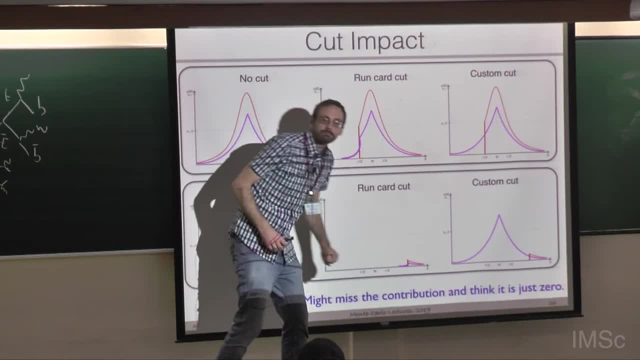 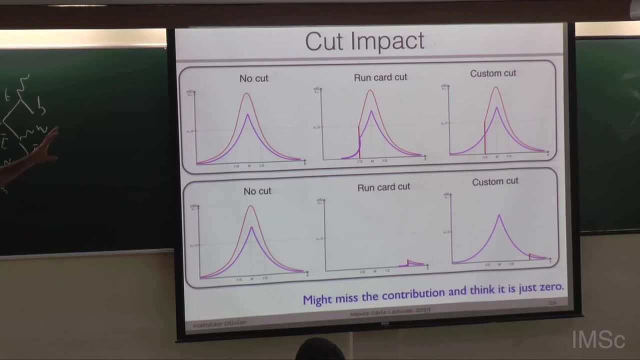 So I'm going to react And I'm only going to probe this part here And all these parts. we never try to reach it at all. So we exactly react in advance. We know there is a cut. We fully change our phase- space integration- targeting to it. 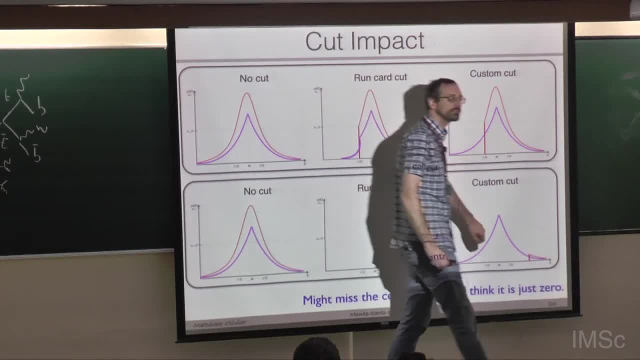 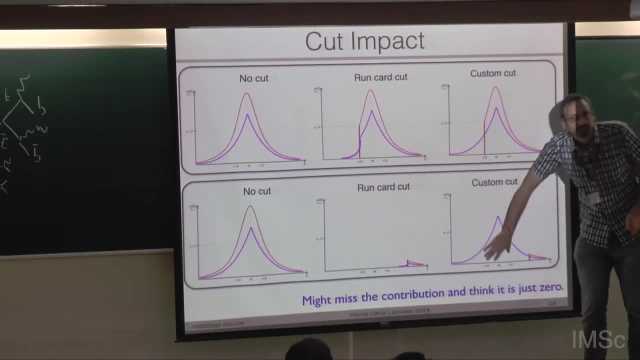 If you are encoding the cut yourself without telling MadGraph that you have a cut, what's going to happen? MadGraph thinks there is no cut And therefore it's going to launch a bunch of events, actually a lot, a lot of events here. 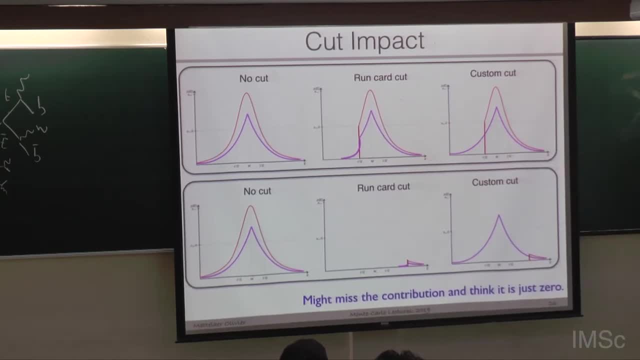 And we'll always receive the same answer from the code saying your cross-sections. your value for your functions is always 0. And after a pong, which is typically a couple of millions of events, since you will never have a value different of 0, MadGraph. 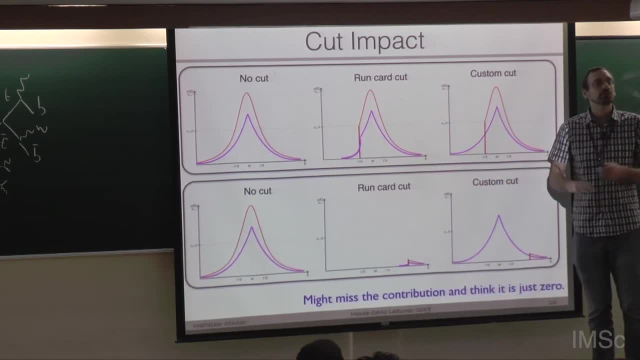 will return 0. in this case, It's just saying: OK, my function is always 0. That means this contribution is 0. And if that's what you are interested in, of course that's not the correct value And that's the worst-case scenario. 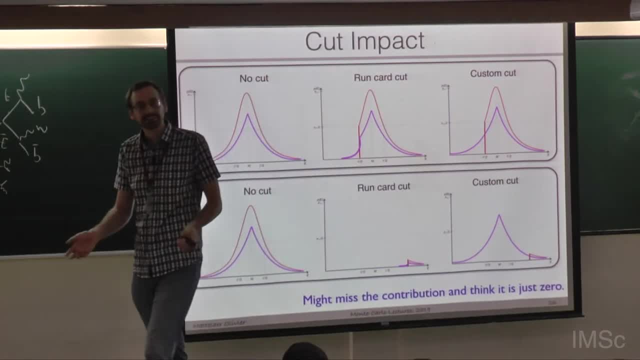 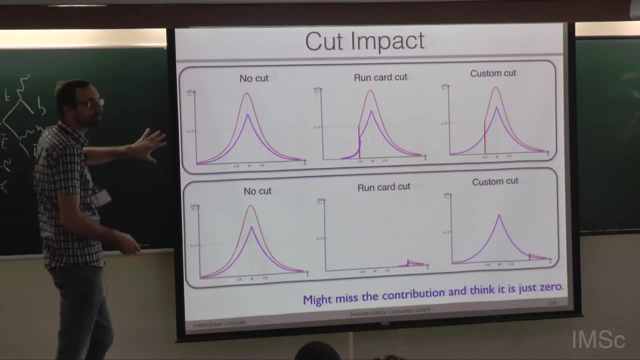 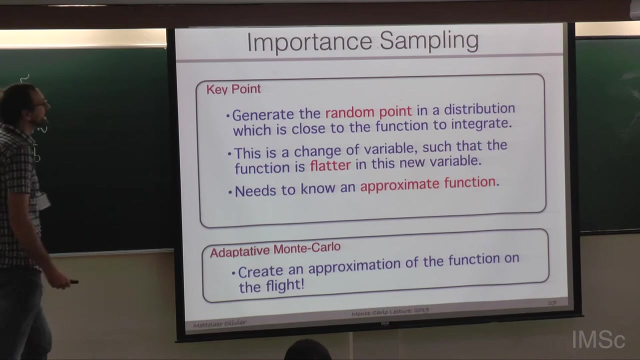 but still simple enough, because if you receive 0, you realize it. But sometimes you can just receive wrong numbers and then it's really really bad. So that's why you need to be careful about cuts. So, going back to important sampling what 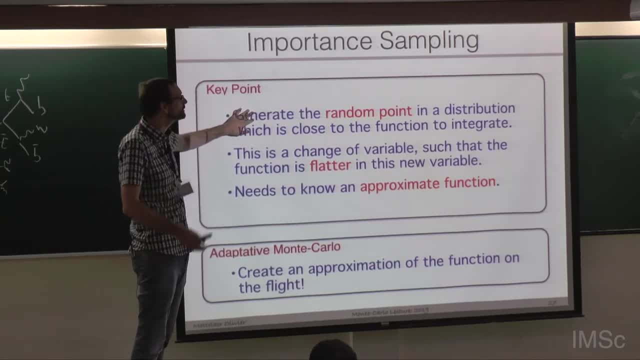 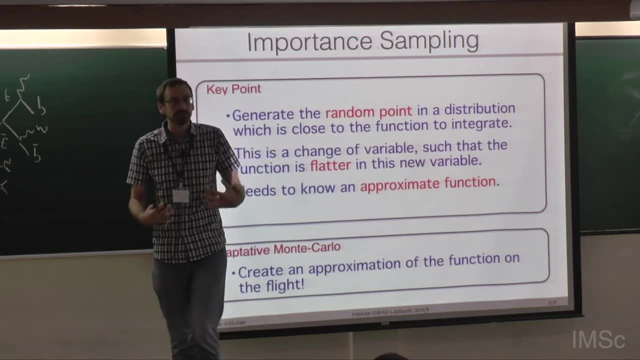 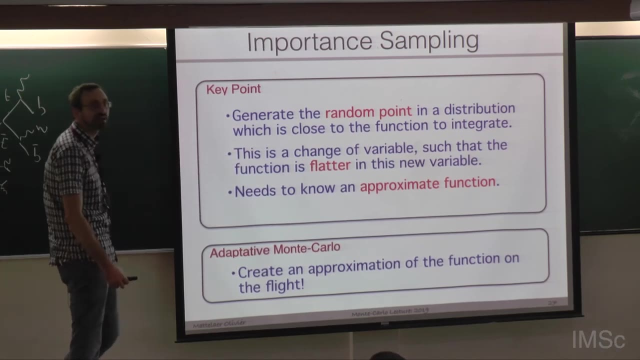 we do now in important sampling is we generate random points, but not in a flat distribution anymore, but in a distribution that is very close to the functions that you are integrating. So that's why it's called important sampling. So this, in other words, this is a change of variables. 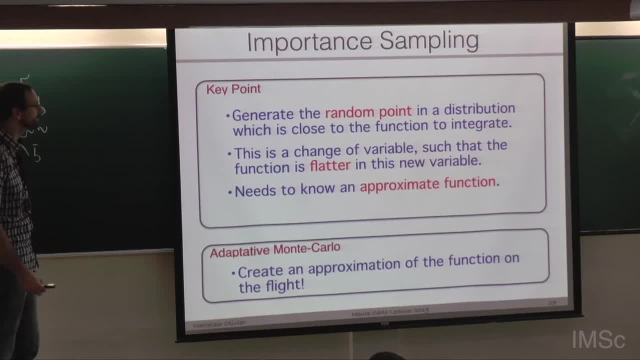 which makes the function flat, which allows to have much faster face-to-face integrations, And the key point here is that we need to know the approximate of the functions in advance, And that's something that we need to Now. on top of that, what we can also use. 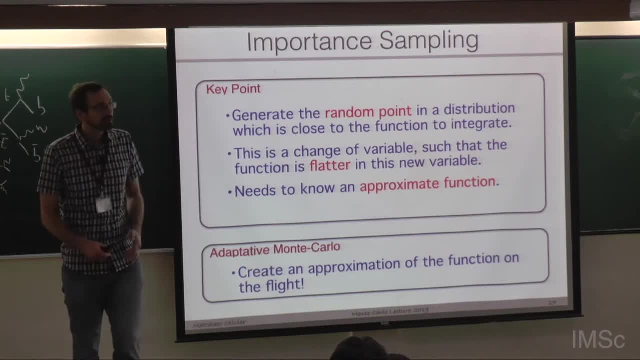 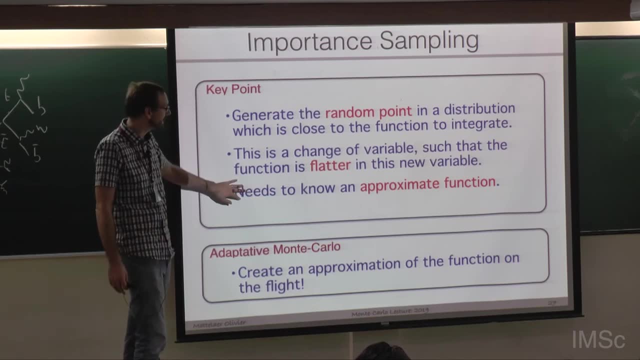 is called adaptive Monte Carlo, And we'll never know perfectly what is the best approximate of the functions. We need to have one, We need to have a good one to start, But what we can do is to improve this approximate by learning the function by machine learning. 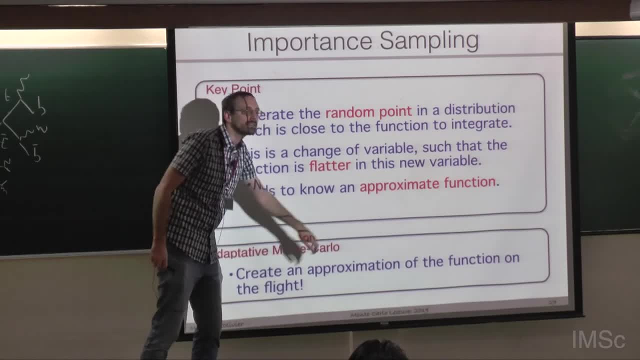 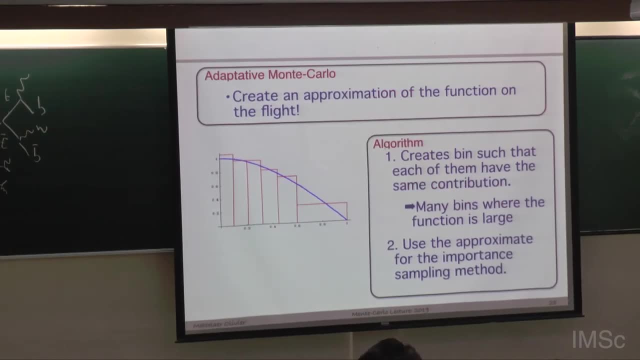 That's a popular word those days- And basically to create an approximate of the functions on the flight. So that's why it's called Vegas And the idea is just going back to one dimensions. first You have your functions, going back to the simple cosine. 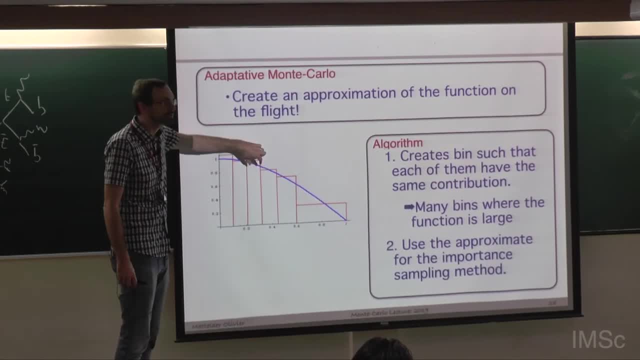 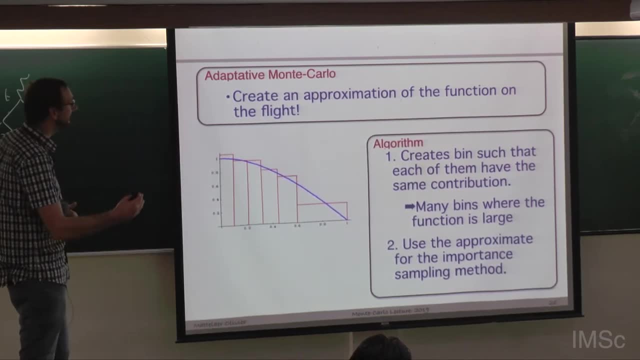 And you can just create bins And you're going to fluctuate the size of those bins so that in each bin you have the same contributions of the integrals. And that's what Vegas is going to do And like that, it's going to know an approximate. 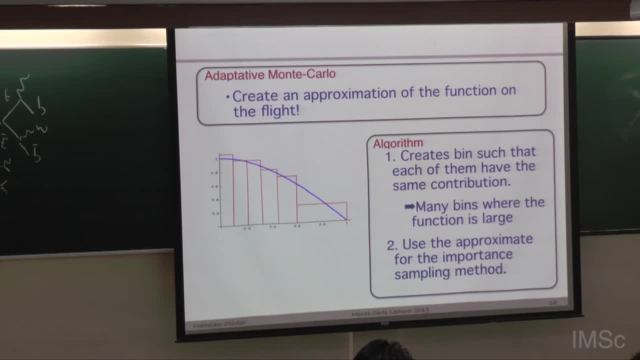 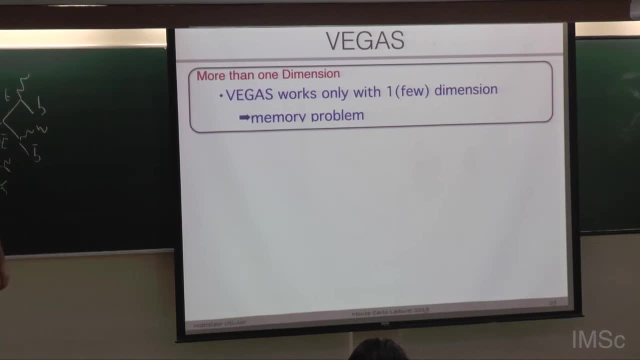 of the integral. It can use it to fasten the face-to-face integrations. That's the basic idea of Vegas. Nowadays, a huge problem in Vegas is the memory. So you need to do those histograms And if you go to n dimensions, the number of squares. 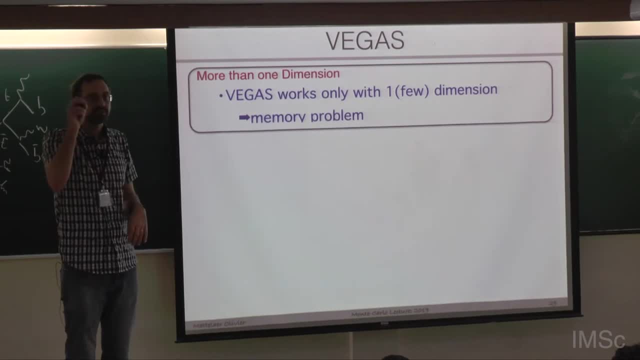 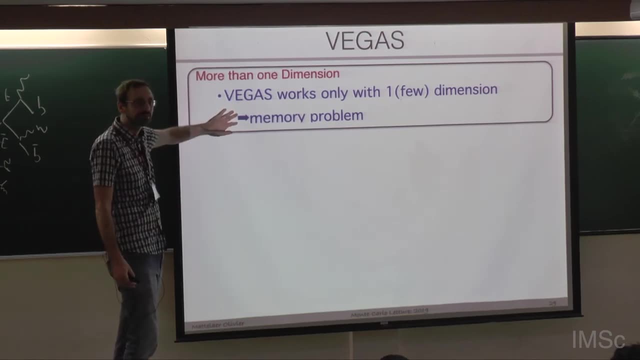 that you need to have is: go like n. Go like n to the power of d. So that's going very, very quickly, Very quickly. we don't have enough memory to store all those numbers. Also, it means that you need to have enough evaluations. 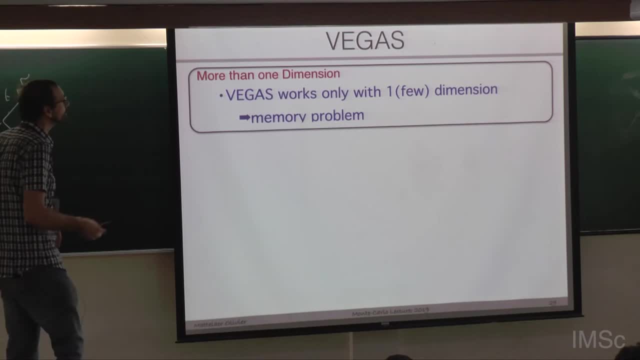 to probe all those histograms in nd. So that's also a problem. So the solution to this problem is saying: OK, I'm going to use projections on each axis, So I'm going to use the trick of the histograms, But I'm going to project my full functions. 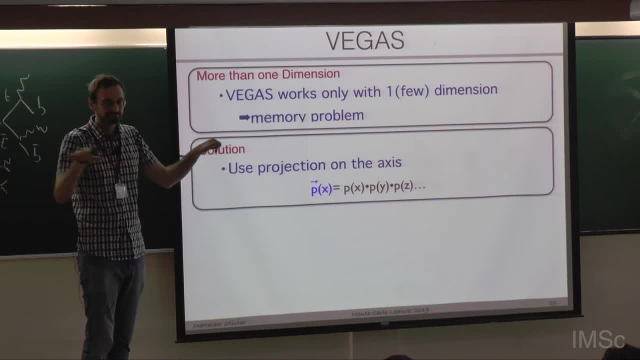 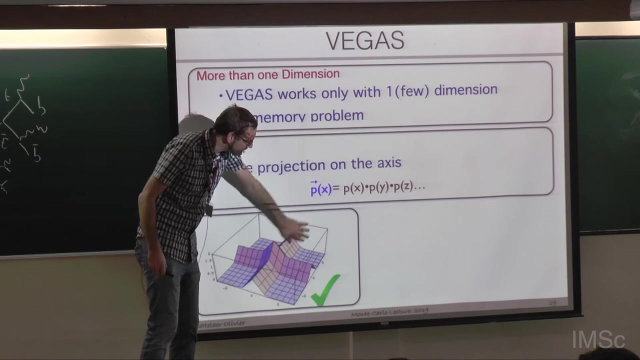 only in one dimensions. And now I have n dimensions And on each of those dimensions I'm probing one histogram, But then I'm losing all correlations due to that. So if my functions looks like this, so it's as: px. align with the axis. 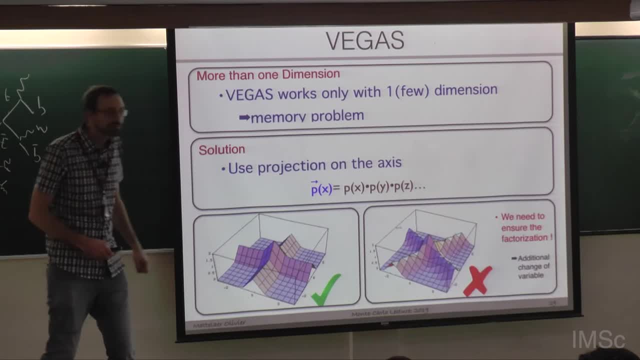 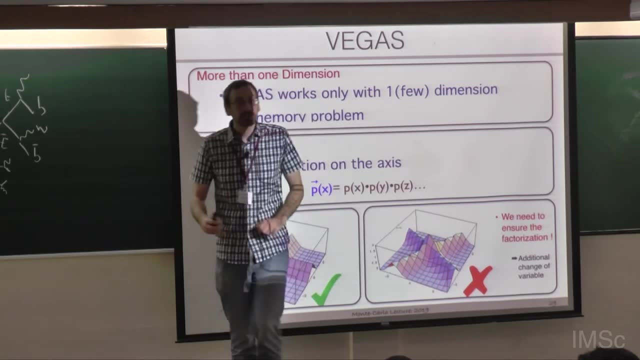 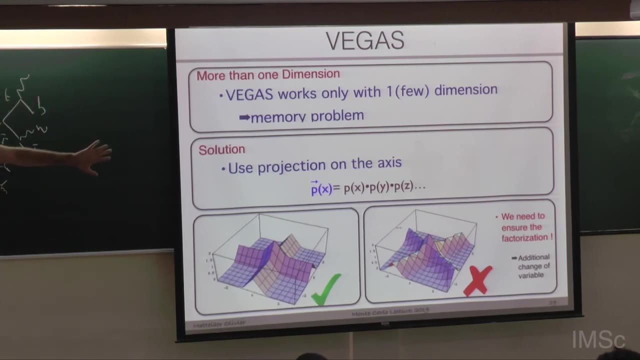 these approximations work very, very well. Now, if I have this- since I actually have strong correlations between my x and y variables, but not expressed. but it's a rotation- technically this Vegas will fail completely, And that's another level of optimizations. 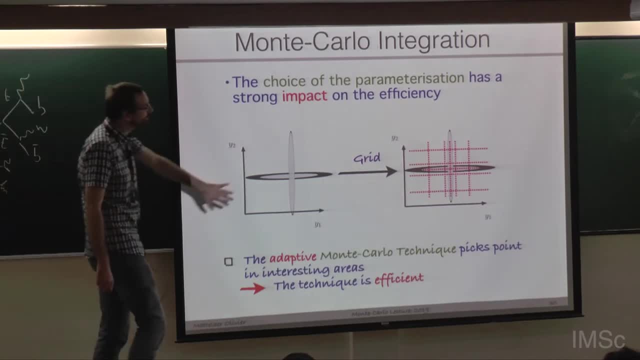 And that's how I'm going to do this. I'm saying the same now in different plots. Now, if you look from the top, this is where the function is big, All the white spots where the function is close to zero- What you're going to see- how Vegas converge in this case. 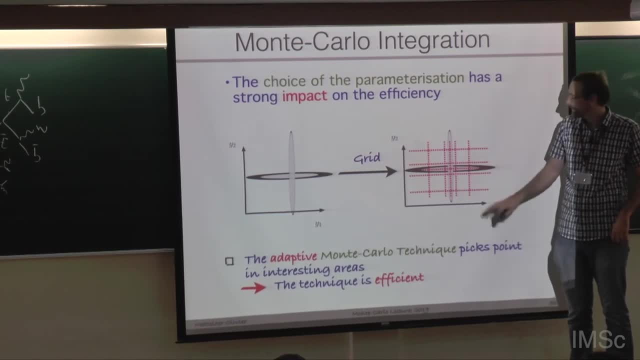 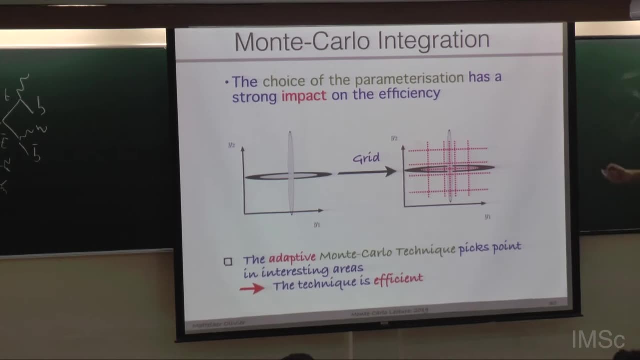 is going really to have a lot of bins where the function is high and a very small number of bins where the function is small, So that will be really optimal. You will learn this automatically Now. if you have this, it's very difficult. 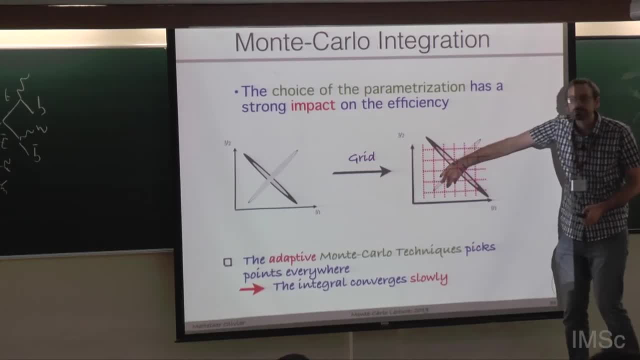 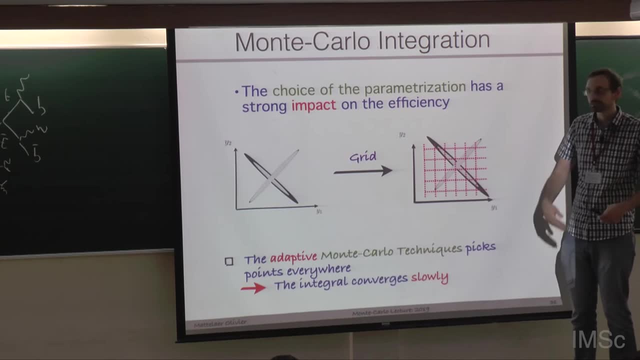 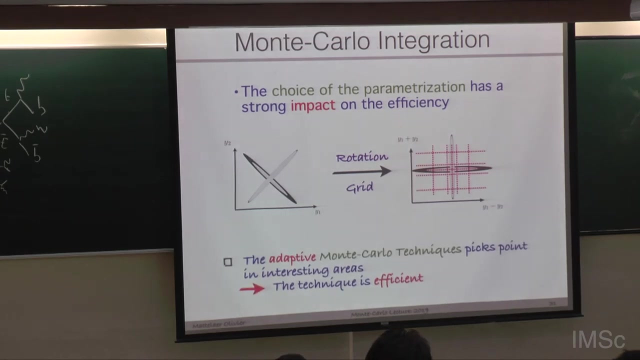 to write to change the size of the histograms here to have a nice convergence. So you're going to probe a lot of times here And that's why your conversion will be slow. So the solution obviously is to make rotations. That means again you need to know in advance. 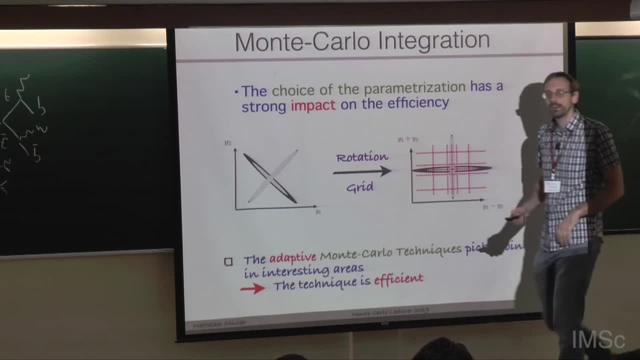 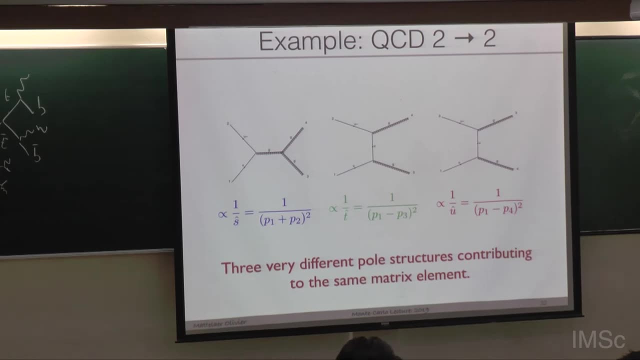 what is your function? And that's also stuff, of course, that we do in MadGraph. Let's go a bit more specific to particle physics now, Because up to now I could have given the same tool to chemistry or whatever I want. 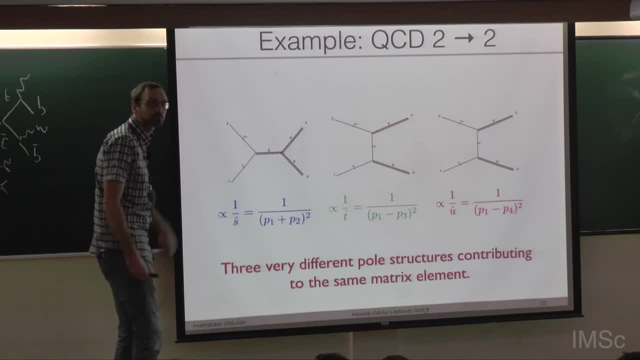 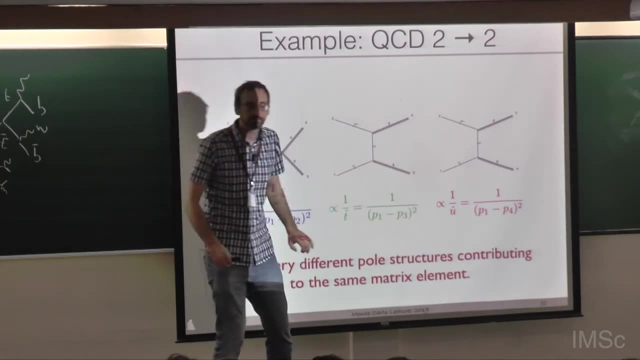 So now, if I'm looking at my frame and diagrams here- a simple to process QCD- you see that they have different peaks. One is the S channel, one is the T channel and one is the U channel. So I have a lot of different peaks. 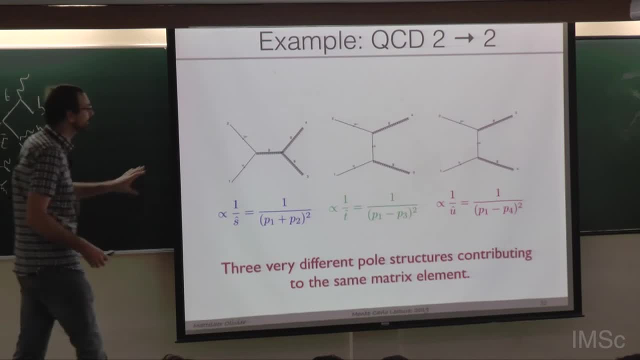 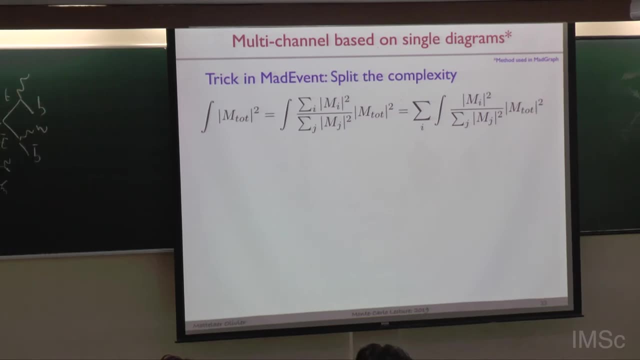 I need to do these approximations And it's very difficult because I have so many frame and diagrams. So we use the tricks implemented a long time ago by Fabio, which is called important sampling. What is the exact name, Fabio? 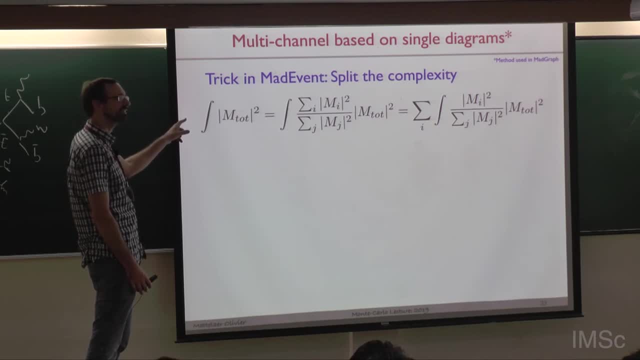 I don't remember of this Single-diagram enhancement. FABRIO DOPINO- Yes, thanks, I was looking last time for it, So it's single-diagram enhancement. So you multiply and divide by the sum of the amplitude square. 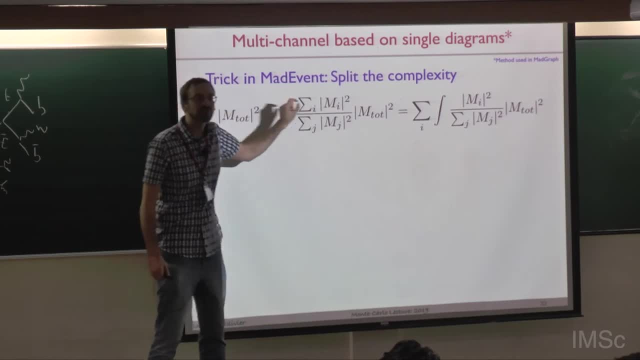 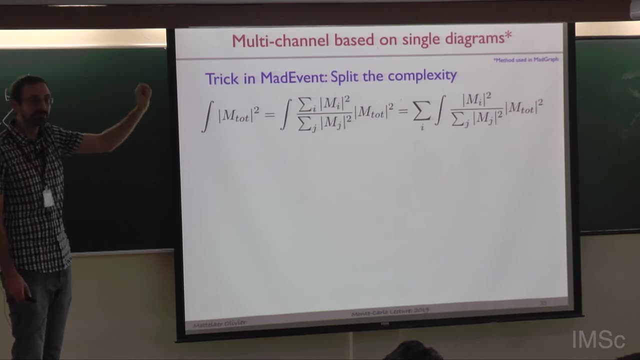 And that's what I said I was looking last time. That's why, here, I need to know each amplitude individually. If you remember, in the valuation of the matrix element I was saying, oh, I will need later each amplitude individually, and that's because of this that I'm doing that. 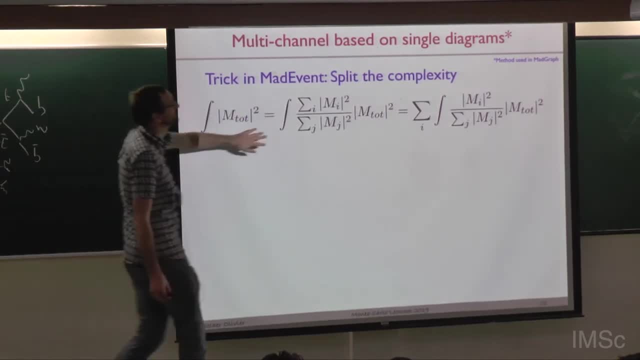 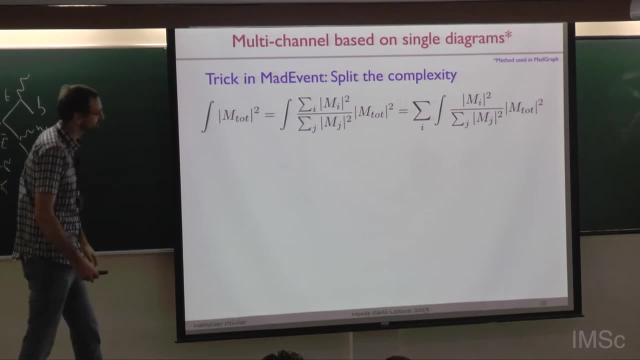 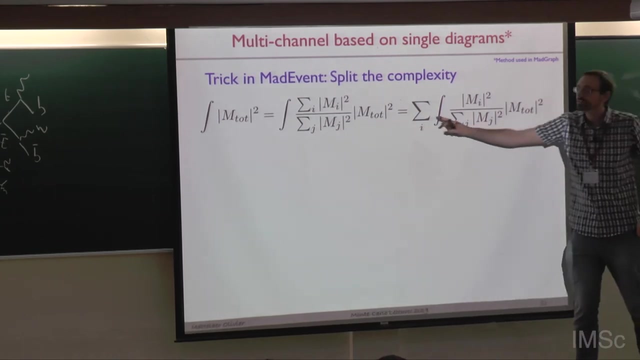 And therefore in the eliciting formula that we use evaluating, these are for free. now The free is not really true, because that means we cannot optimize more, but that's the idea. And now we put this first term here, outside of the integrals, and now we have a sum of 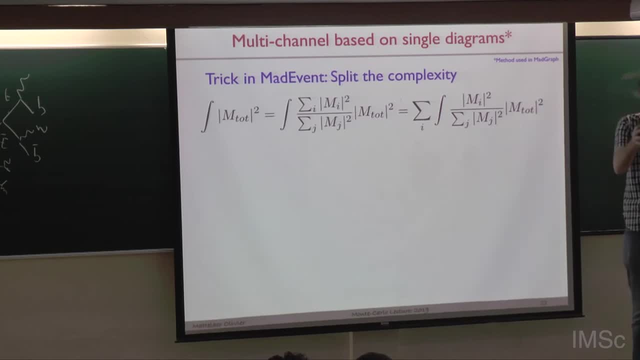 different integrals to evaluate. So we pass from one big integral that was very difficult to integrate to a bunch of different integrals to integrate. And what is So? the interference terms are not in the summation. Yeah, not in the summation, correct, correct? 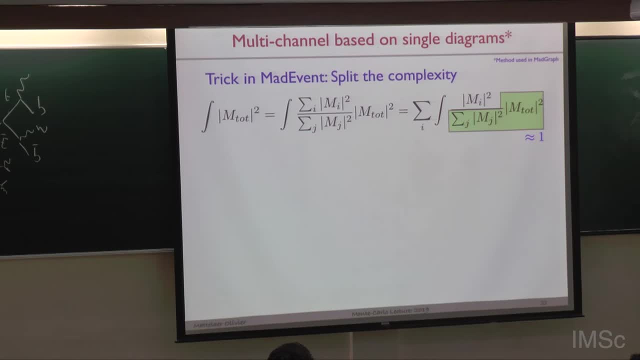 So that's a crucial point. I'll come back in two seconds on it. So now it is actually. it's basically now. So this ratio here is basically one. The only difference between the numerator and the denominator is actually the presence of interference in the numerator and the absence of interference here. 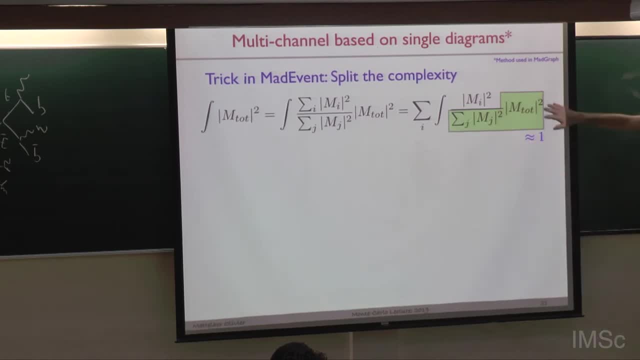 So that's the only difference. So this is basically one. as long as the interference is negligible- And that's the huge assumption that Margraf is going to do for the phase-based integrations- is that interference is negligible In most of the cases, it's correct. 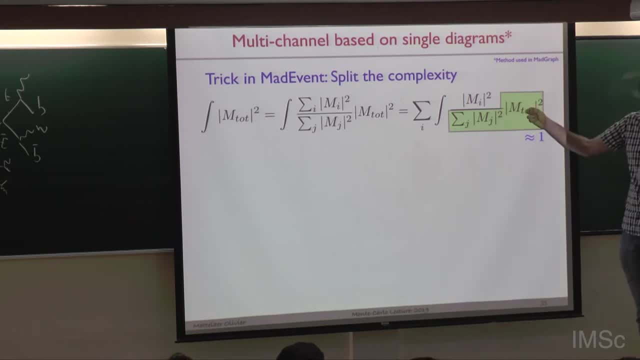 Of course, in some cases Some people want to integrate here interference-only terms and that is a nightmare for me because I don't know how to do the phase-based integration. We are still using that, the exact techniques, but it's really on the 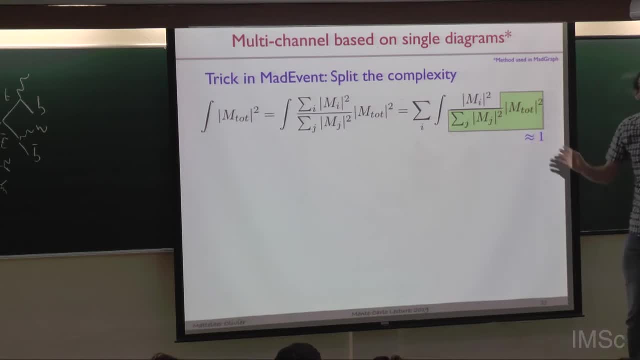 Not on solid ground anymore, because the assumption here interference should be neglected, I mean can be neglected Of course. you see, and I want to stress that this formula is exact, I'm still My integrals is still the full integral with the interference. 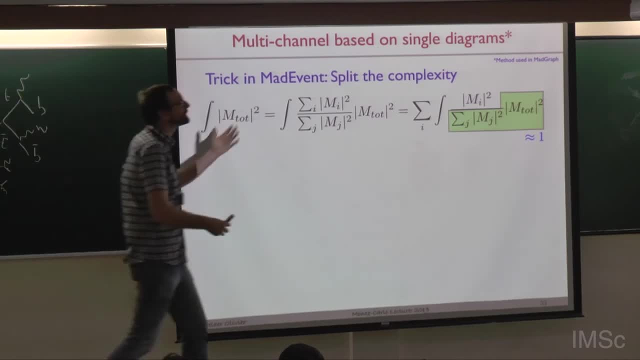 So Margraf doesn't neglect interference itself. Is this for the optimization's point of view, if we want to integrate that in an efficient way, assuming small interference. If the interference is big, that means my optimizations will be bad, my code will go. 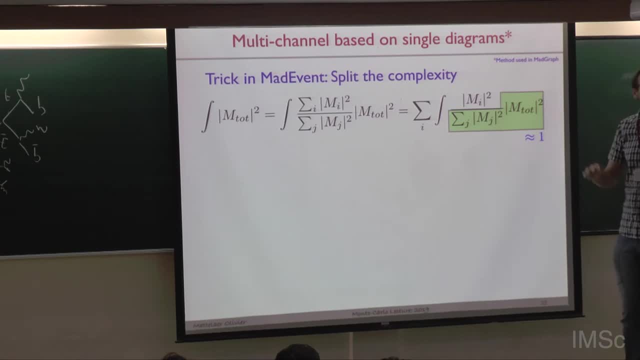 slower and worst case scenario we can have bias or wrong result in very, very case, basically where you have on interference here. So this is really nice because now I'm integrating only one single diagram at a time. What happens? Is this good? 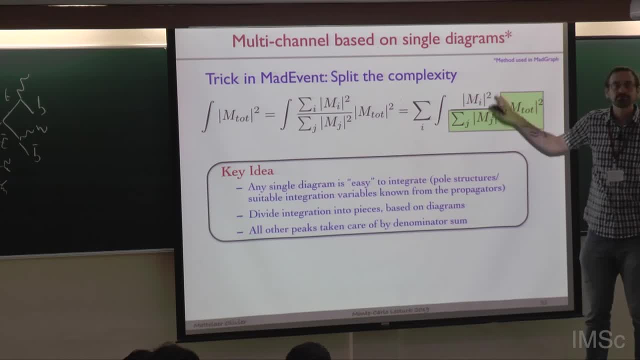 Is this good? actually, I have n integrals corresponding to my n Feynman diagrams, and if I have one single Feynman diagram, I can do all those rotations, all those important samplings, because I know exactly what is the propagator for that Feynman diagram. 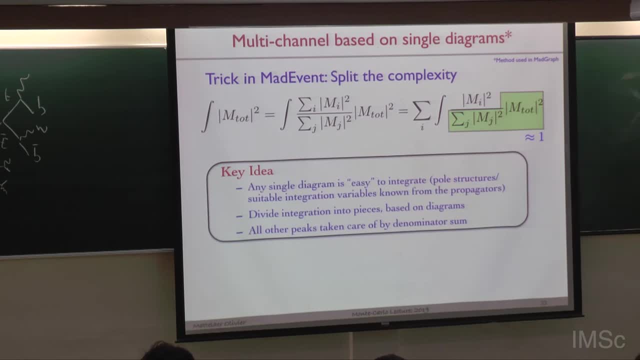 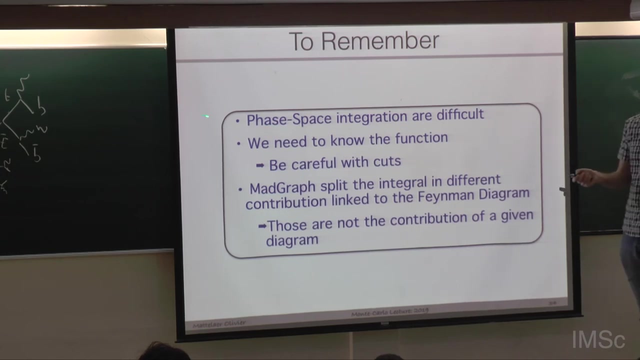 I know exactly how everything behaves. The second interesting point here is that I've basically split my program, my problem, in a lot of small problems, So I can now basically send that on a cluster and I've basically paralyzed my computations. Okay, so what is to remember for this part? that phase space integrations are difficult. 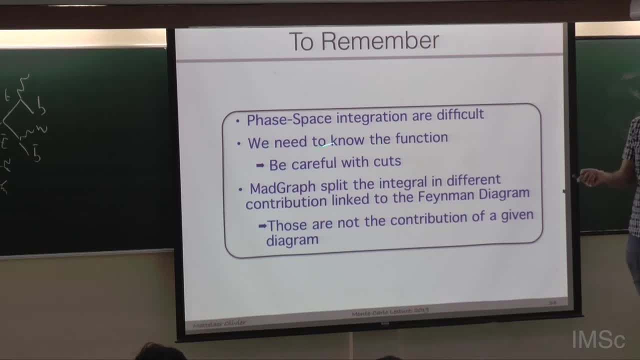 You need to know the functions you integrate in advance and therefore you need to be careful with the cuts. I always prefer cuts that are provided within my graph than cuts that you will outcode yourself. Sometimes you don't have a choice, And then okay we, we split the computations. 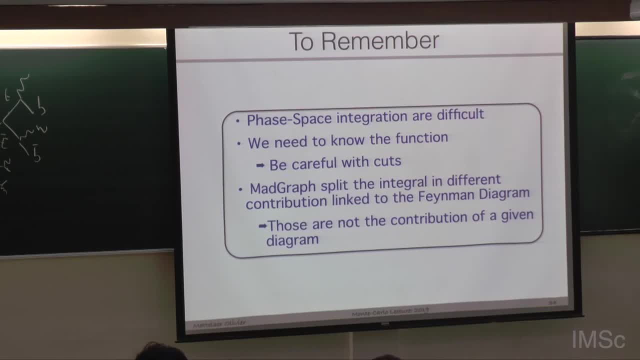 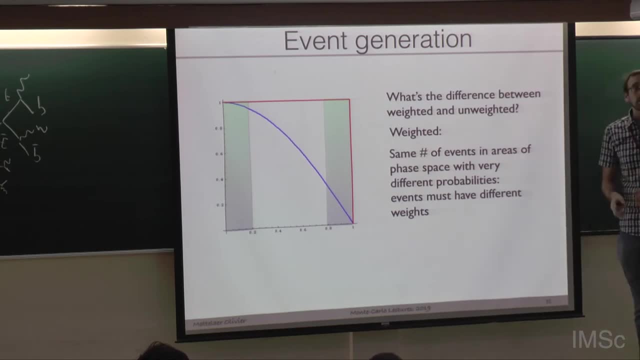 in a lot of smaller parts, okay. So now, maybe the most important part I would say is: so far I've concentrated myself on how to compute that integral, how to compute the cross-sections. What we really want is actually how to generate events. 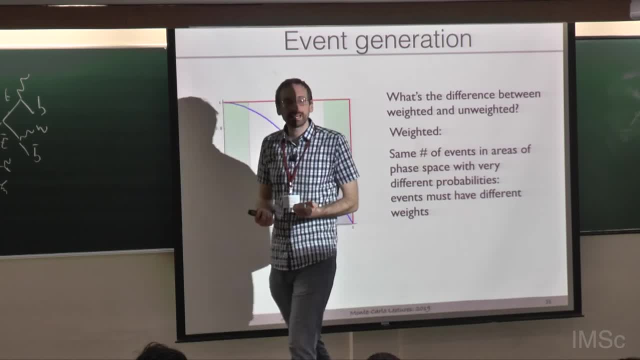 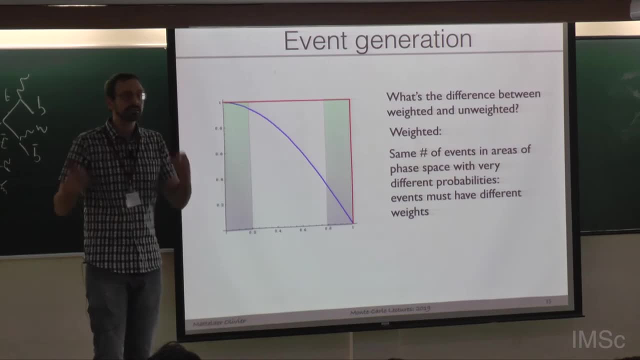 And what is nice in itself in the Monte Carlo method is that actually I'm probing randomly, So I have no correlations between my events. I can simply use those as representative of my computations. So I'm already generating a lot of events here and I have no correlation between my events. 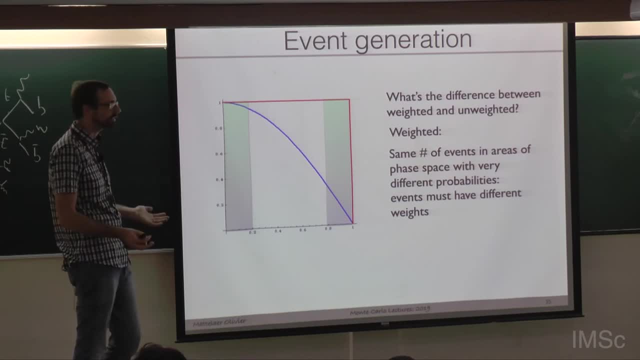 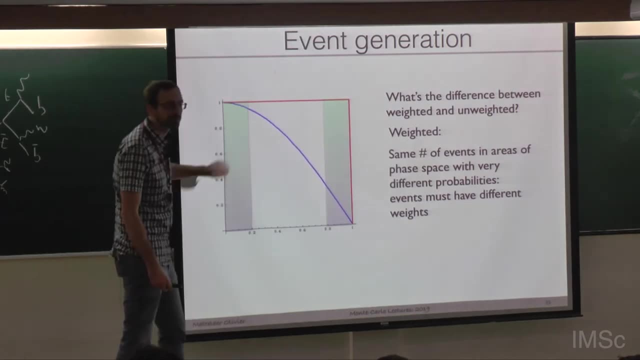 so, in principle, I can use them, because everything is random. at the end of the day, The issue is, of course- so let's assume that I'm not using important sampling first- What I'm going to do, since it's random sampling. 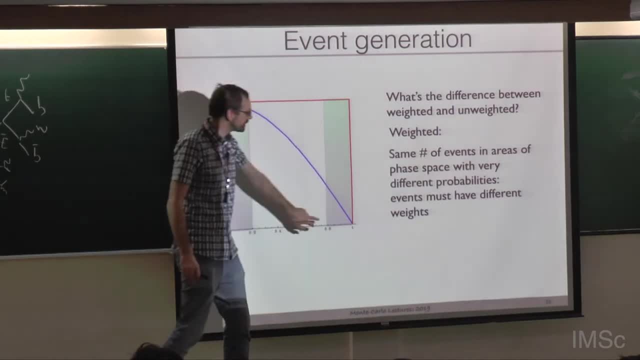 I will have as many events between zero and zero dot two as the number of events between zero dot eight and one. That's why random. That's why random is. You don't have any preferred directions And of course, that's not what you want. 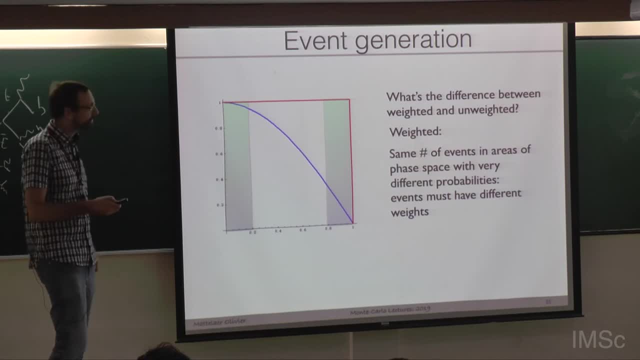 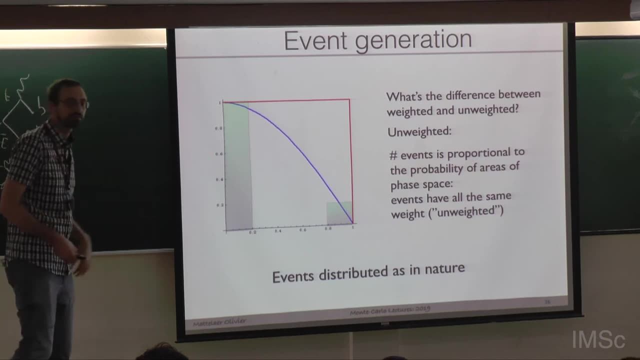 You want to have your events distributed like nature, which means you want to have less event in the last bins compared to the first bin, Around a factor of five. but I'm not sure that's the ratio on the plot. I'm not sure it's exactly correct. 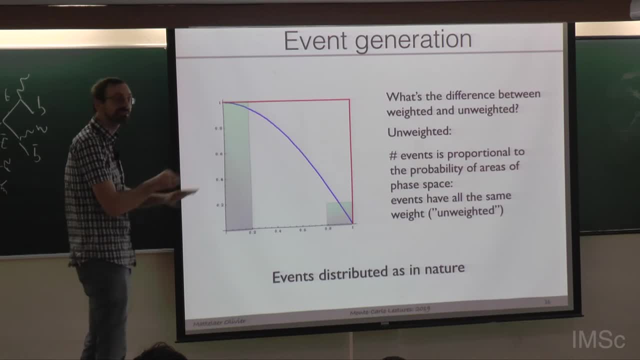 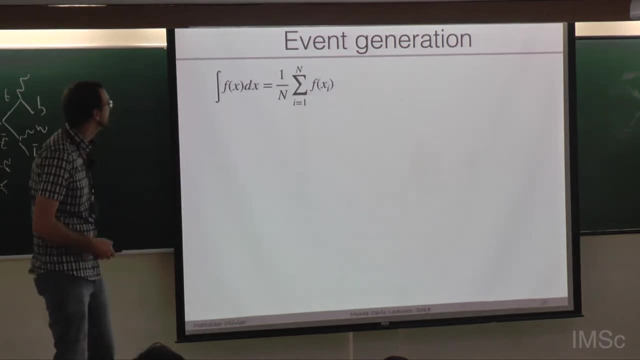 So that's what you want. You have the number of in each bin in any observable that you can construct, to be proportional, finally, to the functions that you are integrating. So that's the idea, So all we are going to do, we are going back to the formula. 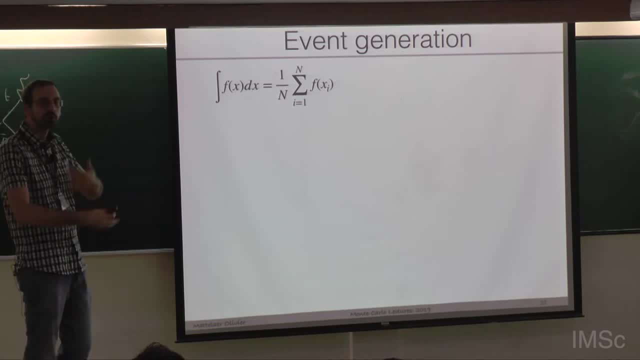 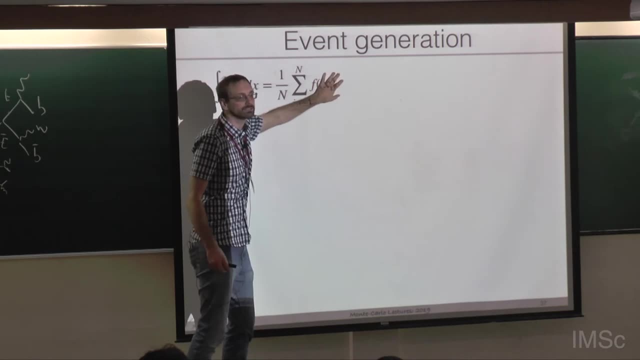 here. I'm going to do it quite theoretically first and then give more of a feeling about what it's doing. So my integral: I rewrite it as a random sum, So I have n random number and I'm taking the average. 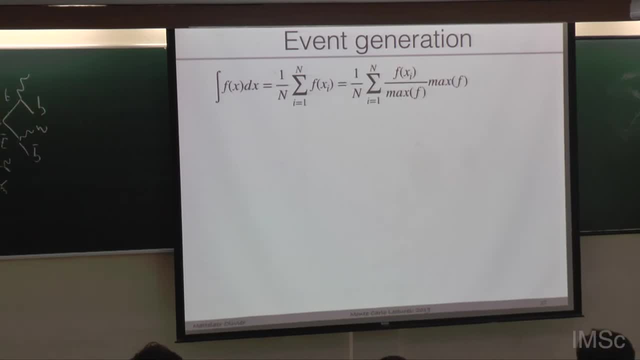 That's what Monte Carlo is. So now what I'm going to do? I'm going to multiply and divide by the maximum of the functions. So this is a strong example. It's a strong assumption in itself. It's meaning that your functions are the maximum. 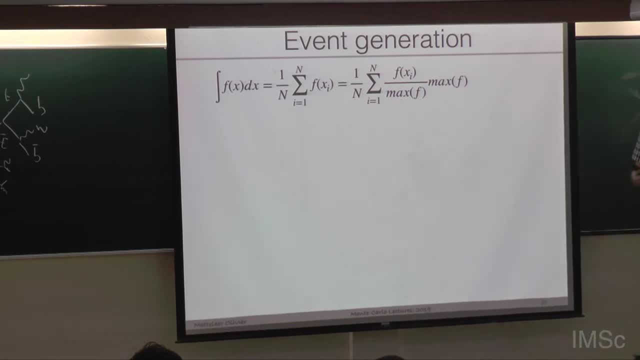 So you need to have cuts in your functions. Your functions need to be regulated. If you have things like soft collinear divergency or if your matrix analysis is not defined everywhere in your phase space, you need to have a cut so that this maximum exists. 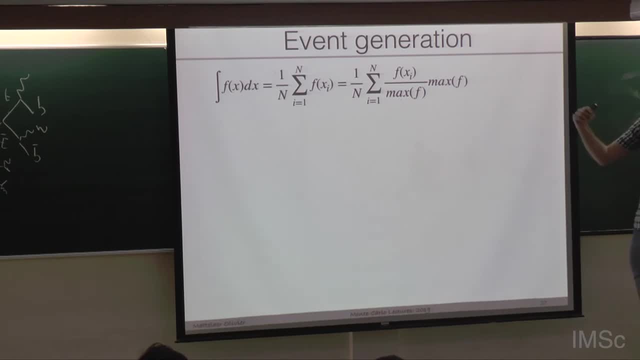 Typically, if you have e plus e minus, e plus e minus, if you go to a small energy, you will have a divergency. That's something that will prevent the function. OK, The functions will have a maximum. So that's something you have to put a cut. 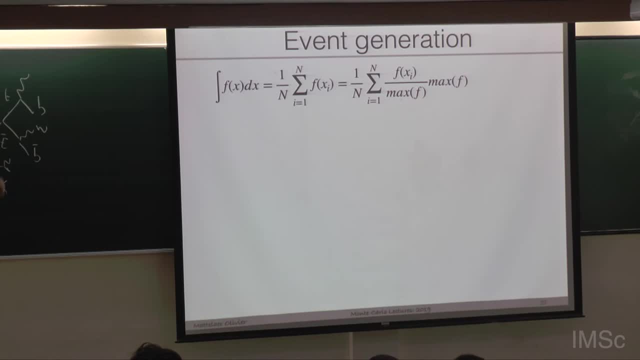 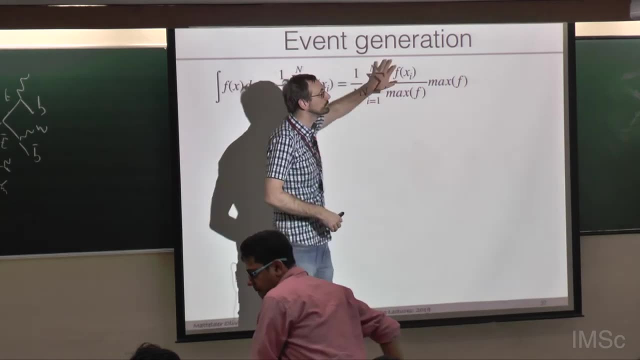 So in MathGraph if you have a matrix element that diverges and you try to do the phase space integrations, the maximum will be updated Every time we update the maximum and you will fail to have enough events and it will take a lot of time to reach that. 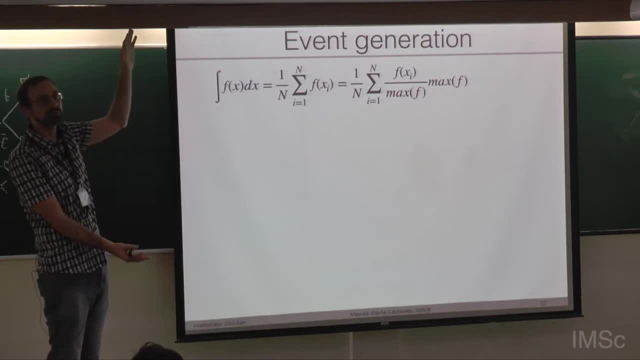 And again they will say these microsections, typically with a huge error because your matrix will diverge. And typically you will say: I generate one, sometimes two, sometimes three events And that's a sign that your matrix will diverge. 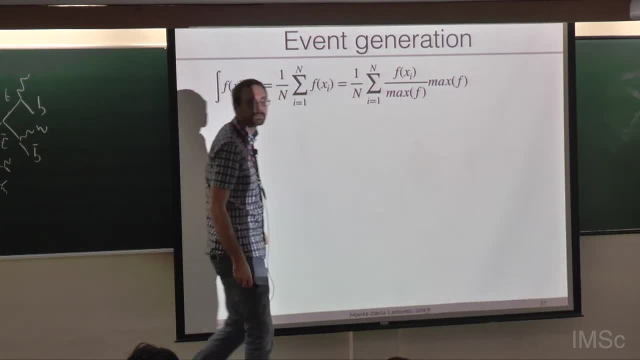 and that MathGraph fails to find the correct maximum here because there is no maximum. So, OK, I've multiplied and divided by a maximum And now I'm going to reinterpret this as a probability. So that's a ratio between a number. 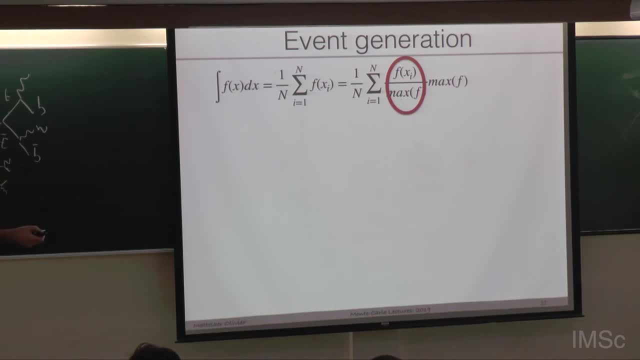 And this ratio will always be, at the end of the day, between 0 and 1.. That's actually a second assumption here. Why between 0 and 1?? That's assuming that f is always positive, which is true at leading order. 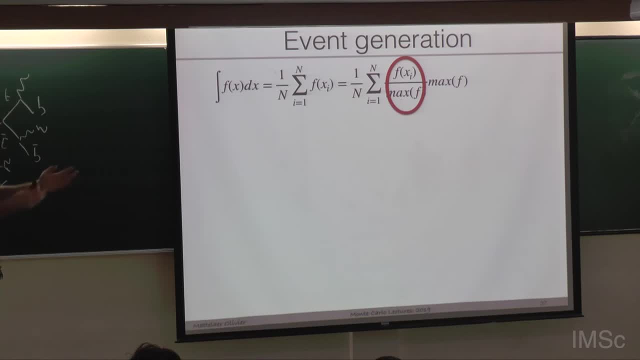 So we'll see, We'll stay with that. today, If you go to NLO, that is not true anymore. That number will be between minus 1 and 1.. But OK, So here I'm assuming between 0 and 1.. 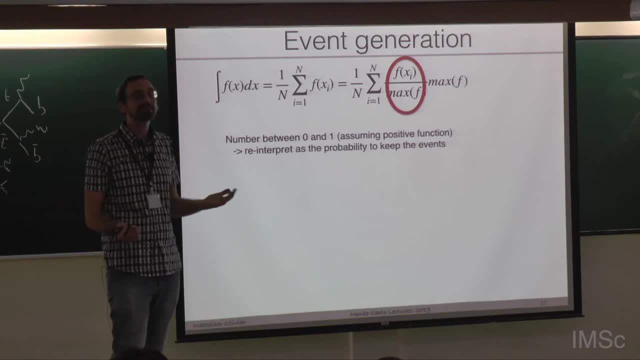 And then I'm going to reinterpret this as a probability to keep or reject my events, Saying actually I can reduce my sum and reject a lot of events. I said in those last bins I was probing too much often. I was probing very, very often. 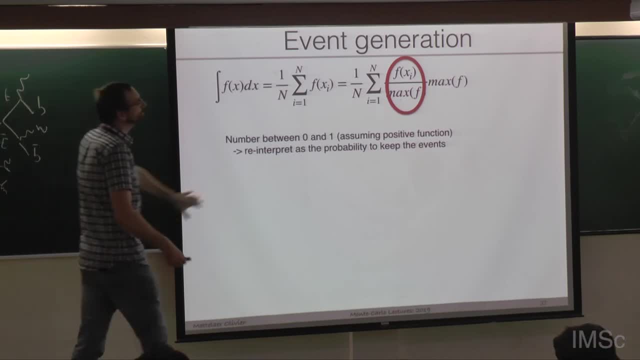 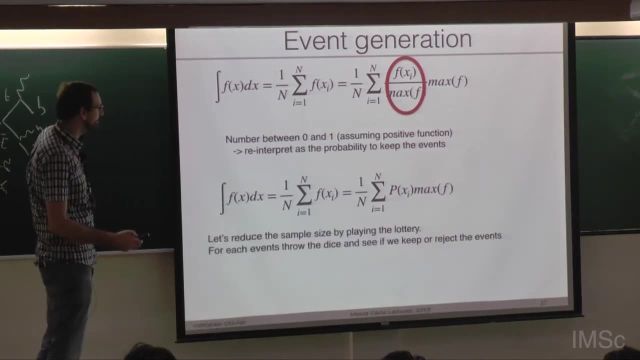 So that's bad. I want to have less events there and I'm going to use that as a probability to accept or reject my events, And when I'm doing that, I'm going to now probing the lottery. reduce my sample size. 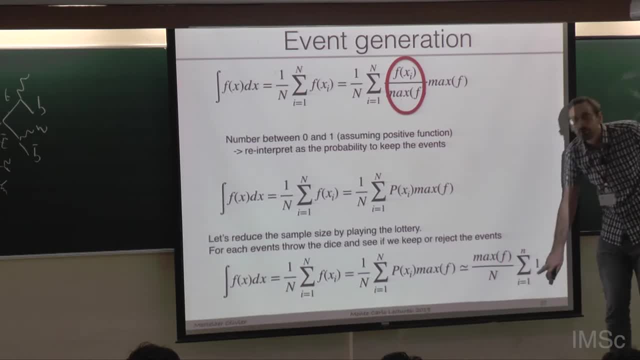 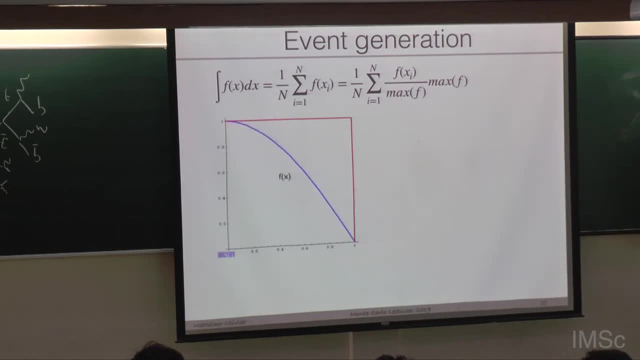 So I will have much less events at the end, But they will all have now the same probability at the end. So that's why I call it unweighted events, So to show exactly the same procedure, but now graphically what I'm going to do randomly, I'm picking a point. 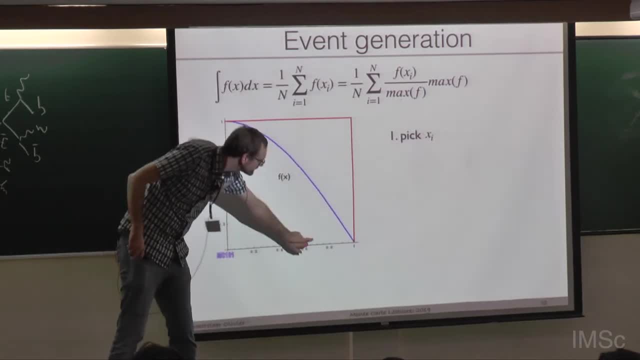 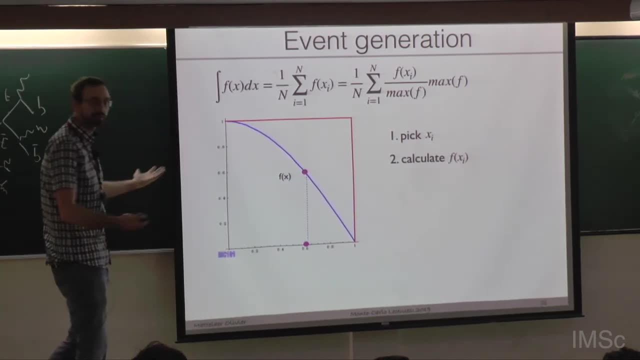 That's my Monte Carlo procedures. I'm taking random points. In this case, I'm taking 0.6.. I'm going to evaluate my functions, what I need to do anyway to make my phase space integrals, And then I'm going to throw a random number, in this case, 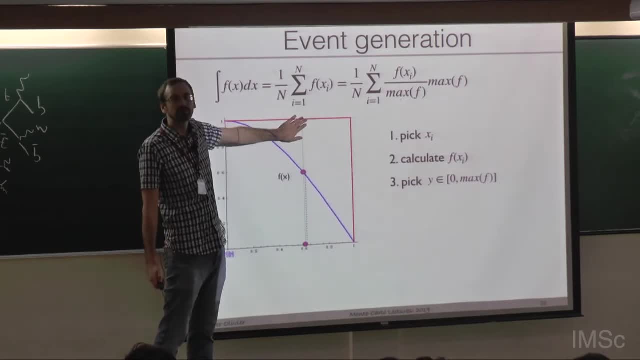 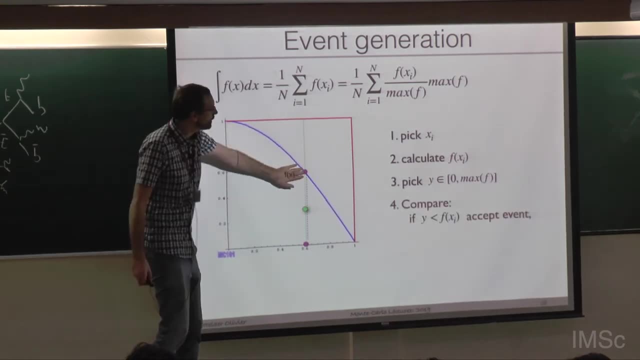 I call it y between 0 and the maximum of my functions. So in this case maximum is 1.. So it's very simple, And either my random number will go below the curves. In that case I will keep the events. 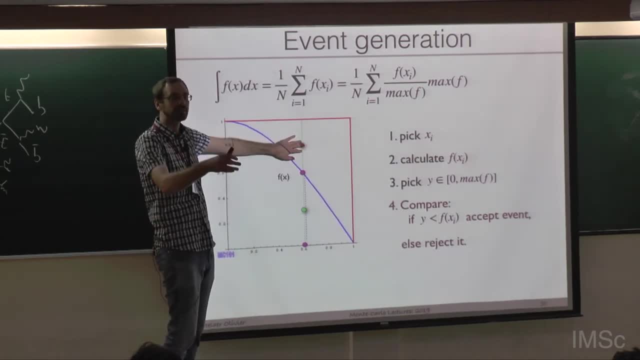 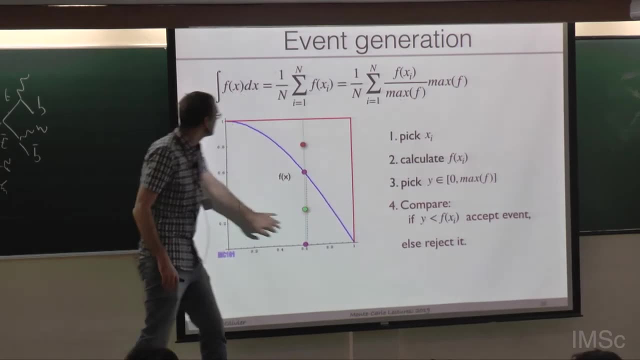 Or it will go above the curve. In that case, I reject the events. And that's allowed me to say that if my function is small, I'm going to reject most of my events. If the function is high, I'm going to keep most of my events. 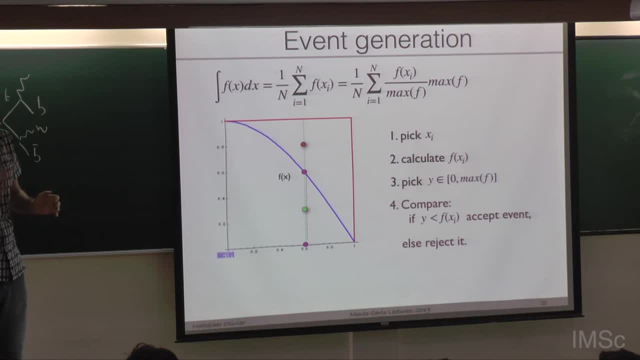 It's exactly the idea of I want to, at the end, my distribution shape exactly like my distributions, But I don't need to have any binning or anything. So that will be true for any observables that you can do, You can build. 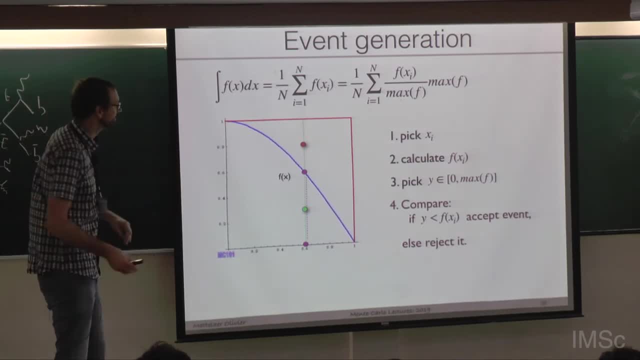 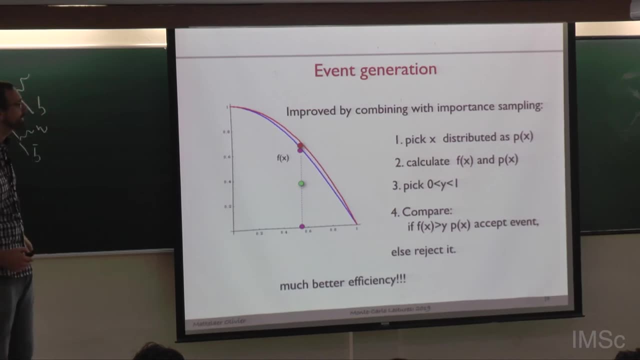 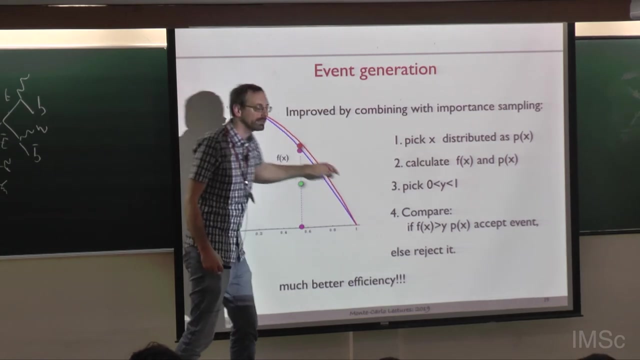 So it's not using ttbar, pt or whatever. It's really any observables in that procedure will work. So now, if I'm going back to important sampling, what it does basically is now that, instead of probing the function is a flat way, I have probing my functions. 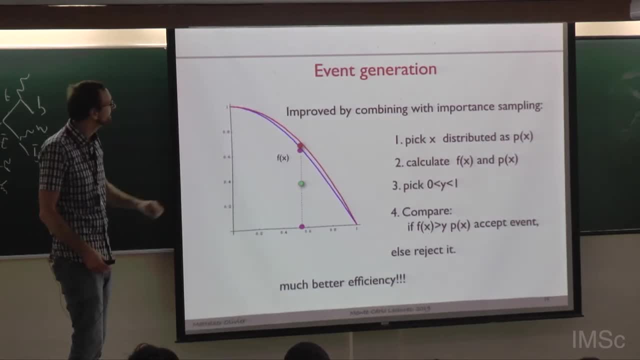 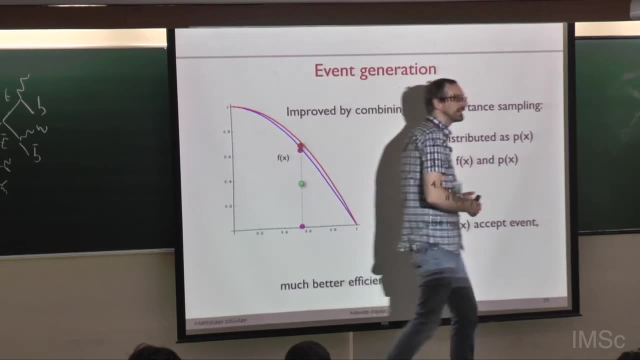 in a slightly different way, which is very close to my functions itself, And therefore the efficiency of unwitting is much higher. So it's basically the same idea actually in both, And that just means important sampling than before. That's just faster on your code. 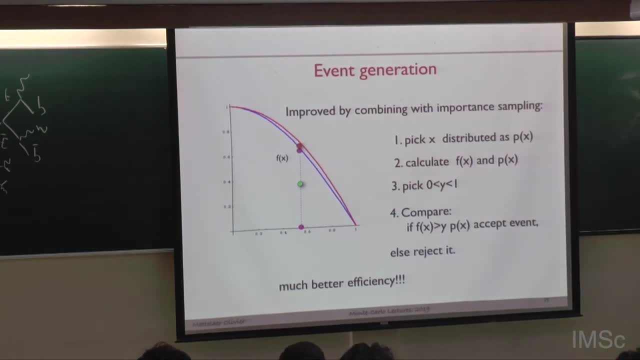 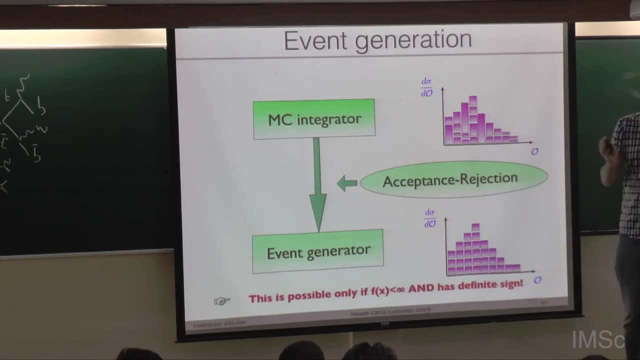 It's much faster to the 10,000 events, But the same idea all basically. So one key difference between normal weighted events and unwitted events is how you feel: histograms In principle for each event, and weighted, you have different contributions, which is the fact. 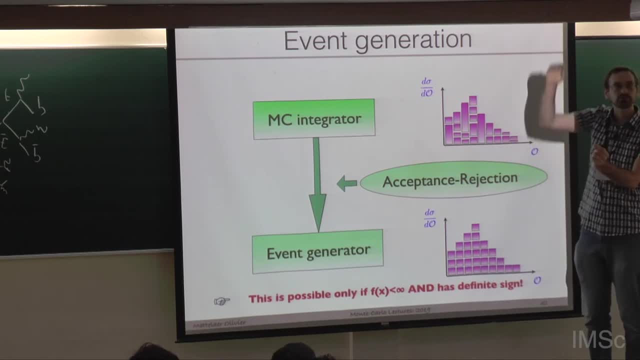 that, oh, I'm probing a place where my function is high or my function is small After an waiting. you always enter one in your histograms whatever events you get, And one key importance between those two is that, in this case, your histograms typically. 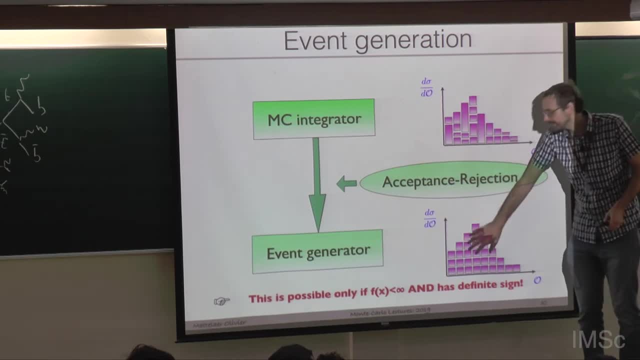 have millions of events and for the same accuracy here you only have 10,000 if events And that's crucial if you want to pass those events to pattern shower and, even more important, at the end to event reconstructions. Doing the full event reconstruction in CMS and ATLAS. per event takes around one and two. 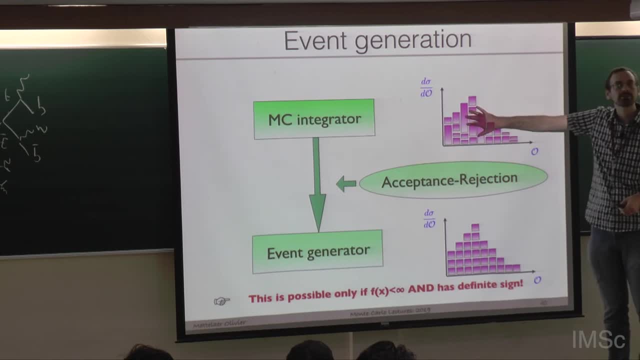 minutes, So it's extremely slow. So if you need to do that for one million events with a lot of events, which contributes very, very small in your total cross-sections, it's a huge waste of CPU time And actually now already CMS and ATLAS, we don't have enough CPU time to do these. 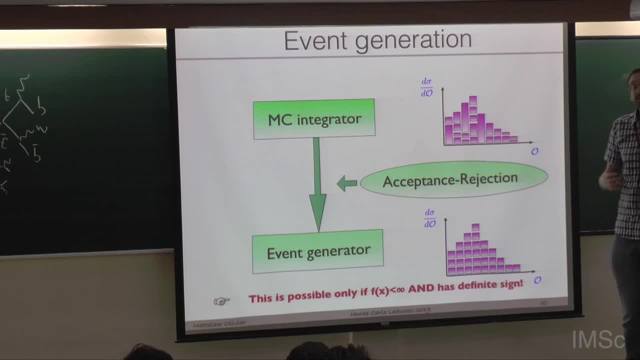 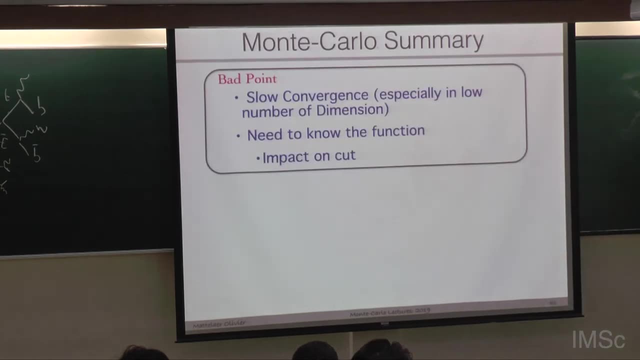 full reconstructions most of the time, So they are a really limiting factor. So going from there to here is really important for them, obviously OK. so the summary, The bad point of Monte Carlo, and I stress that enough. I guess it's extremely slow. 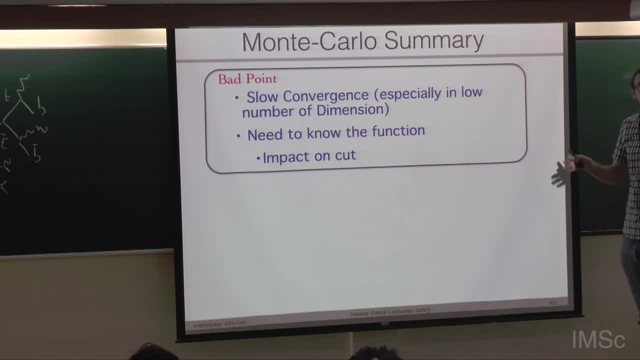 It's the best solution, obviously, but it's still extremely slow. You need to probe your functions a lot, a lot, a lot of times And, in order to have it faster, we need to know the functions in advance, which is a 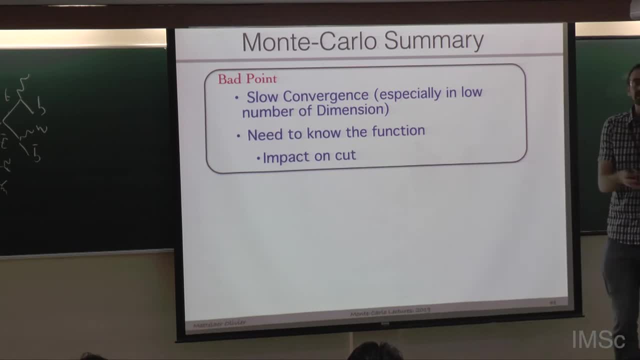 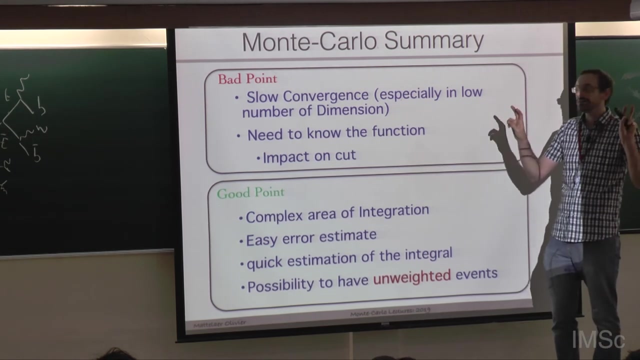 bit counterintuitive. If I know the functions and the primitive in advance, I'm much faster, but that's actually what it is. We need to know all the knowledge that we have in order to have that fast. So the good point is that you can basically implement your cut if they are small enough. 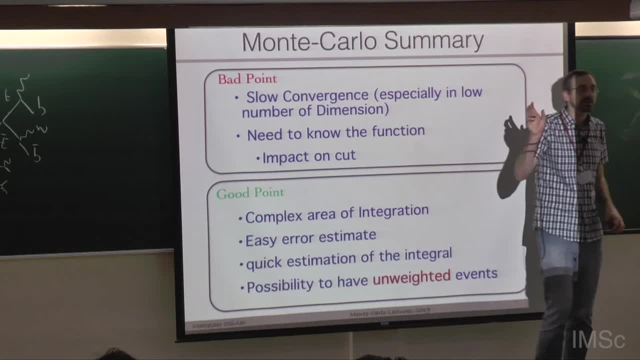 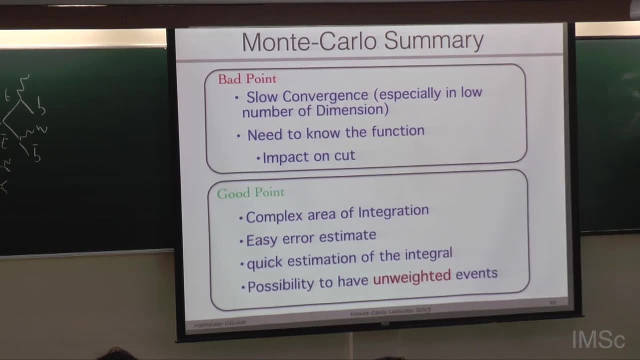 Implementing your cut is quite simple. It's quite simple to estimate the error, because you can estimate the variance as well. And therefore, the last, most important point, the procedure of unweighting, And that's really important for experiments. 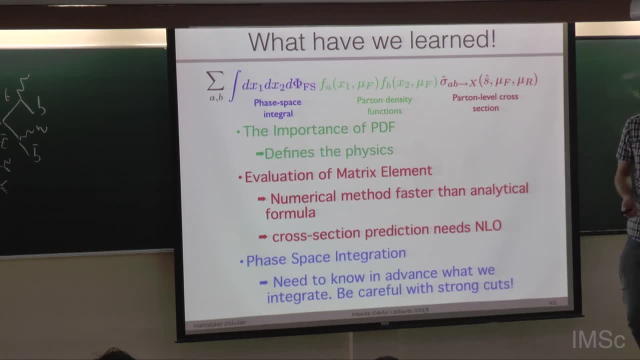 OK, OK. So it's a good time to sum up now what we have done so far. We still have a couple of slides after that. So what we have interested so far is these huge equations. I have stressed the importance of PDF. 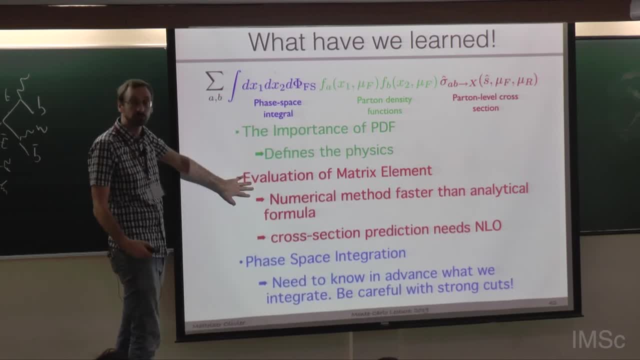 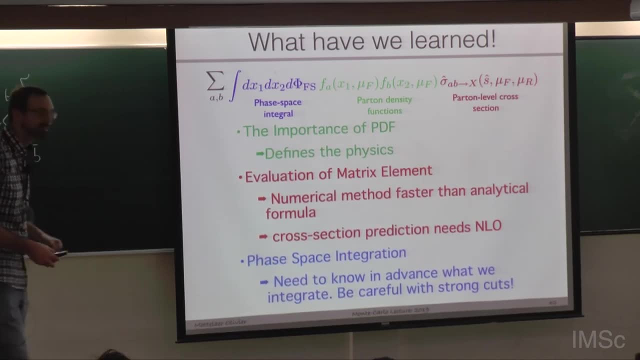 In relation to the matrix element, we do it numerically- It's much faster than ethically- And the phase-phase integrations. we need to know in advance what we're integrating, So it's not a black box when you enter functions and it returns for you the phase-phase out. 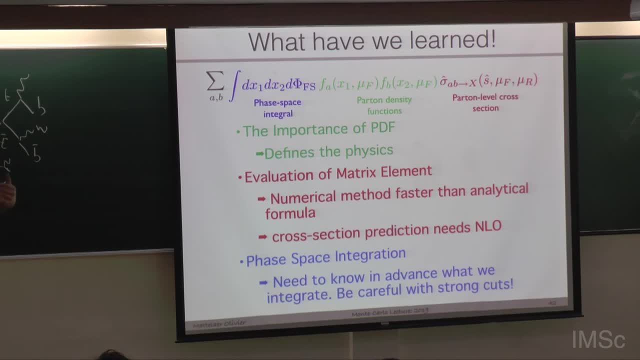 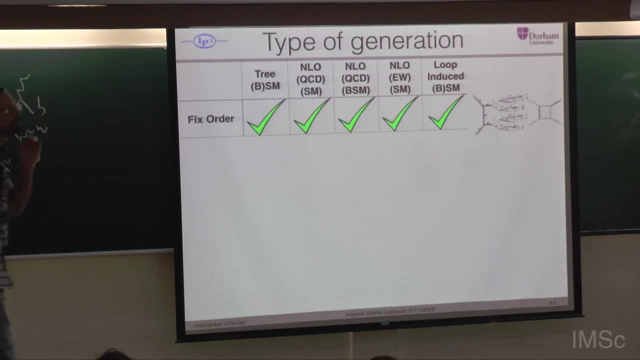 of magic, like a bit like a neural network would do. We need to know in advance what functions you put in, and that's how we get the result. OK, So now I want to go back more on what Milerov can do. 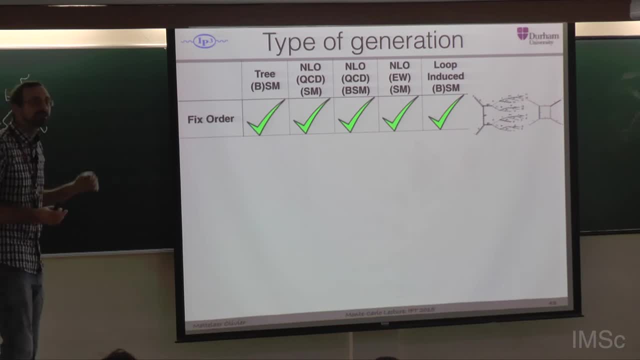 And for that I'm going to describe quickly the different type of physics that Milerov can do, And that's going to be explained more in details tomorrow and after tomorrow, more in details what that means. So the first type of computation is what I have basically done. 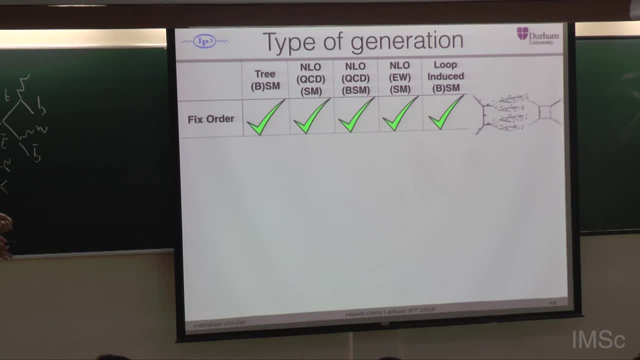 The second type of computation is what I have basically used so far. It's called fixed-order computations. So I'm doing computations at leaning order or next to leaning order without any pattern show at all, And for this, when there is a check mark, that means Milerov is able to do that computations. 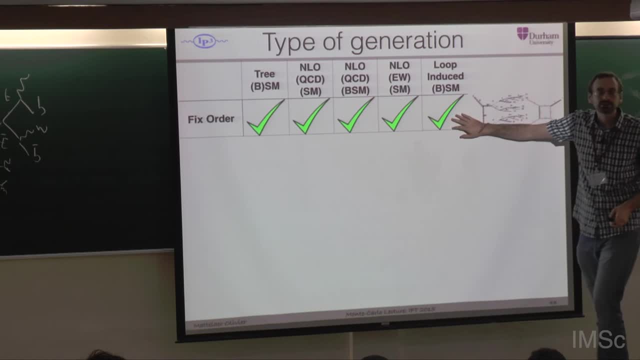 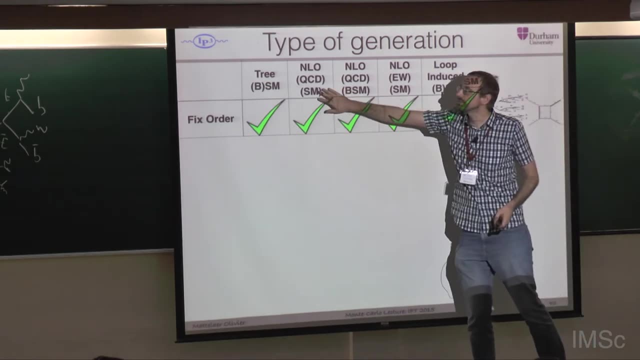 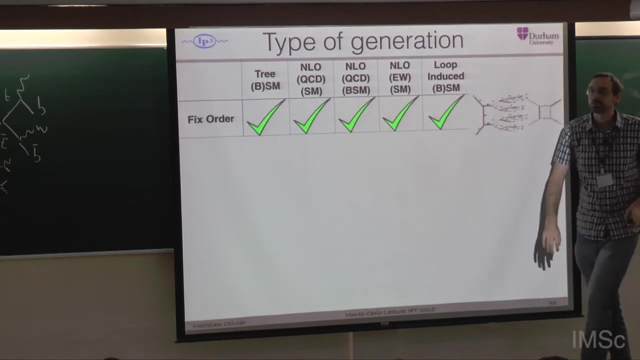 Here at three level. here for loop-induced processes we take three-level leaning order as well, And those want different type of NLO: NLO in QCD in the standard model, NLO in QCD for the BSM physics And NLO in the standard model. 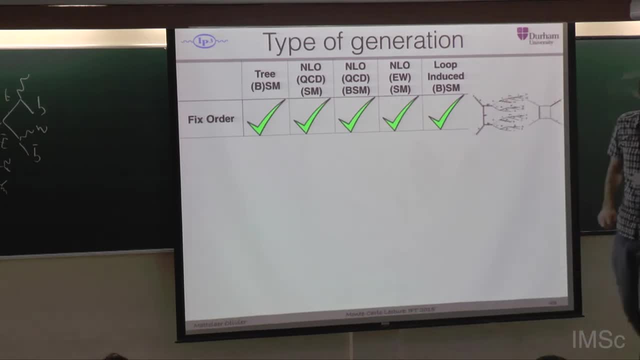 So this is technically still in beta, but it's available, publicly available. So the second computation is to be able to use those events and pass them to the pattern shower. So that means that you need to be able at this first stage to generate unweighted events. 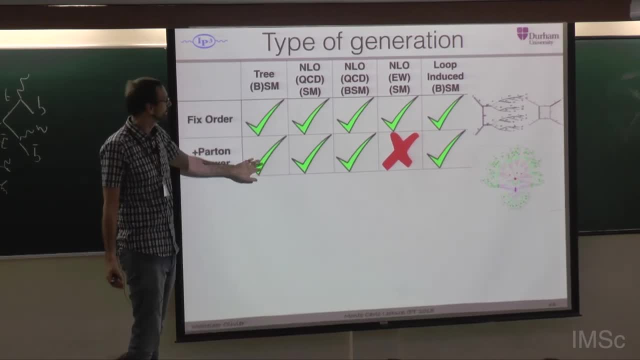 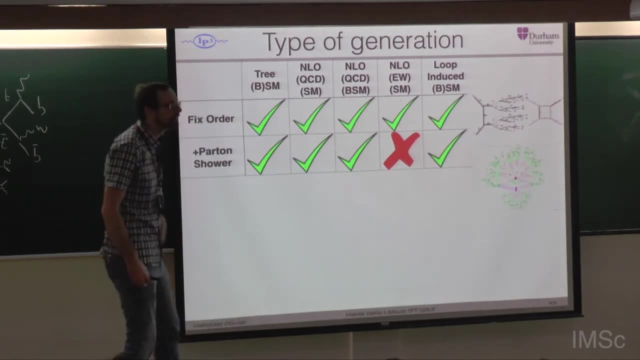 And therefore this check mark is basically what I have discussed five seconds ago. We can also do that at NLO. We can also generate events at NLO, And that could be explained later. We're not going to explain today- And that's much less trivial- how to generate unweighted events at NLO and pass them to. 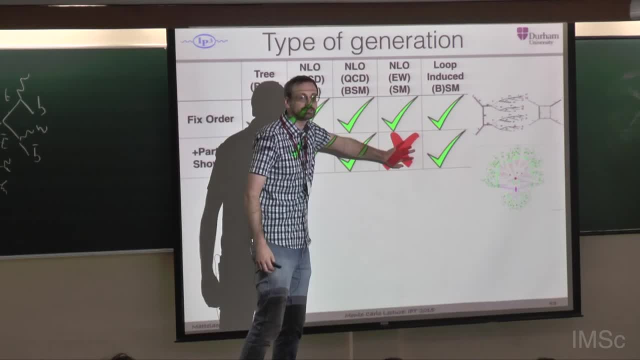 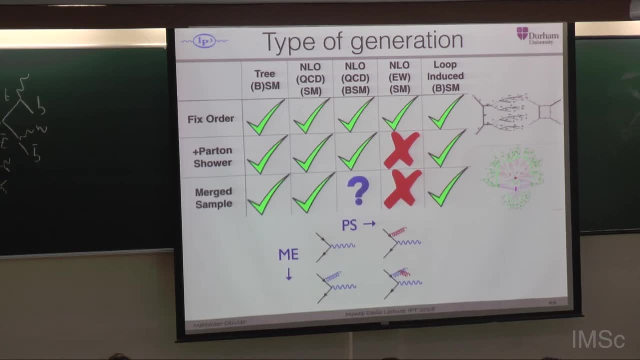 the pattern shower. We cannot do that for the moment at NLO in QED. We have some issue there And the third step- that will also be described tomorrow at the settling order and cover a bit of NLO already- is to have Merge Sample. 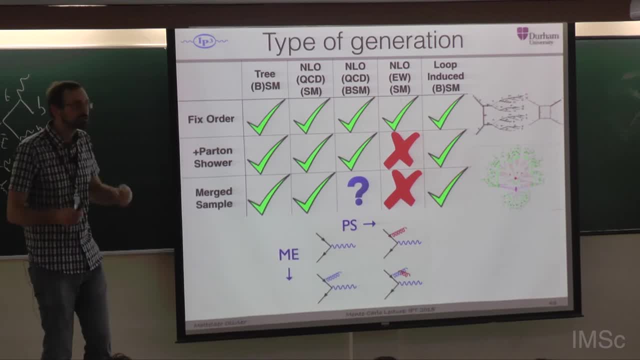 Merge Sample. So if you want to express your jet correctly, you need to have the I multiplicity jet. So you need to have your full matrix element and you need to use Margraph for ttbar plus three jets if you want to observe correctly the three jets in the final state. 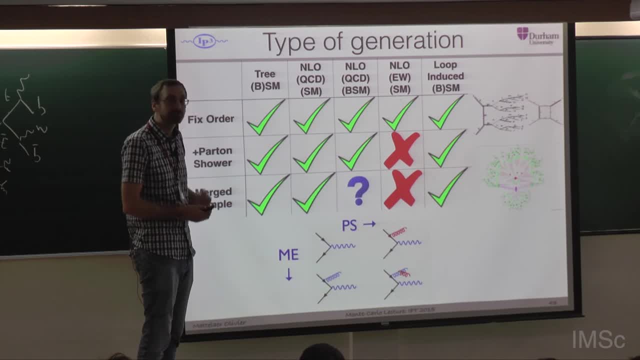 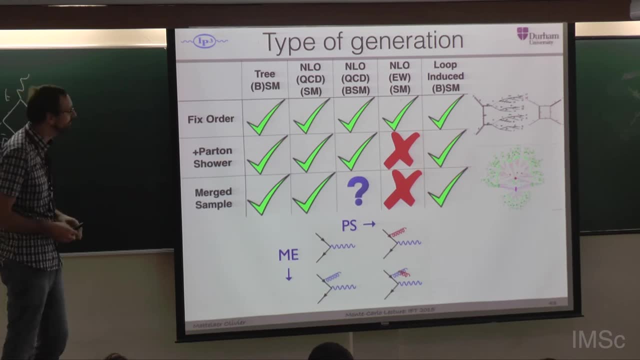 But then you also want to have the source jets described correctly, and for that you need the pattern shower. So what we are going to do is going to merge the sample with some magic- that will be explained by Leif- And in Margraph you're going to generate ttbar sample. 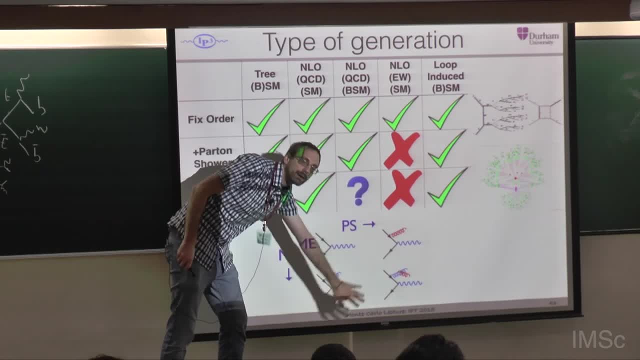 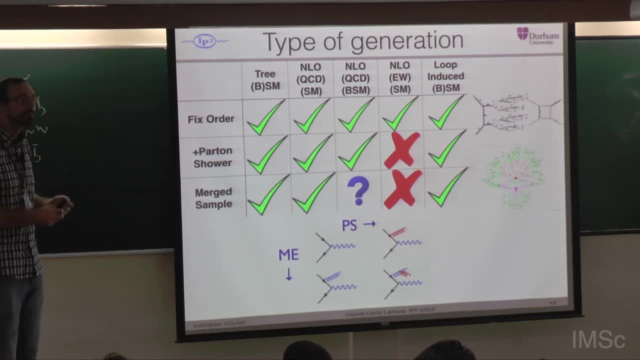 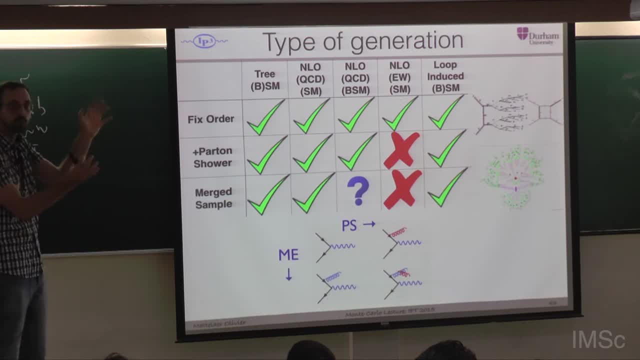 ttbar plus three. Another example: with ttbar plus one jet, ttbar plus two jets. then you run the pattern show of all those samples. you have a lot of double counting and that's where you need to apply a lot of magic in order to remove those double counting and combine all those. 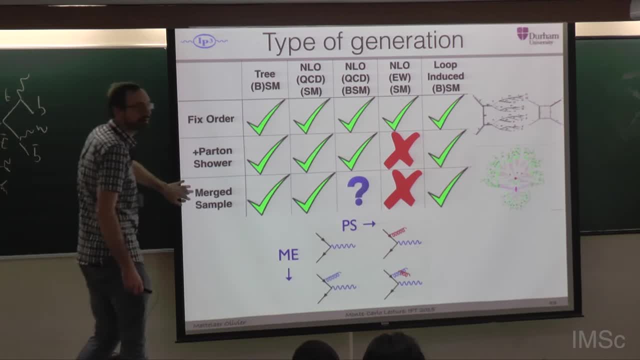 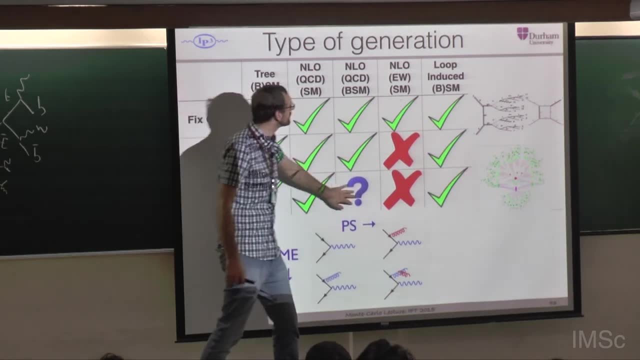 samples together in a coherent way, And that's what we call merging. And then we can do it at three level. we can do it at NLO and of course for BSM it's always complicated, so that's why I put a point mark and we cannot do it, of course. 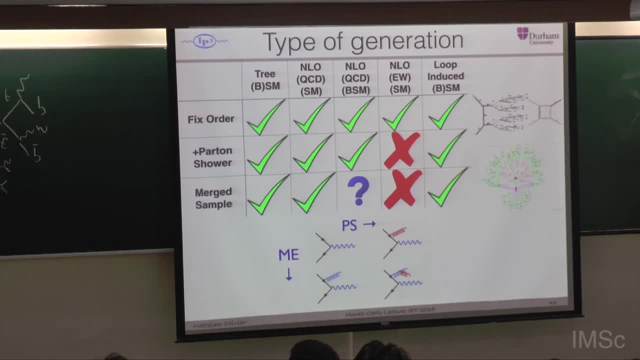 in ElectroEak, Basically the status of all the type of computations that we can do in MadGraph so far, which is already quite large, and of course we're going back doing those lectures more in details. It's very short descriptions of all those steps. 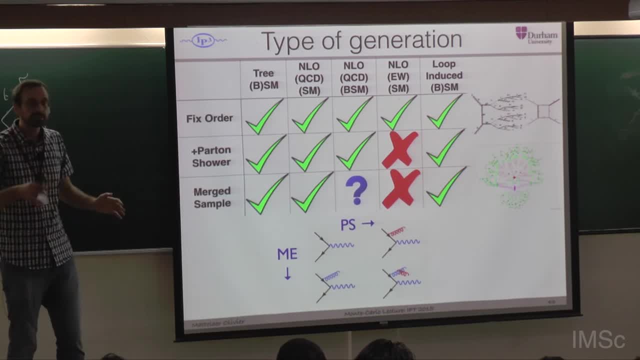 But what is part-on-shower, what is merging? that will be explained in more details tomorrow. What does Christian mean? Hm, What does Christian mean? Well, because if I put a yes, people complain. If I put a no, people complain. so I put a question. 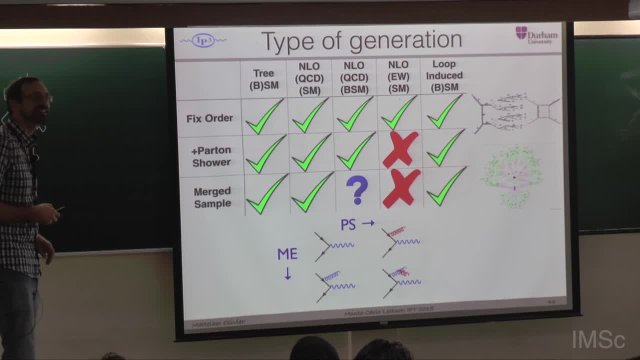 mark. If I don't want to enter in actually long discussions, let's say it's an open debate. That's why I put a question mark. In a lot of cases you can do it. There are a lot of cases where you cannot do it and 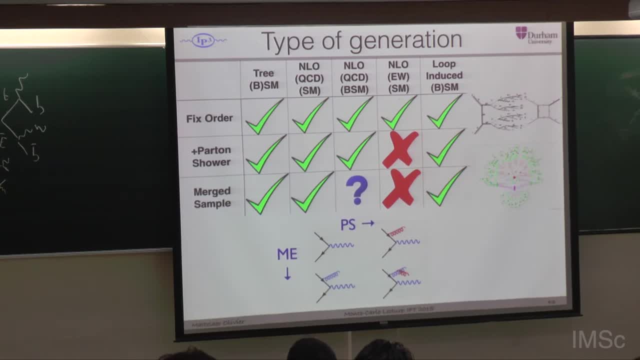 therefore, it's really in the between. Does this also take care of the final state radius? Yes, yes, yes, yes, Yeah. in this example it's on initial state. You can also do for final state. OK, so good amount of time. 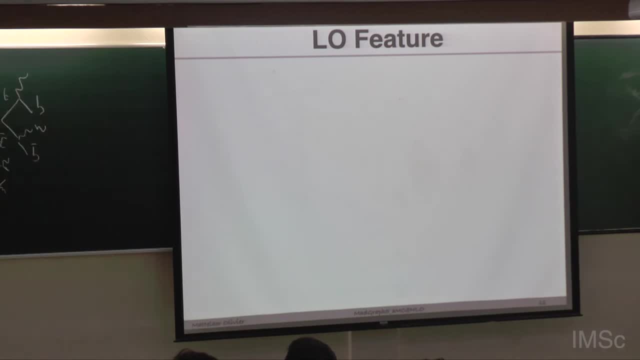 So I want quickly to show up a couple of leading other features that you will learn basically during the tutorial. I'm not going into details, But we have in MathGraph methods to compute the whiff. Whiff are extremely important for physics obviously. 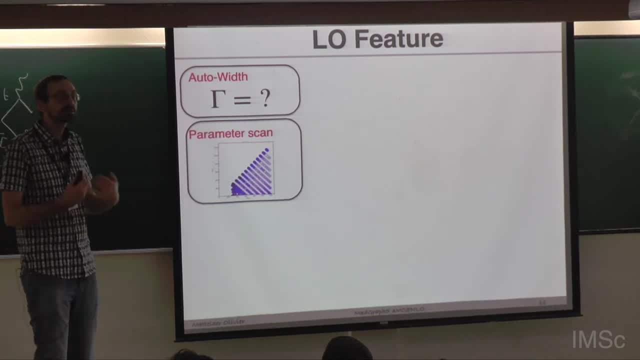 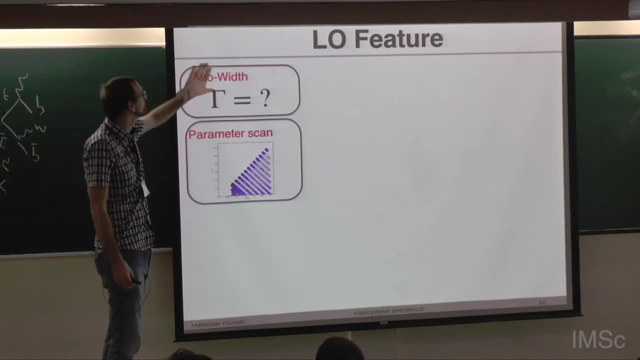 The fact: what are the whiff of those particles? Those are not taking any other computations. That's a full other effect. but it's of course important to include them And in MathGraph we have an auto-whiff and we'll probably 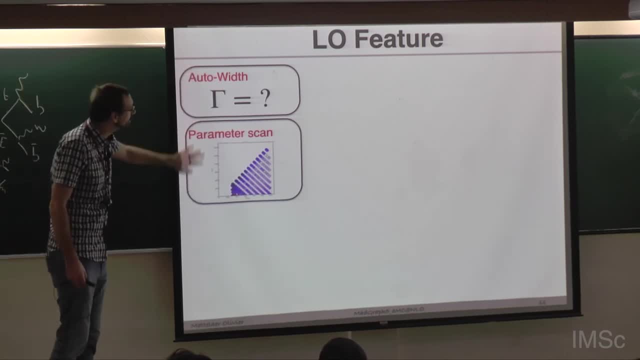 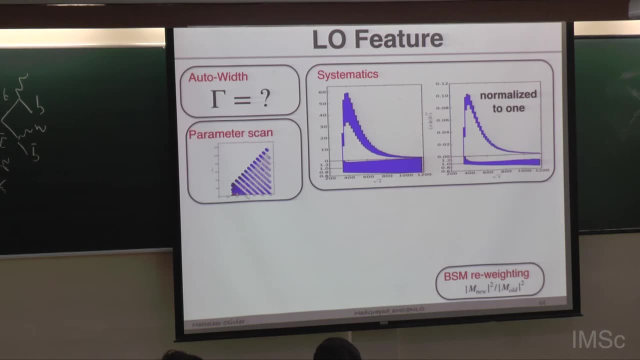 cover that a bit during the tutorial. We also- that I'm sure that we're going to cover in the tutorial- How to do a parameter scan. We have a model for that. What is quite important- and I like this plot a lot- 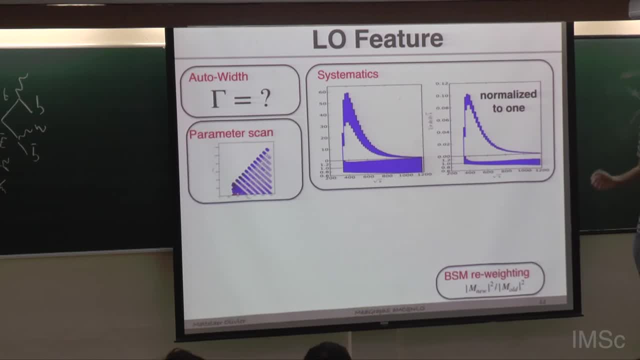 is systematics and reweighting. So we have a couple of reweighting features in MathGraph and this one is the most important. So I told you before you have a huge scale uncertainty at cleaning order, And that's actually what I mean by that. 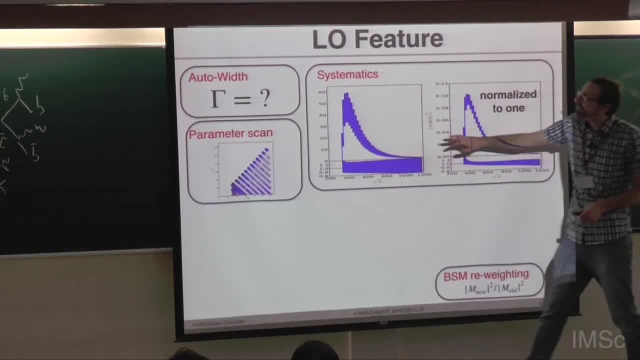 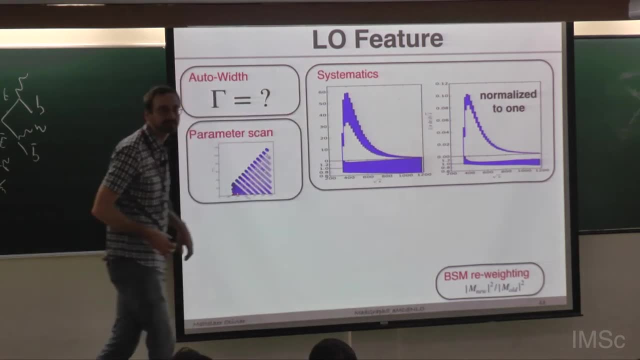 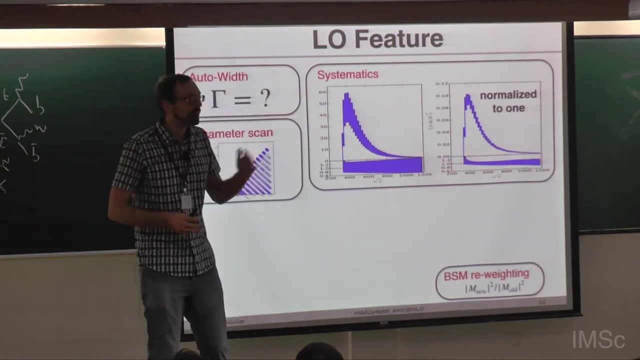 So this is TT Bar Productions and this is the. what is it? The square root of s? okay, So that's the invariant mass of the TT Bar system And those error bars represent what is the difference if I change mu f and mu r by a factor of two? 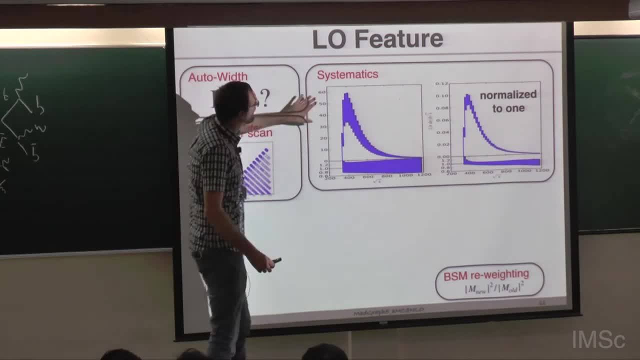 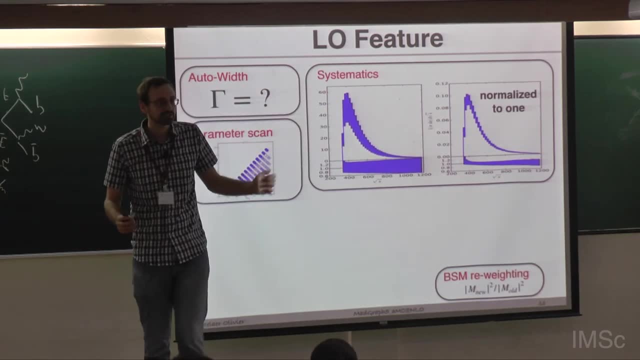 So if I multiply those by two or divide by two, my predictions fluctuate in that range, which is around 40%. So it's a huge fluctuation in that case. Now, what is interesting if I'm doing now removing? I don't know. 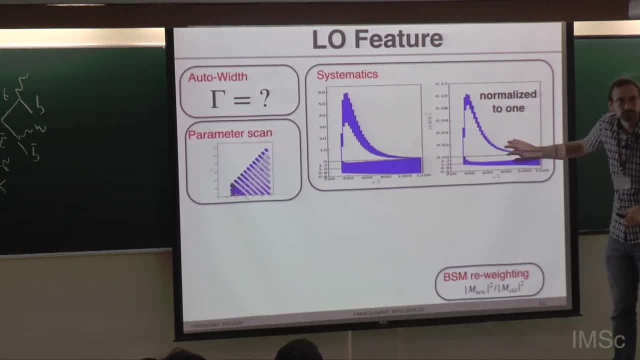 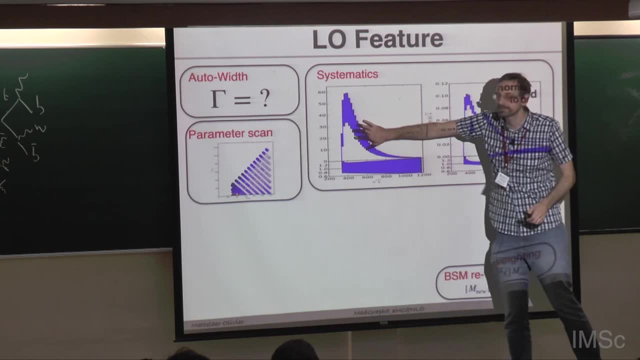 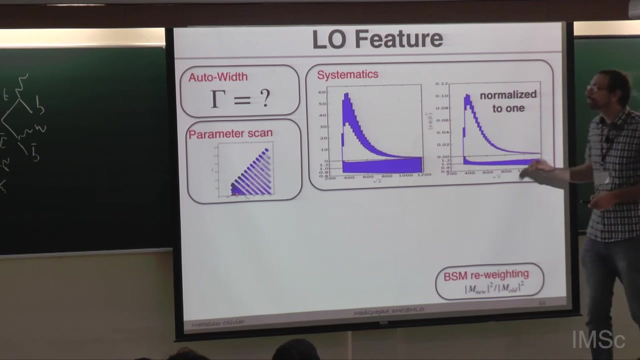 but the normalizations, you see that it shrinks quite a lot. So that's why I say that cleaning order. the shape is well described, but the total normalization which is included here is not well described. In order to do those plots in principle, I would need to do nine. 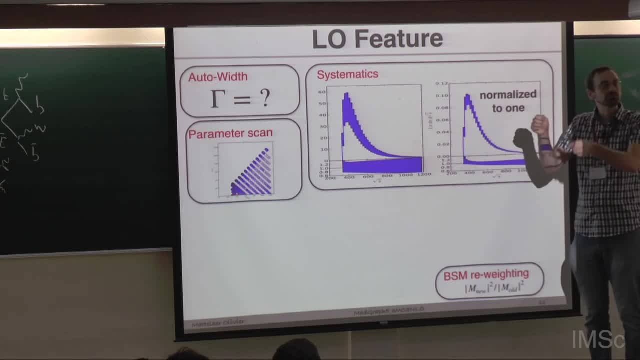 computations of MathGraph, one or two other, and each time change those factor mu f and mu r, by a factor of two up or down, And that would be slow. If I need to do the same for PDF, I need to do one of the different computations. 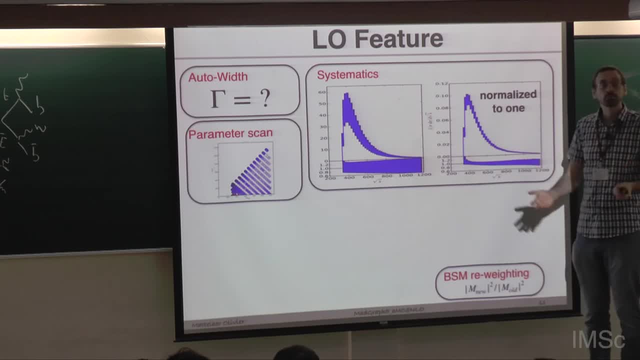 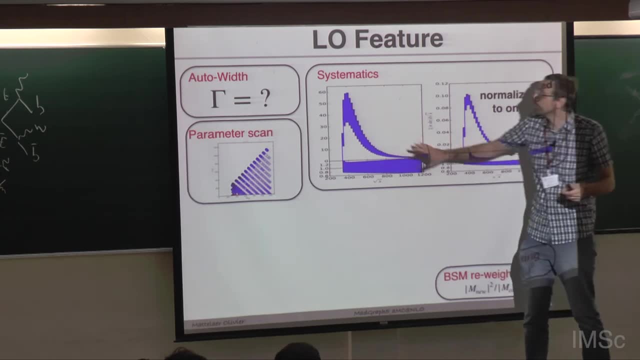 Okay, So we have a method which is called re-weighting: Instead of doing 100 different computations, I'm actually tracking MathGraph in advance, all those factor centers, and then I'm just re-evaluating a polynomial in order to fluctuate those points here. 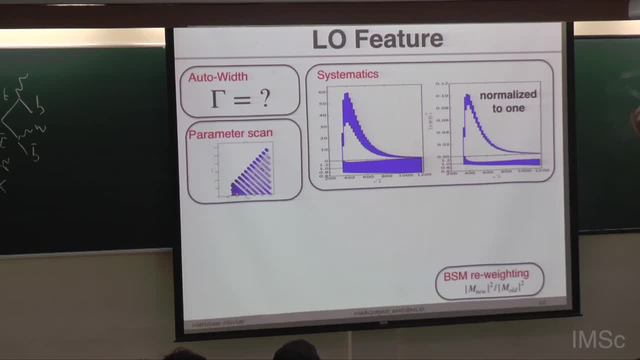 So that's what we call re-weighting, and that is extremely fast. To do those 100 computations, it takes me around 20% more time than doing one computation, So it's actually quite efficient. Interference terms are also included. 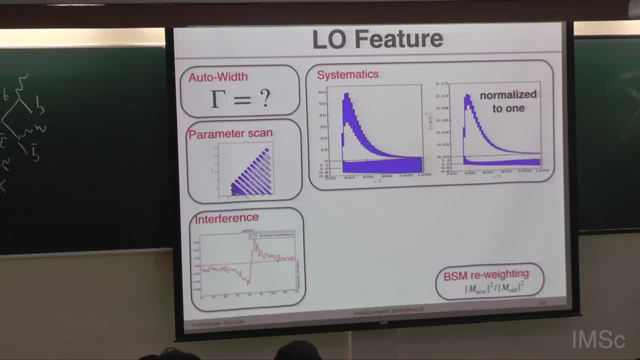 As I said before, this z-photon interference 2-2-2,. that's simple enough. MathGraph can handle that for the phase-space integrations. If you try to do interference for 2-2-6, the phase-space integrator will. 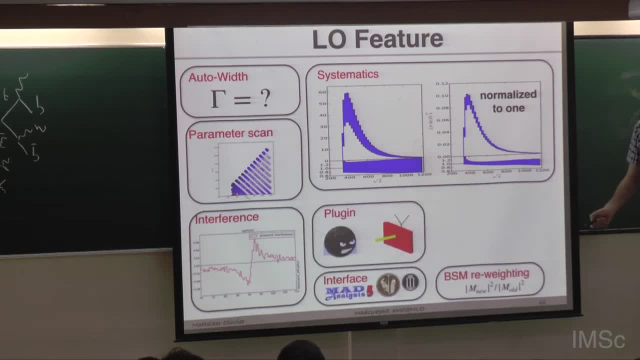 break down most of the time. We also have a plug-in, so that's a way to customize completely the code, like MathDM- that was slightly described, probably on Friday, and here MathDump, which is another plug-in. We changed the physics. 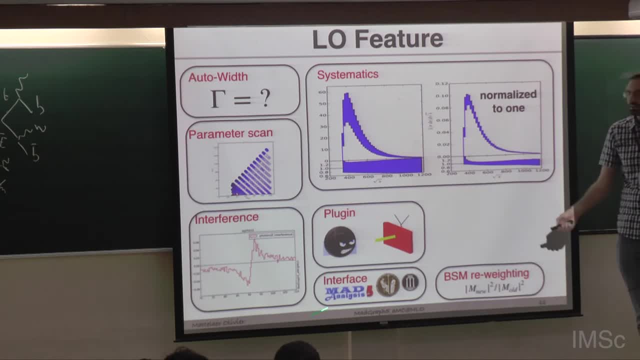 We can approach this MathGraph. We have interface, so you will see that in the afternoon, Not only to run MathGraph but to run the full chains from MathGraph. So we can say, run also PTI8 with those parameters. 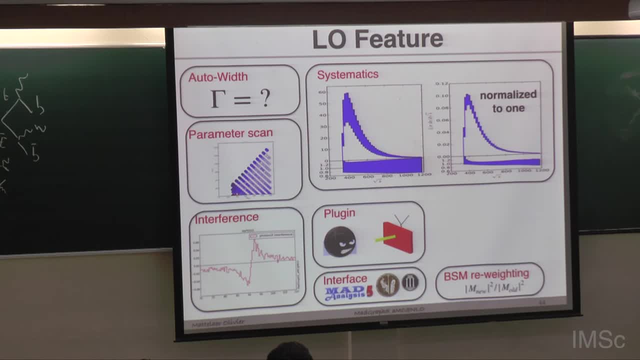 Run also MathLGS5 to do the plot, or run DELs to do the simulation, and so on and so on. So that's all what I call interface. That code's not developed by us. We don't want to take any credit here. so you still, when you use them, give the proper. 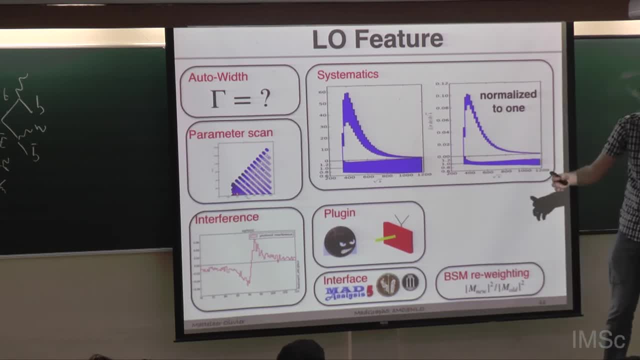 credit to the author, obviously, But that's code, That's code that you can run from us so that you don't have to manually move the files and stuff like that. And finally, and I still have a couple of minutes, good. 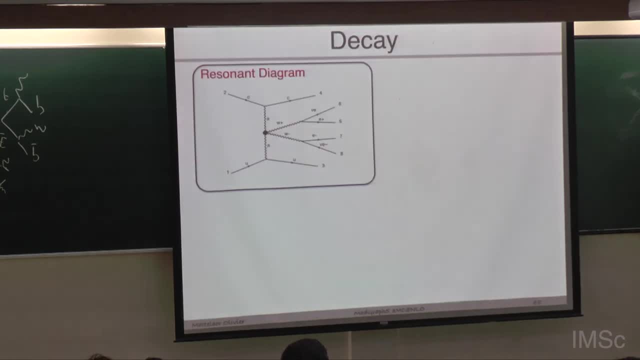 Now with approximations. I'm going to describe a bit now. Okay, So now with approximations. this is a VBF process and I have my two W decaying into leptons, So this W leptons neutrino and this W leptons neutrino. 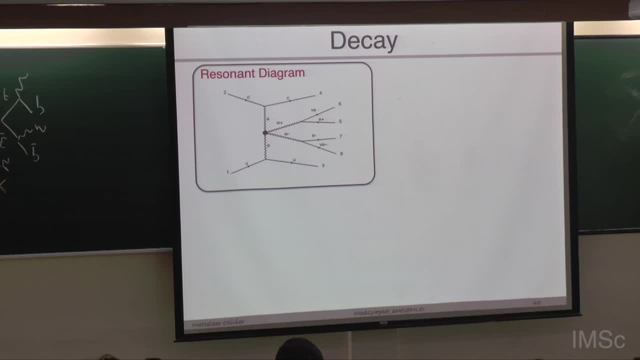 So I have a two to six final state, But I'm really interested actually to two W decaying. But if I want to do the full computations, what I actually have, I have a bunch of diagrams like this, which I call non-resonant diagrams. 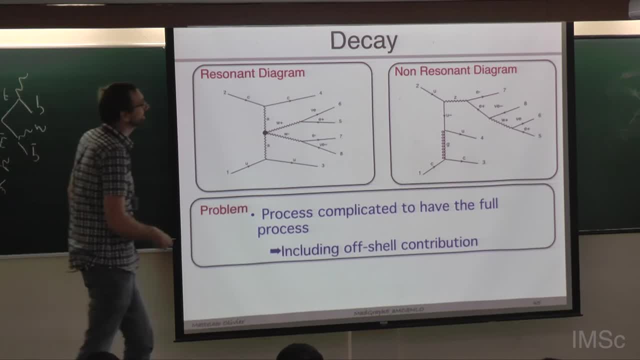 I don't have my two W, which decays afterwards. In this case I only have one. So that's not really what I want. but if I want to do the real computations, I need technically to integrate all of them, And that's, of course, will slow down the computations, as you can expect. 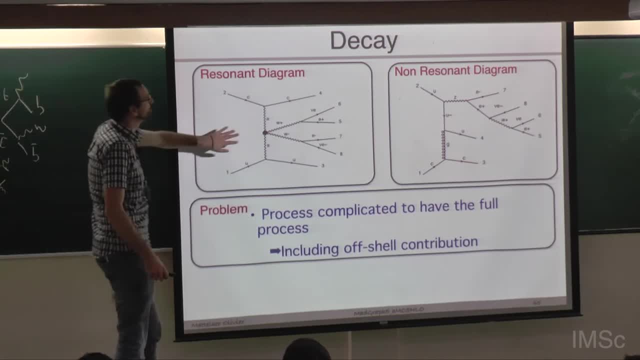 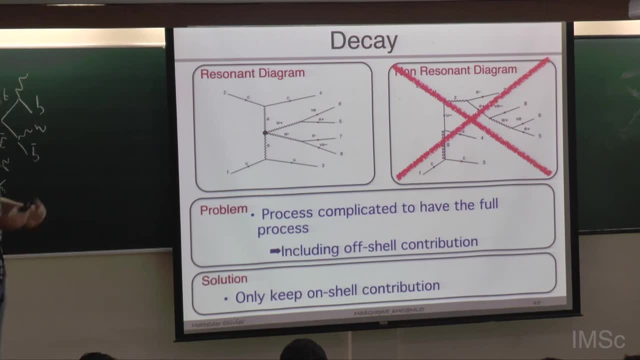 But in practice these diagrams, when those two, those W are on-shell, completely dominates about everything else, And that's because of the whiff. So a practical method is to say I'm only interested in the on-shell contribution. So when those particular on-shell, because that's where those diagrams are going to dominate. 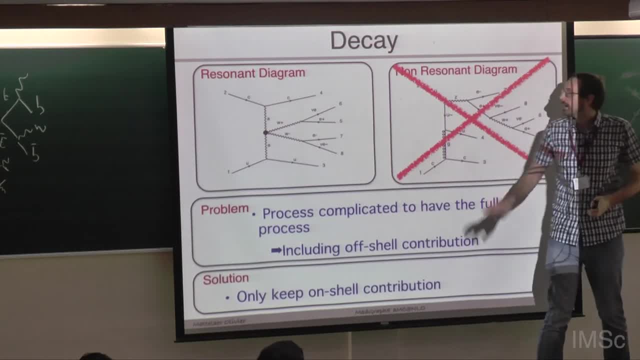 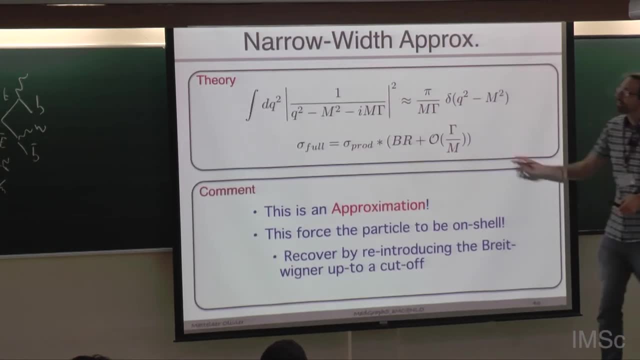 compared to all the other diagrams And therefore you can say: I'm going to neglect that. So this is based on now, with approximations. So if you go back to these integrals, which is the that we saw before, you can resolve this. 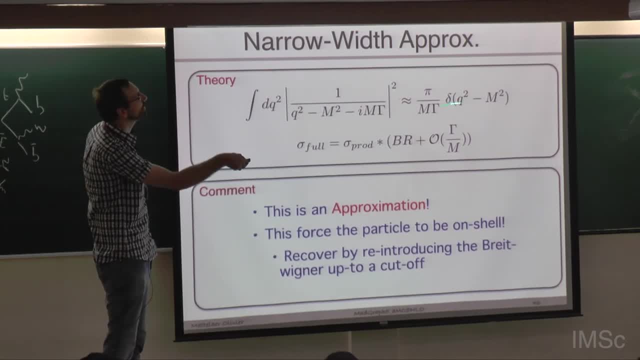 And if the whiff is small enough, you can resolve this by a delta function times a prefactor which is one over the whiff, And therefore saying, in other words, the full cross-sections is the productions times the branching ratio. 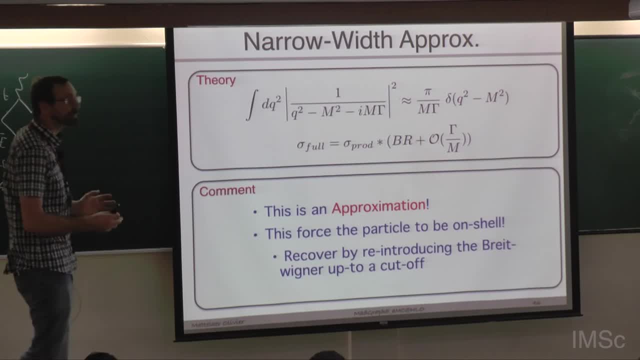 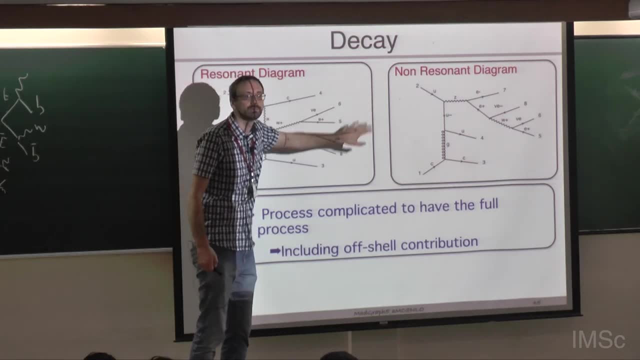 This, of course, is correct only now with approximations in the whiff is small, also because otherwise those diagrams here are not negligible. So I've seen a lot of people using the fact that they can only keep those diagrams even. 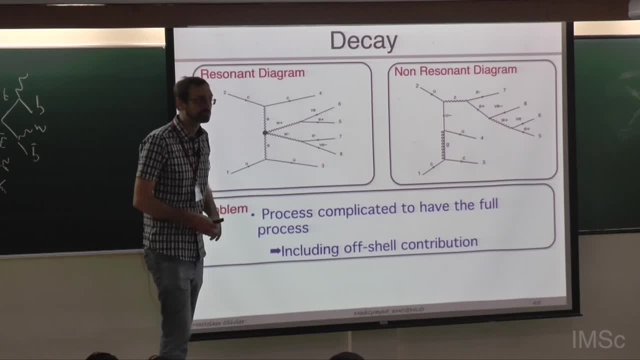 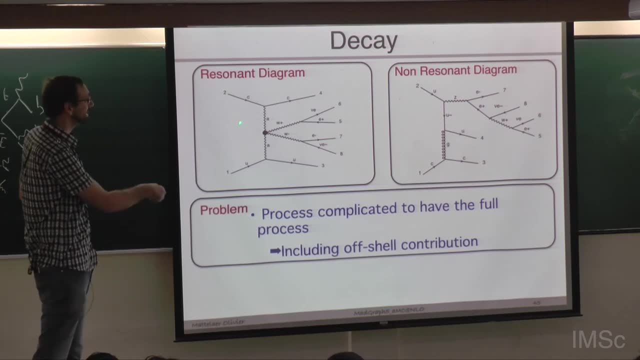 when the whiff of those particles, in that case BSM particles, are 20% times the mass, or even 100 times, or sometimes the mass, when the whiff is as big as the mass. Of course, in that case you cannot neglect the interference term. 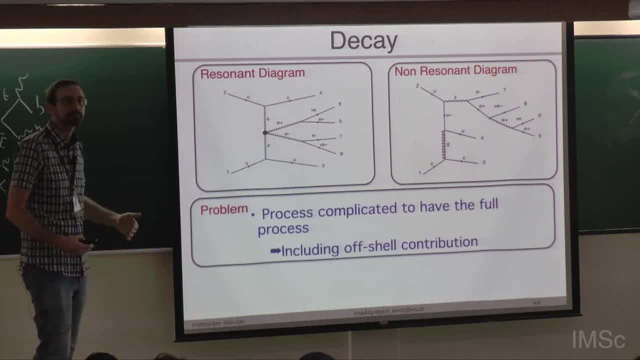 There's no enhancements to the Brieg-Wigner and that's a bad idea. So my message here- and that's really why I wanted to show this- is my graph is, of course, doing hypotheses when it's going to computations, hypotheses like the maximum. 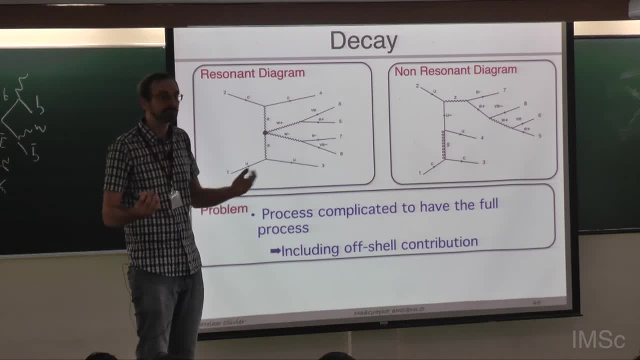 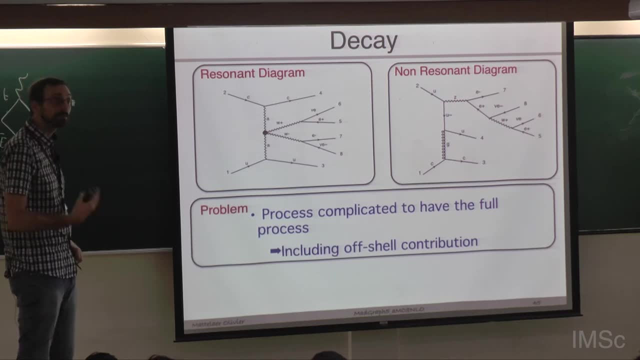 exists, You have to put cuts, otherwise my graph cannot integrate infinite numbers. obviously, But also like: oh, if you only select those diagrams, you actually have a hypothesis that my graph will not check for you is that you are now for approximations. 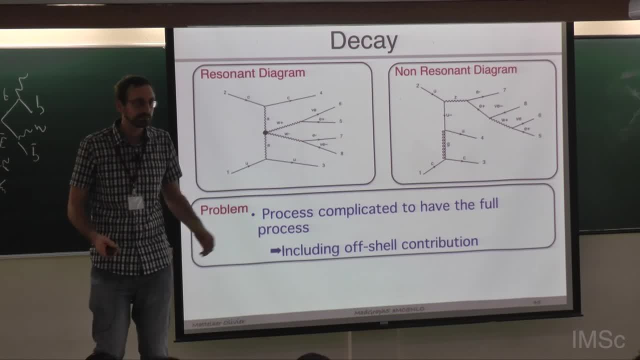 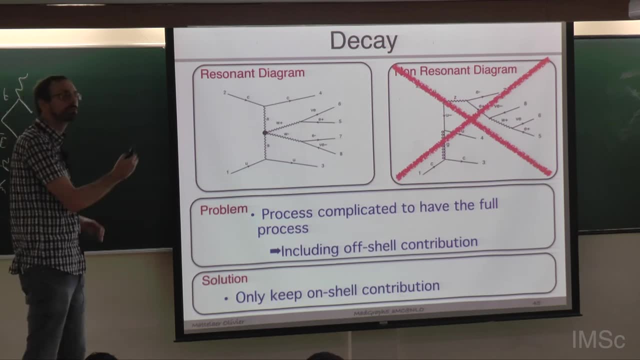 The whiff of those particles need to be much smaller than the mass, and that's something that you need to check when you're doing the computations, otherwise my graph will go probably in the world. So you can't return bullshit result, or clearly at least not physical result. because what? 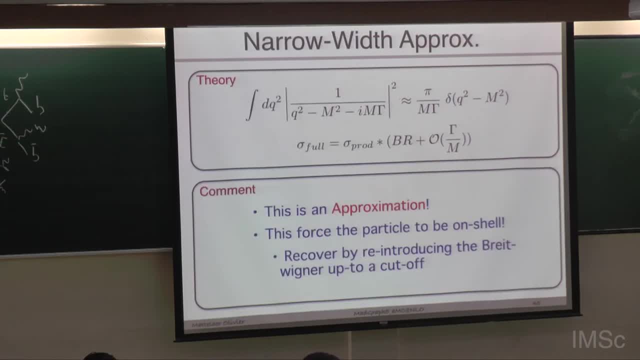 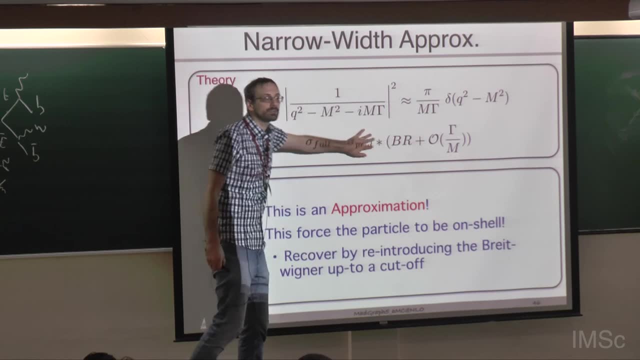 you ask, is unphysical. Yes, of course. also a comment I have. often this formula is in approximations, obviously, and therefore my graph will not use most of the time this formula itself. It's going to do the full phase-based integrations up to cuts, and those cuts are really important. 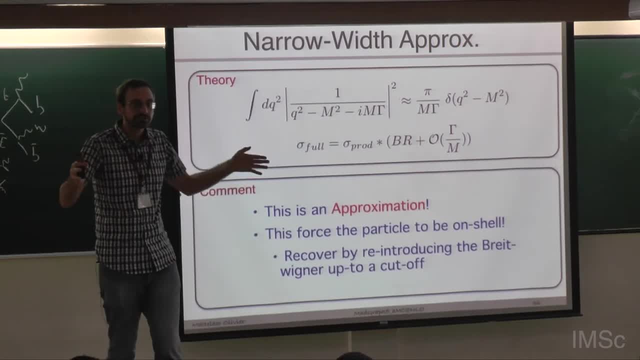 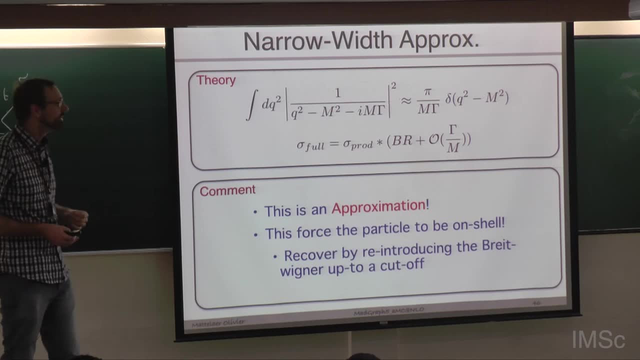 So, as I say, we recover by introducing Brieg-Wigner cuts, So we do the full phase-based integrations up to cuts. If you remove those cuts- that's something I see a lot of people doing quite often- you actually allow to be extremified in the tail, where again those interference terms are important. 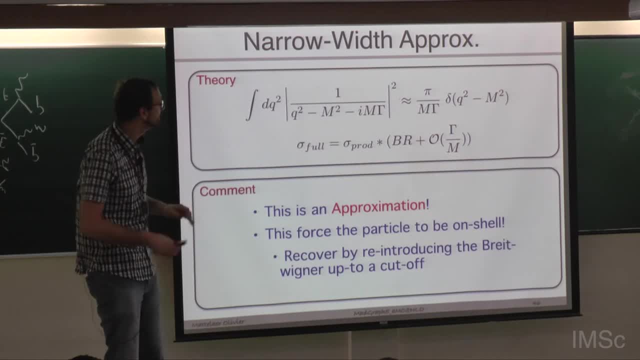 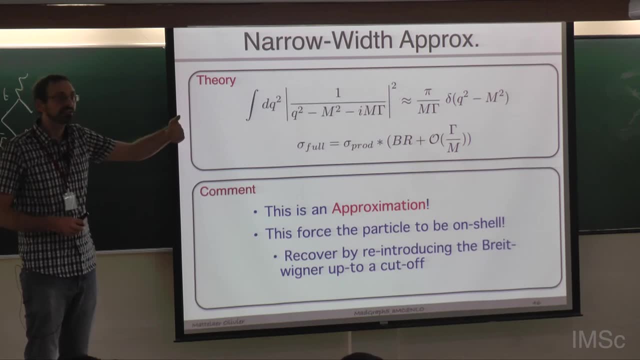 and they are extremely important- to recover gauge invariance. So if you don't put those cuts, then you're allowed to go to regime where you miss those interference terms that restore gauge invariance and therefore you can have unphysical growth of your cross-section and stuff like that. 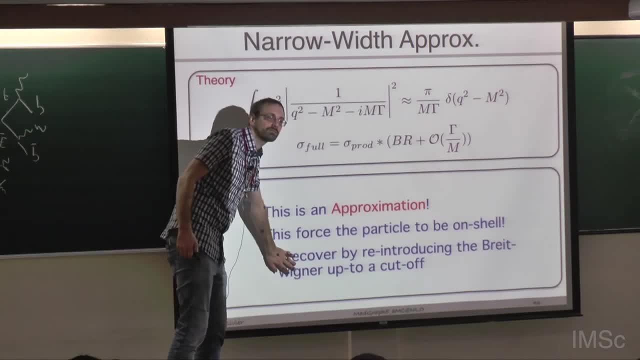 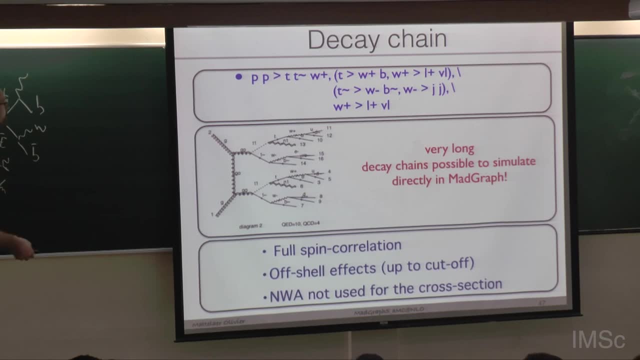 So that's again. Those cuts are really important to preserve gauge invariance and I see a lot of people who try to bypass those cuts. Okay, thanks to that, we can do process like 2 to 16 in this case. 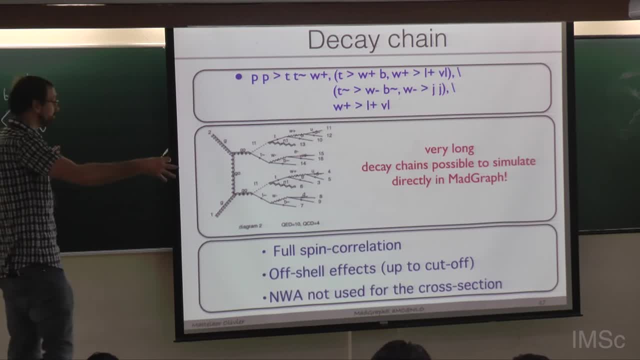 I even see once 2 to 18, so extremely long- phase-based integrations. but this has a lot of particle on-shell, with decay to on-shell particle and so on and so on. That's one of the most number of final states we can ever do. in my graph is something like: 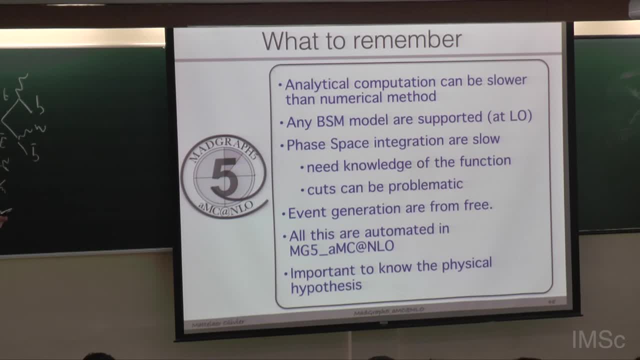 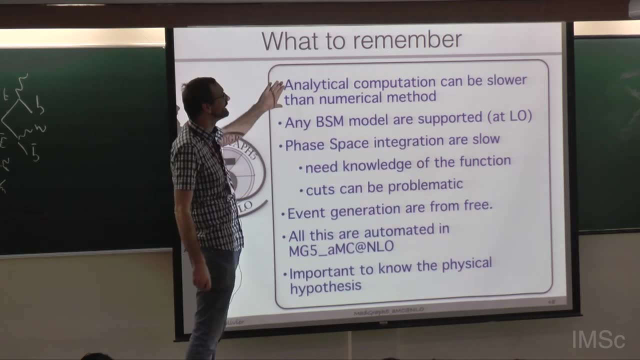 this, Okay, So that brings me to the End of my talk. What I want you to remember for today is, first: analytical computations is slower than numerical methods, and that's quite important for me, because a lot of people came with me, oh. 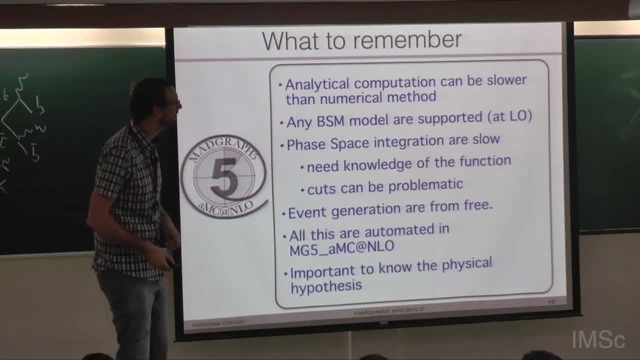 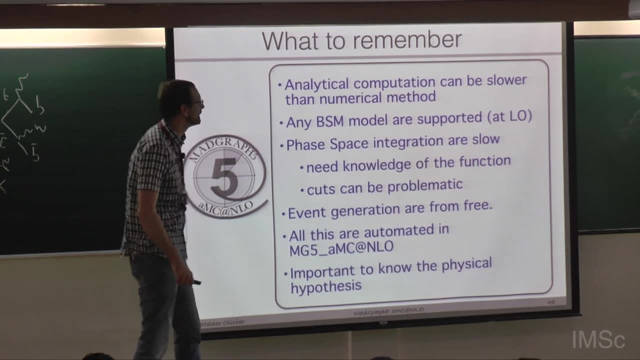 I know how to compute that matrix analytically. will it be faster? And the answer is typically no. Also because I need not only the full computations but the amplitude individually. actually, We can do any BSM model at leading order, but actually now more and more at leading. 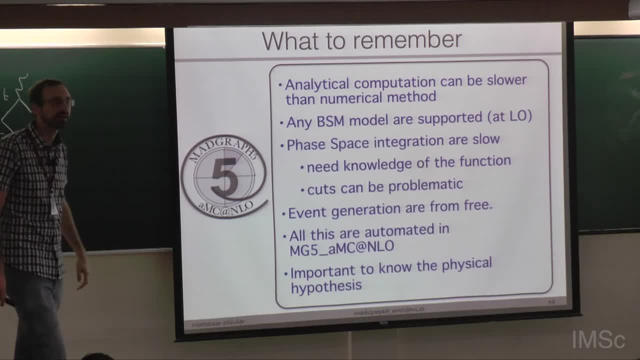 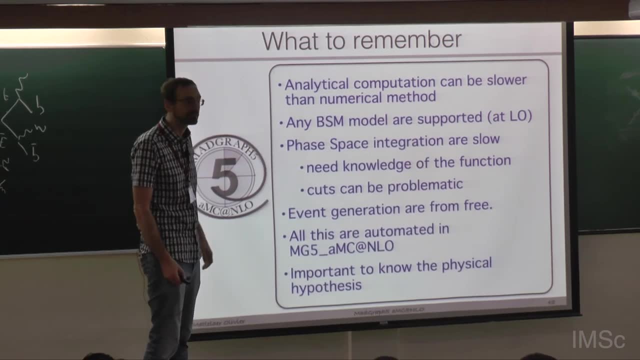 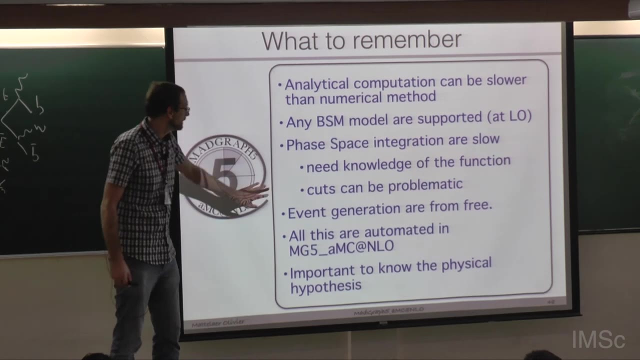 order as well. So we have the full chains actually now to do NLO as well automatically. The phase-based integration is slow. We are using Monte Carlo method, which is slow, And therefore we need to know the other functions. therefore, be careful with cuts. 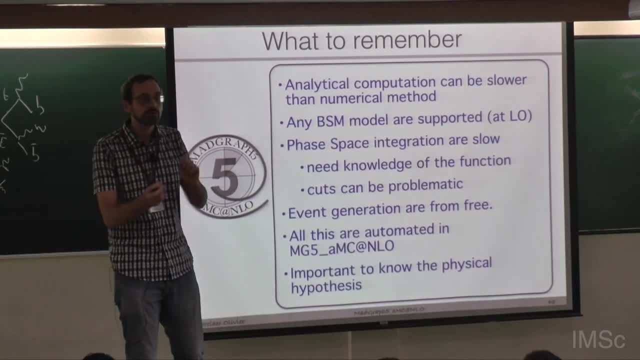 Event generation. I can for free. We use Monte Carlo, so we have no correlation between our events, so we can just use those ones. We just need to select them to shape like the detector. but that's very simple to do, Okay. 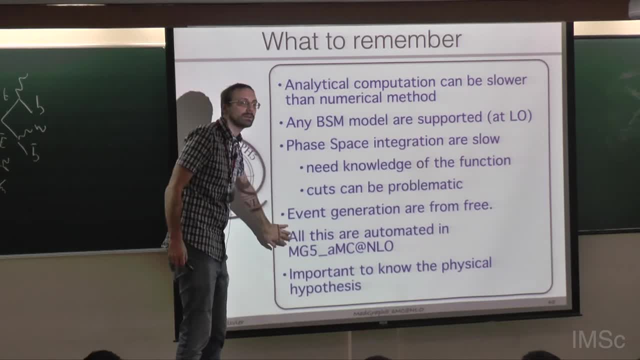 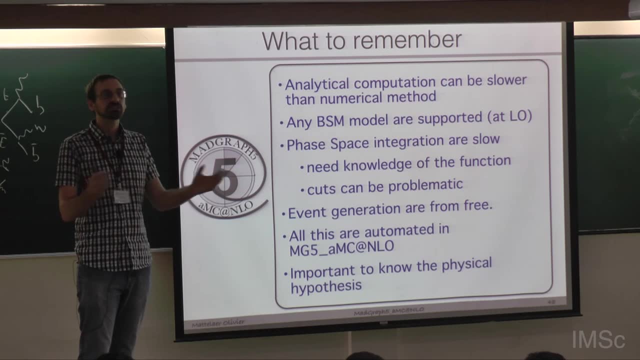 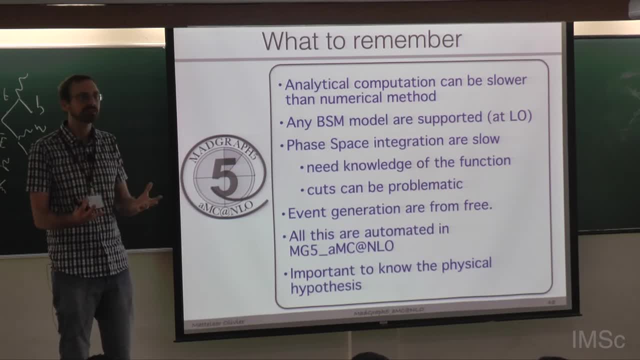 Come back to us if you have any questions, if you don't understand something. That's really an opportunity for you to learn and to communicate with us, obviously, And for us to learn what you don't understand, what is not good in our code.